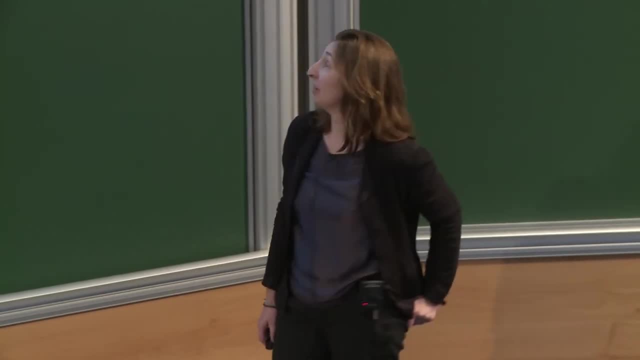 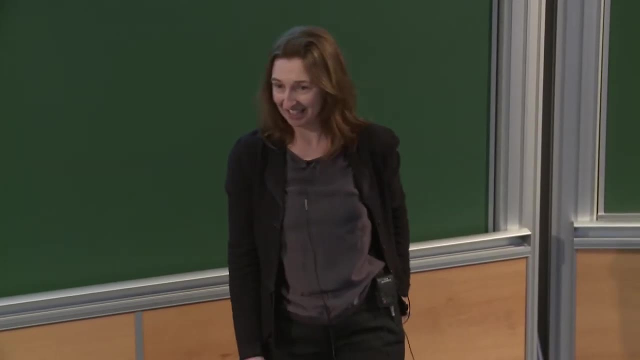 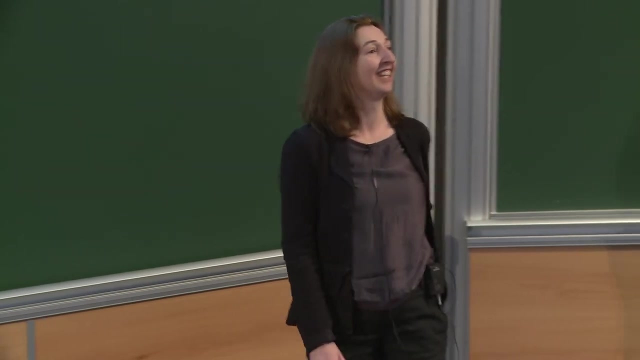 for nearly 20 years now in Trinity. So in that time we've had many interesting physics discussions, I think. but we've also fought many battles together with our university administration, or against our university administration, I should say. So in that sense we have worked. 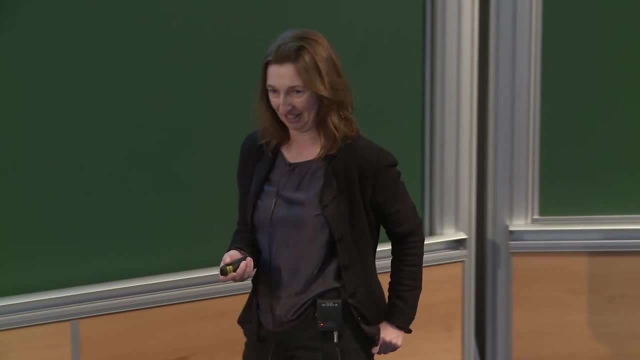 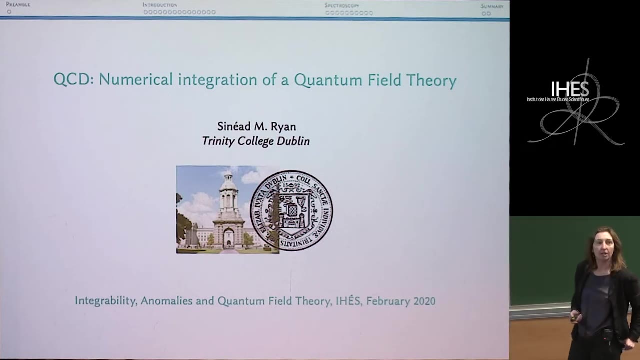 very closely together, even if not as collaborators in physics topics. So I work in lattice QCD. so a little bit tangential, I suppose, to the main topic and thrust of this workshop, although of course still within the theme of a quantum field theory. 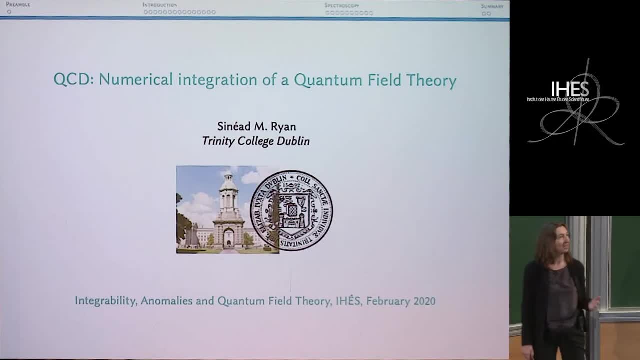 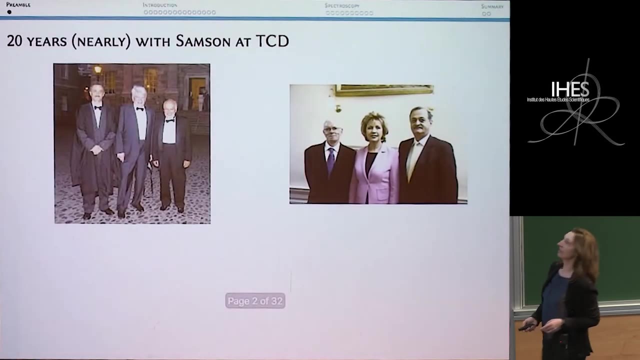 and somehow still, if you stretch it a little bit, within the theme of integrability, although here we're talking about numerical integration, so it's a little bit different, I grant you. Okay, so let's see if I can get this to work. Okay, so, just to start, I found some pictures, 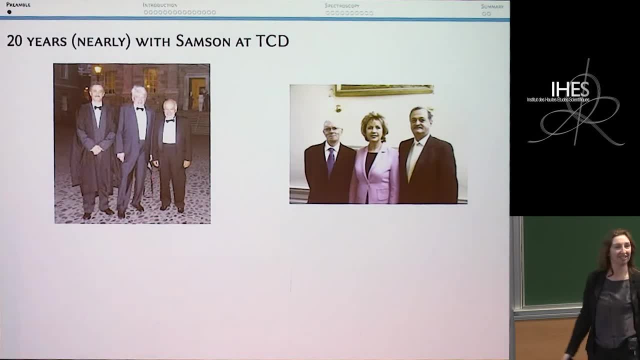 from Samson's nearly 20 years in Trinity. So Leon already showed this one this morning. so this is Samson in his academic robes in Front Square with people that of course you recognize, but this one you won't maybe recognize the people. this is Samson on the. 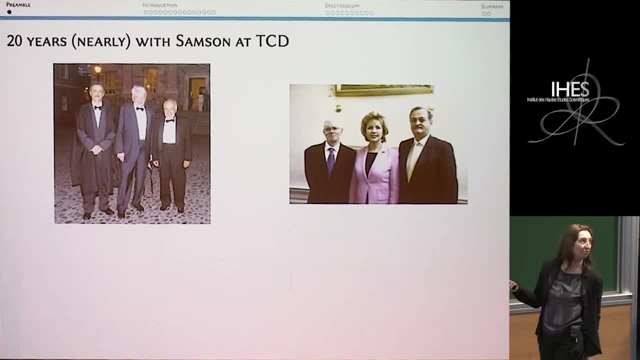 occasion of the award of his gold medal from the Royal Irish Academy for his contributions to science. This woman in the middle here is Mary McAleese, who's a president of Ireland and awarded the medal at the time, and I have to confess I have no idea who that person is, so I apologize. 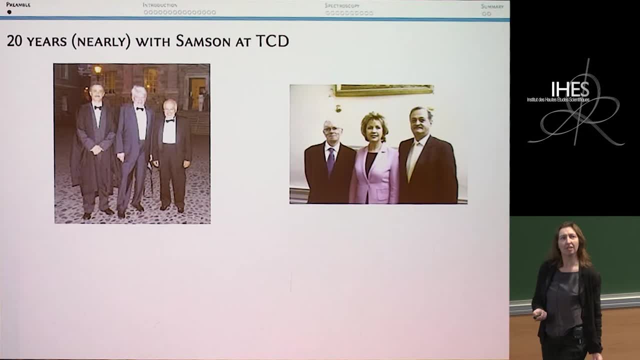 Maybe, maybe One in mathematics and one in humanities. So this is okay. So Nana knows far better than I do already. So these are some highlights, of course, from Samson's time in Trinity, but I should also point out that Samson lives on campus, as many of you know. 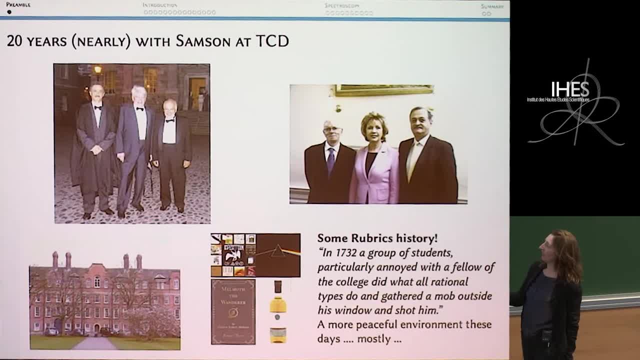 he's very warm and hospitable and I've had the occasion. his apartment is on this side over here somewhere- so I've been invited many times by Samson and Masha to spend an evening with them, and then we've listened to good music, we've discussed somewhat esoteric literature. 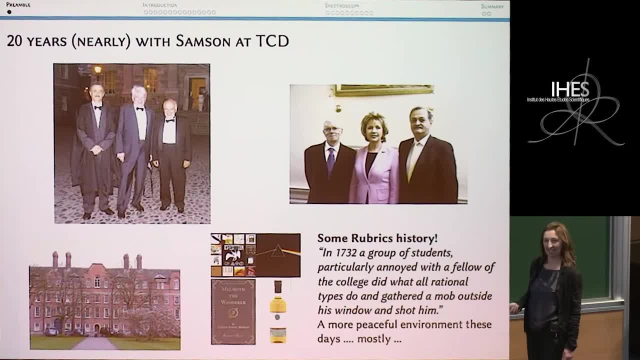 lubricated, always by some very nice beverages, But I also found this when I so. this building is the oldest surviving building on the Trinity main campus. It's called the Rubrics, where Samson lives, and so there's some history which I discovered. 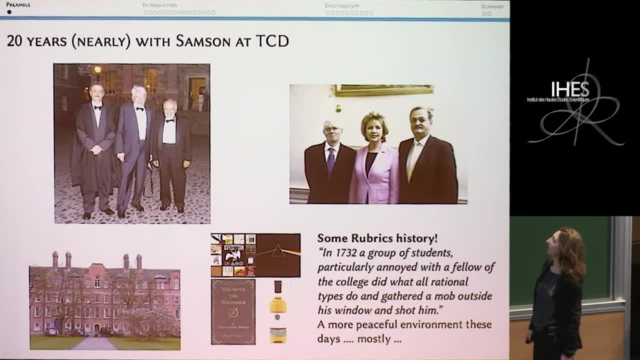 which I don't know whether you already knew this, Samson, or not, but in 1932, a group of students who became particularly annoyed with a fellow, of which Samson, of course, also is of Trinity, apparently did what all rational types do. so this is from a history of the time: gathered a mob. 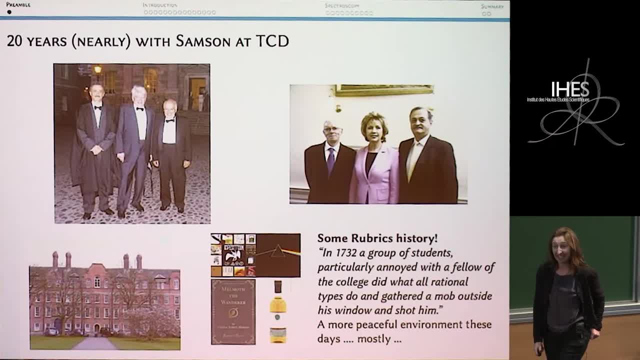 outside his window and shot him. So apparently, nobody was arrested and held responsible for this particular murder, because they were all in costume and they weren't identifiable. however, the group of students was expelled. I think that's right. yes, yes, so it's much more peaceful these days, at least normally. 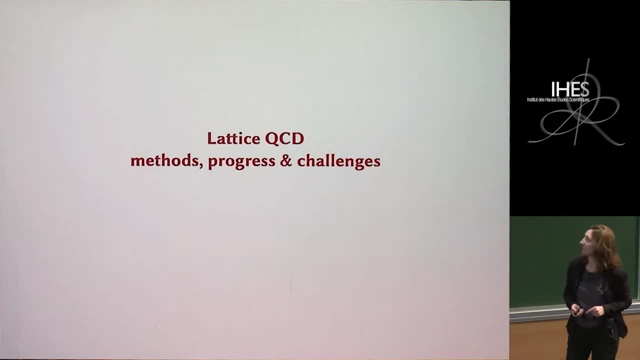 Okay, so I, as I said already, as advertiser I was talk on lattice QCD. I will tell you a little bit about the methods that we use to evaluate observables in this quantum field theory and try to give you a sense of some of the progress that's being made and the challenges that remain in the topic. 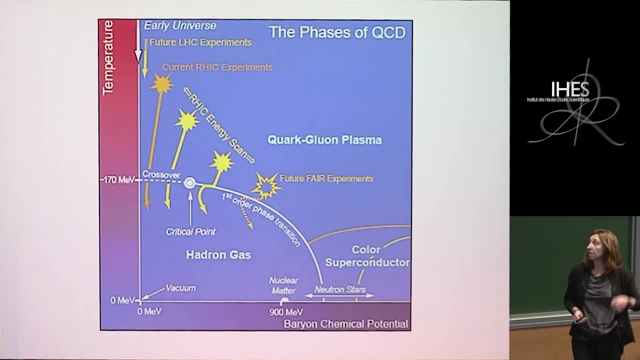 Okay, so this is a cartoon of the phase diagram. so to understand fully QCD, one should of course any theory, one should try to map out the phase diagram. and so this is the phase diagram in the chemical potential, the baryon chemical potential and the temperature. 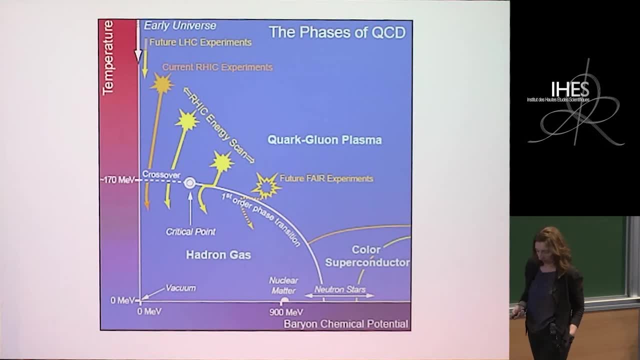 and what we know is in fact quite limited, or at least what we know from first principles is quite limited. it's certainly limited, as I'll discuss in a little bit more detail soon. it's limited in particular to this temperature axis here. 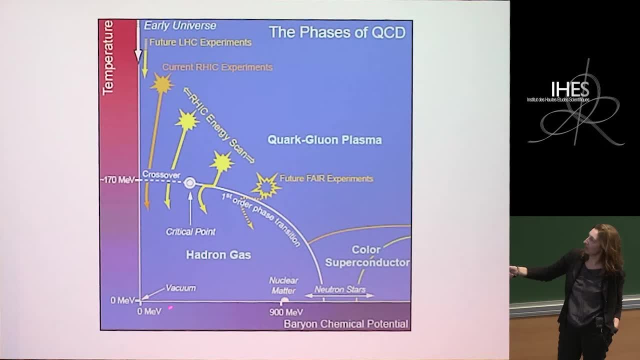 so we understand quite well how to formulate the theory and how, in a discrete and numerical simulation, to to calculate observables and to properties of the theory at zero chemical potential. so as you go out in chemical potential, as I'll allude in a little while, you'll see that this becomes an extremely difficult problem. 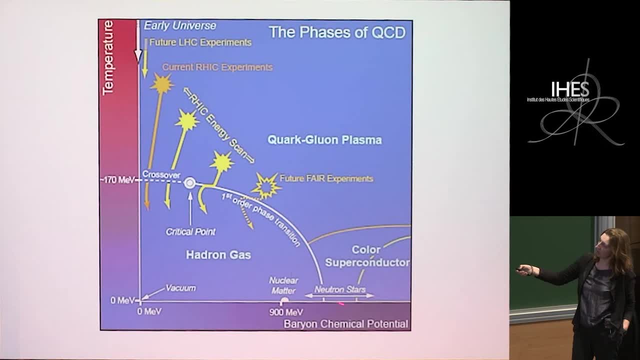 in fact, it's an unsolved problem to understand how to make calculations at finite chemical potential. In Bruggemann National Lab, we're building an electron ion collider. is there any place? Yes, Yes, so the EIC. so this is Rick. 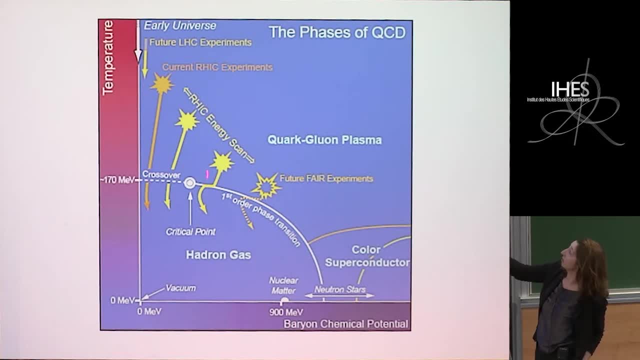 this is Rick is up here doing an energy scan and EIC will certainly be probing higher energies and higher temperatures. so there's a lot of interest from the lattice community for EIC physics for sure, absolutely So. one thing that so in lattice calculations, as I said. 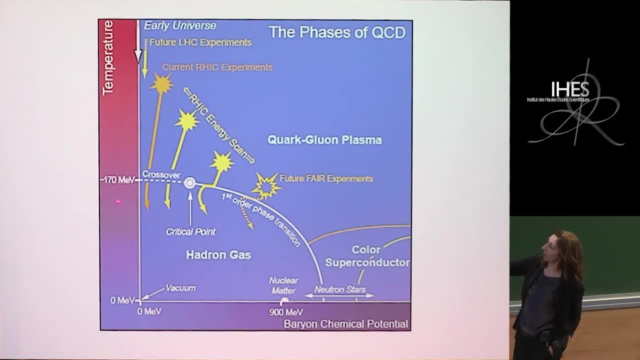 you can formulate the theory in a thermal field theory background and you can make calculations at finite temperature. in fact, that's done, although it comes with particular challenges in its own right. and you can, if you're brave, you can try to venture out a little bit. 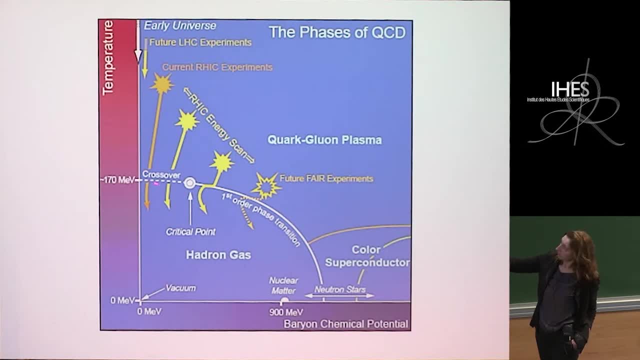 into this non-zero chemical potential plane, and those people who have done this have been able to at least make some baby steps in this direction- and you see those lines dotted there and then establish that the transition here is a crossover, for example. so this was a contribution from lattice calculations. 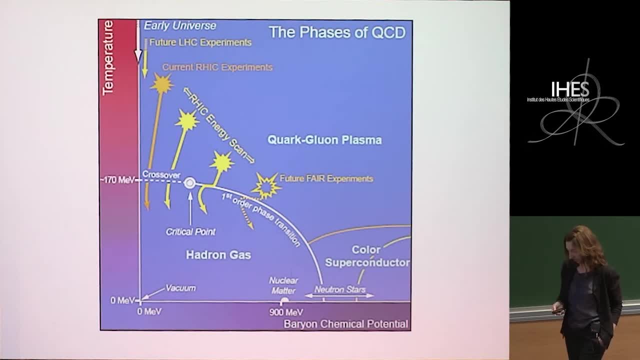 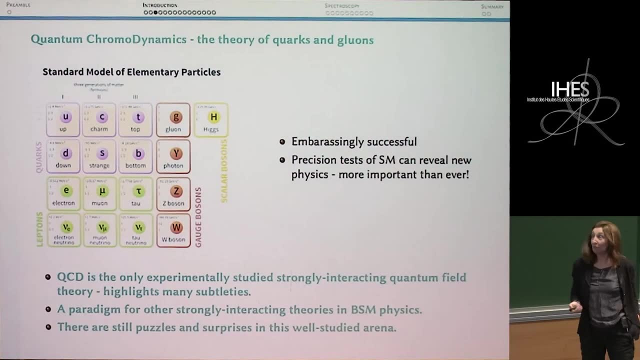 but you see that there's a rather a large amount of the phase diagram that remains, at least for the moment, inaccessible to us. Okay, so what can we do? So the QCD, of course, is a quantum field theory within fundamental variables. 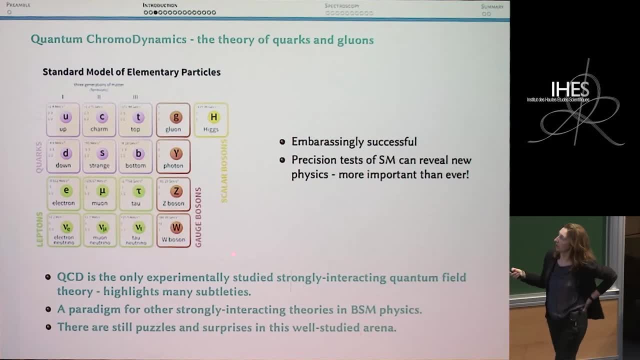 which are the quarks and gluons, and is a building block of the standard model, which whose parameters you can see gathered here. So just a few short words on the standard model. I won't say very much about this, except, of course, to remind you that this is embarrassingly successful. 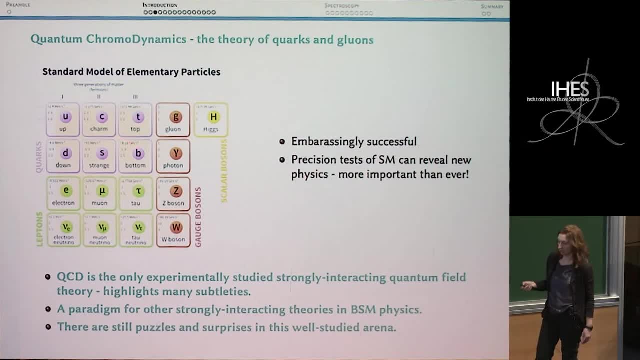 and despite huge efforts, certainly from the experimental community, this in some sense is not broken yet and in fact this motivates QCD people even more, because the precision tests, so new physics, has not been immediately or directly accessed yet in experiments. 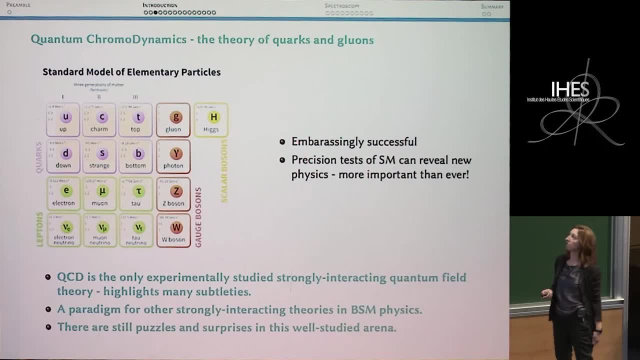 and so looking for signs of new physics indirectly through precision tests of standard model variables is more important than ever, and in fact QCD plays a role in those precision tests. It also remains the only experimentally stable, studied strongly interaction quantum field theory. so one gets to learn quite a lot about. 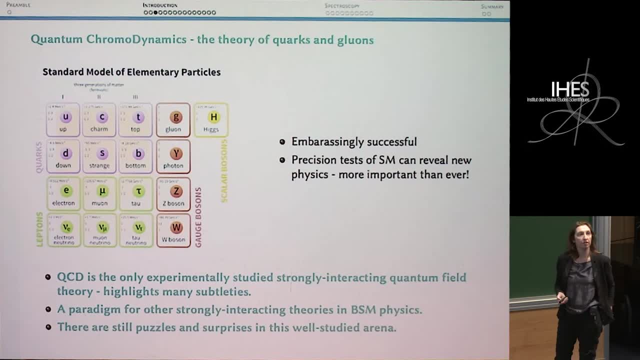 such strongly acting theories in a regime where, at least in principle, there are some benchmarks and experimental tests that one can check your results against. So it provides us with a paradigm for strongly interacting theories, for example in beyond standard model physics. And I should also say it's important to note that this is not in some sense a solved problem. 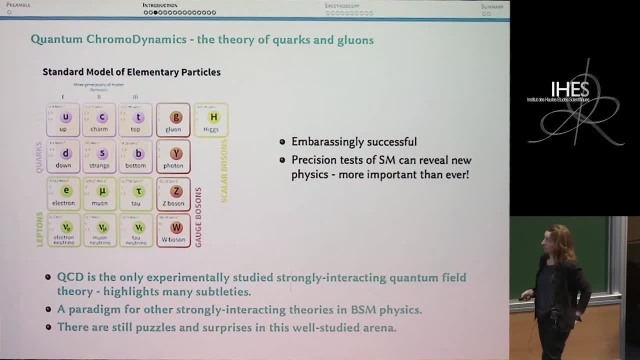 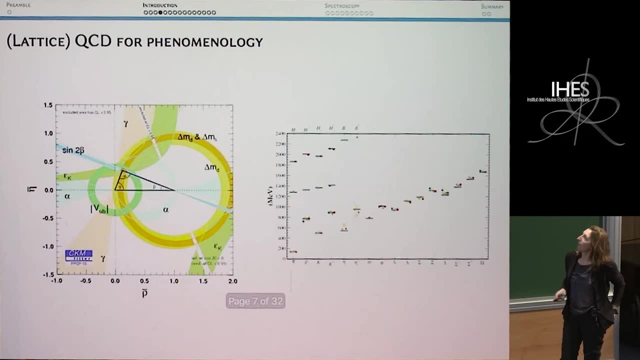 There are still very many puzzles and surprises that we don't understand, even though in some sense we know a lot about the theory. So just to highlight some progress. So this is a typical if you have been to colloquia in particle physics either theory. 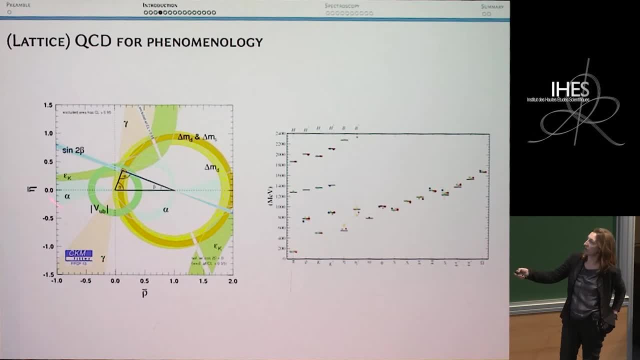 or experiment phenomenology, you'll see plots that look like this. These are the parameters of the CKM matrix, And so they parameterize the sort of the known standard model. If the standard model is complete as a unitary theory, then the triangle that you see here 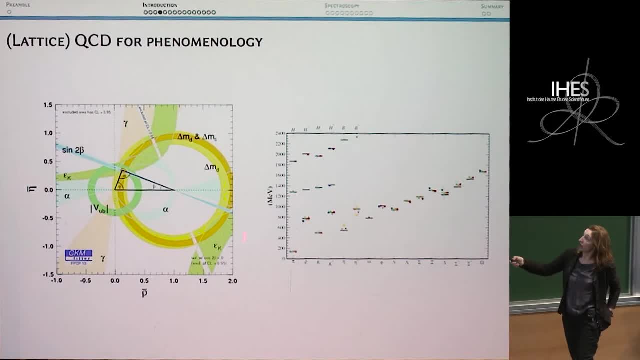 meets at the apex, the lines meet at the apex and the error bands, the colored bands, give you a sense of the uncertainty and the parameters that go into making up this triangle. So you see that the bands are certainly wide enough here that it's not yet fully proven. 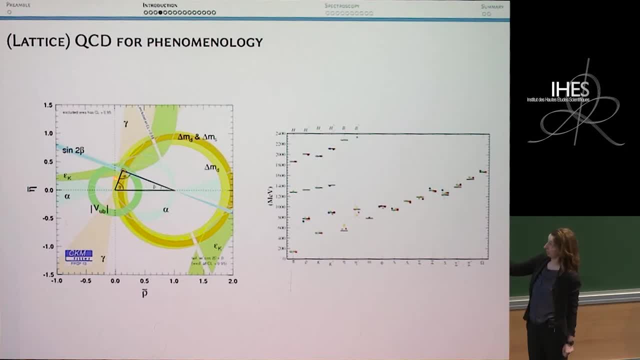 that indeed this is unitary, or indeed fully proven that it's not unitary. The bands are the combination of experiments. So you see here that the bands are driven by experimental and theoretical uncertainty, And by and large, most of the bands that you see here are driven by hadronic uncertainty. 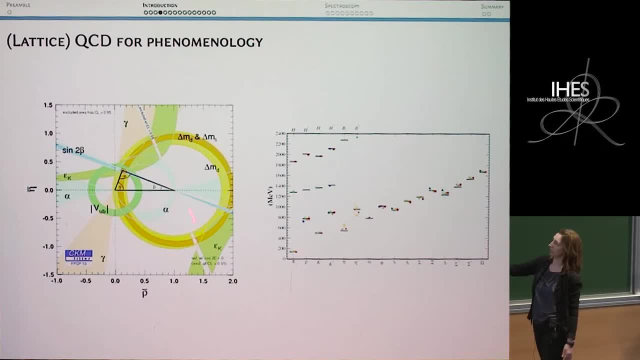 in particular theoretical uncertainty that comes from the QCD contribution to this combination of electroweak and strong interacting physics. So it is the job of QCD theorists to shrink the size of these bands, to understand more about this CKM matrix, in particular the unitarity or not of the CKM matrix. 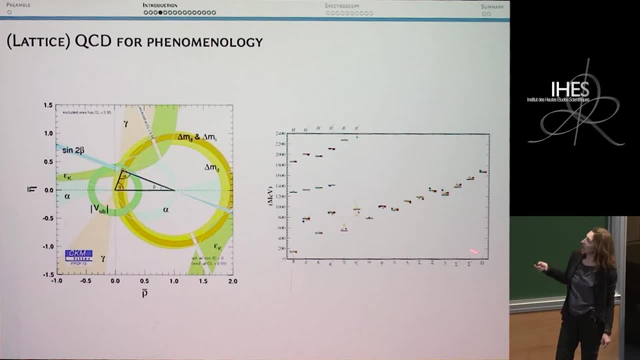 And over here apologize. this is a little bit small and certainly hard to read on the axis, so don't worry about that. so this is a sort of a universality plot. in some sense this is a collection of lattice calculations of many low-lying mesons and baryons. the different, the black lines first of all are the. 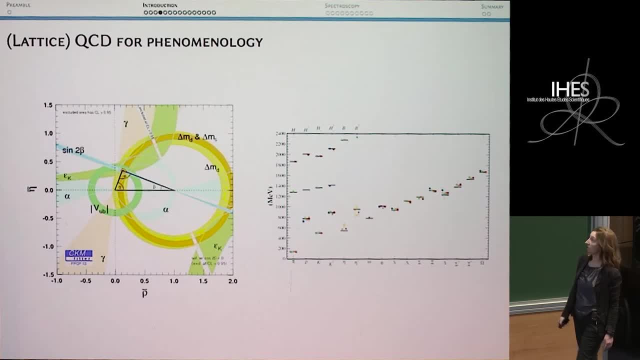 experimental measurements. the different colored dots are different lattice calculations, so these are done in many different ways. the fact that they all sit on these black lines is confirmation that, although we do things in very different ways, everything is agreeing very nicely with these low-lying measured experimental states, and this is true for light. these are like mesons and baryons. 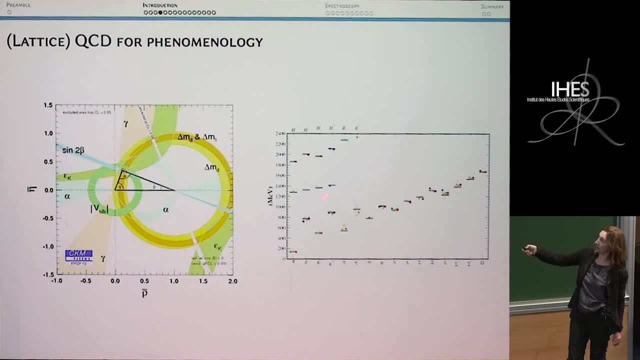 heavy light mesons and heavy heavy mesons and baryons. there's some offset here which I haven't included on the plot. so everything works very nicely, at least for this. this level there are also it. you need rather good eyes. but there are also some error bars on here and this is the result of the numerical 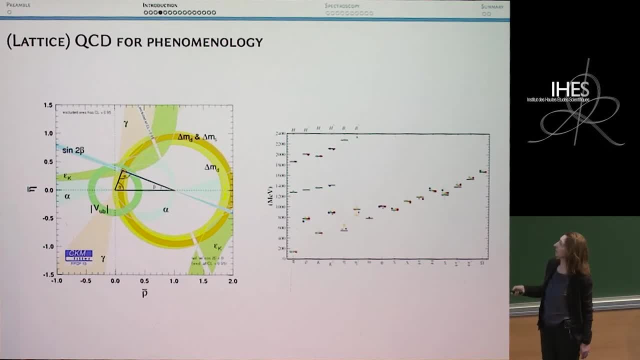 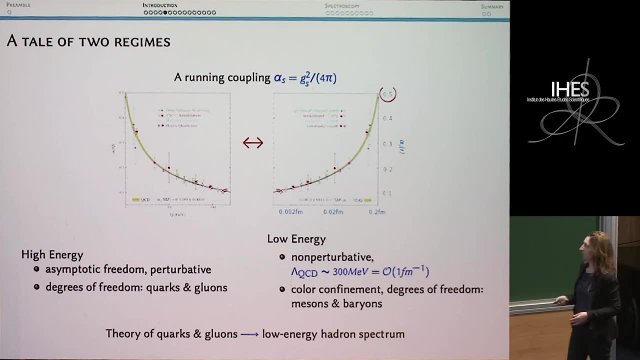 simulation, of course, which has both statistical and systematic uncertainties that go along with it. so for QCD, we know that essentially you can think about two regimes in QCD. so there's a high energy regime, so deep inside a proton, where the quarks are essentially free, with asymptotic freedom, tells. 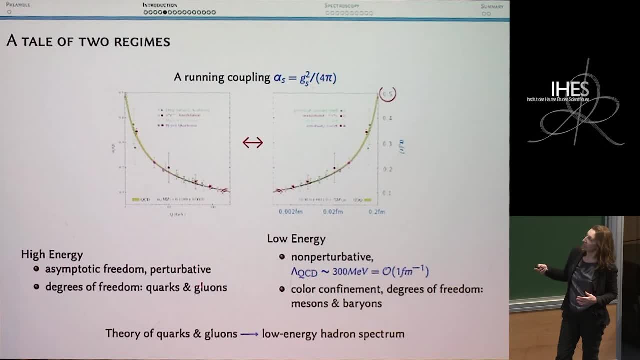 us that the theory is perturbative and in fact perturbation theory works very well in that regime. however, we also know that the coupling, the strong coupling, in QCD runs, and so at length scales that are of order, the proton, for example. so at lambda QCD is about 300 MeV. the coupling which you can see, I 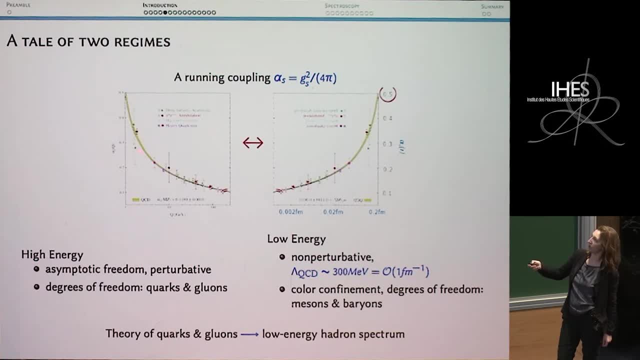 mean by some sort of lazy inversion, which I've done here. so you just reflect this plot. so this is in plotted, this is the running coupling as a function of the momentum transfer. so Q squared. if you just flip this, reflect this plot around and just relabel the axes in terms of the 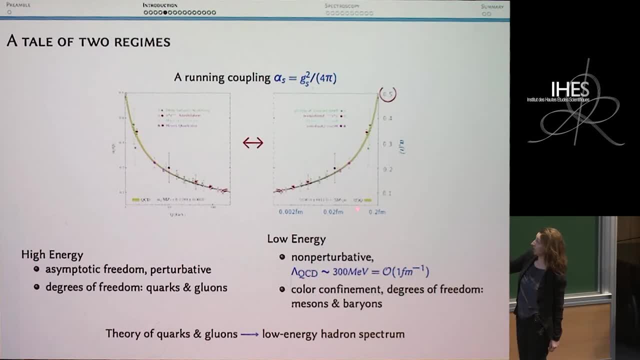 corresponding distances. so Fermi, you see that already by about 0.2. Fermi, the strong coupling is really strong, so it's about 0.5. and by the time you get to one Fermi, which is sort of so hadronic length scales, and this is a quite a large number and is certainly no longer an 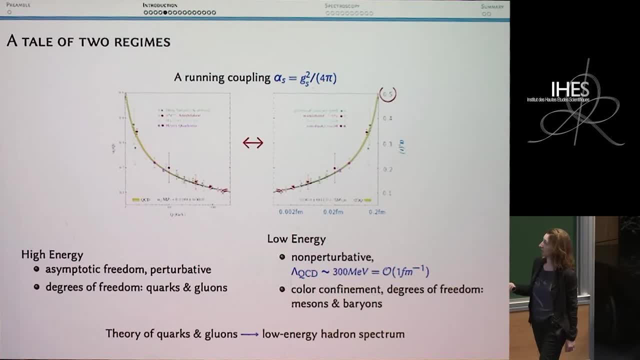 appropriate variable for a perturbative expansion. so a non-perturbative expansion, a non-perturbative treatment of the theories or is obviously required if one wants to understand the low energy hadron spectrum, the emergent phenomena in terms of the quarks and gluons, the fundamental 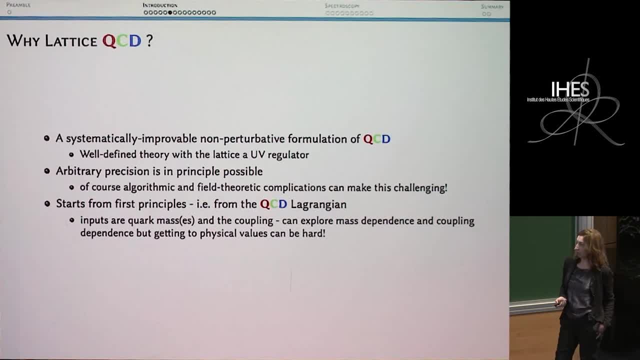 variables. okay, so why would you think about lattice QCD? so the lattice discretization approach is a systematically improvable, non-perturbative formulation of QCD. so the lattice provides a regulator in the UV, also in IR. in principle one can make calculations that are arbitrary, precise. there are, of course, reasons why this isn't true in 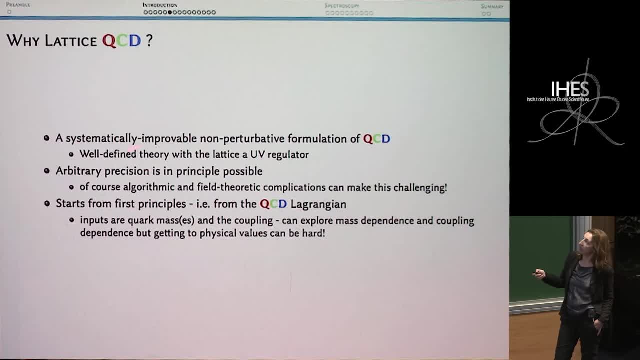 practically true. but we can understand in a formal way how to remove the uncertainties in these calculations and of course it starts from first principles, from the QCD Lagrangian. so this is not a model approach and the only inputs are the quark masses and the coupling. one can turn that around and 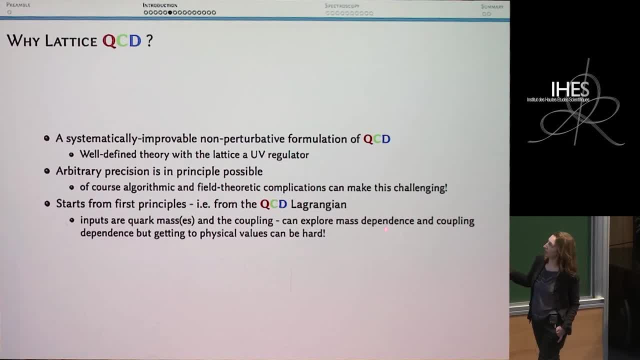 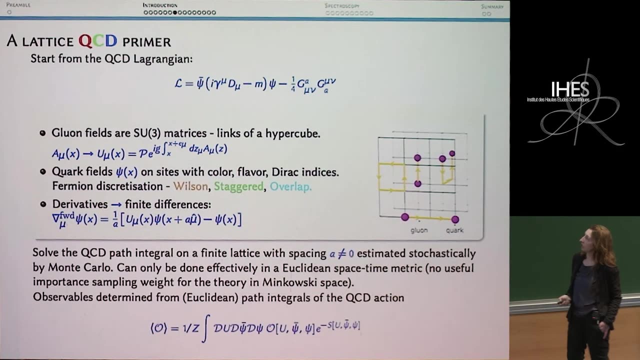 say that you can actually use the inputs then to explore the mass dependence and the coupling dependence in a very nice way, an avenue, for example, that's not open to experimentalists, since these things are given by nature, but here we get to dial them up and down as we want. so what do we actually do? so, as I said, 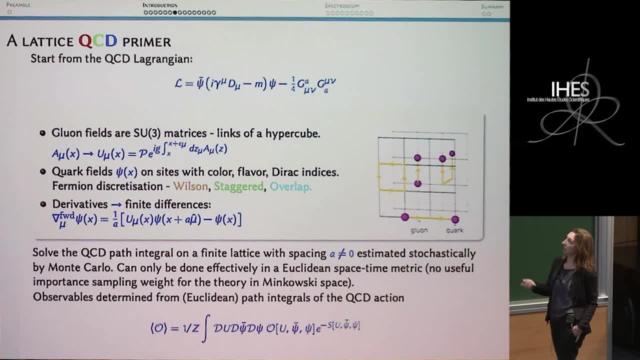 already. we start from the Lagrangian. you know I haven't included the theta term here, so this is the, the QCD Lagrangian. the cartoon over here is to show you how, how this might work. so the gluons are the su3 matrices. these are you think of. 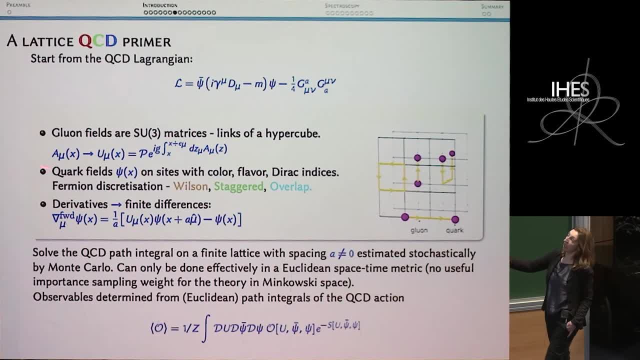 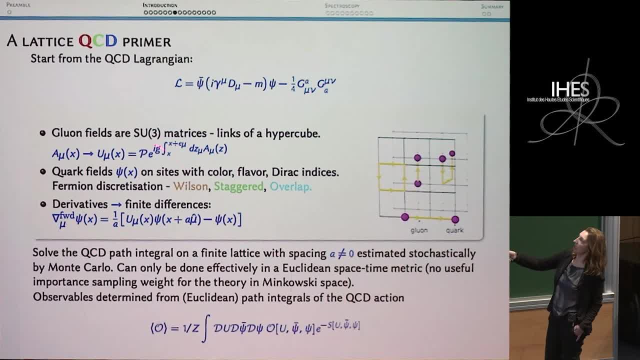 potential, the vector potential, here is rewritten as this link variable in this way, through exponentiation like this: this is a path ordered product of these, of these link variables. and here the quark fields then sit on the sides between the the links. so they have, they carry all of the relevant indices. so 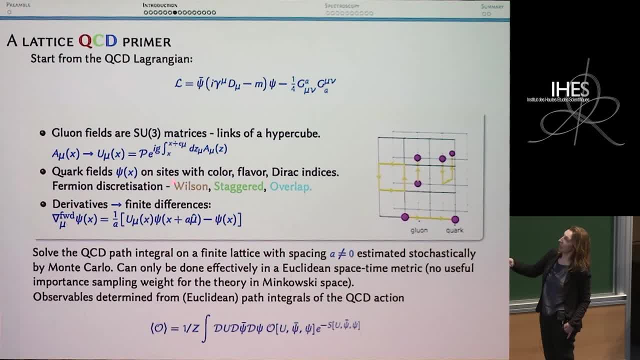 they have color and flavor indices, Dirac indices, and and precisely how you do this, is that you can see that there are a number of different types of this? is that you can see that there are a number of different types of sections, how you visual or how you implement this, these quark fields on the 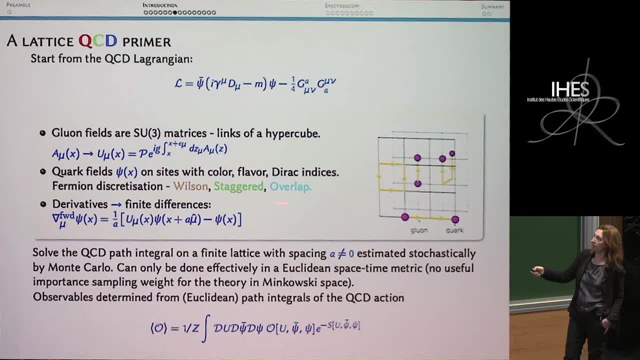 How you visual or how you implement this: these Quark Fields on the sites here in this cartoon, and are there are many different ways to do this there. sites here in this cartoon, and are there are many different ways to do this. there are pros and cons for all of these, wilson. 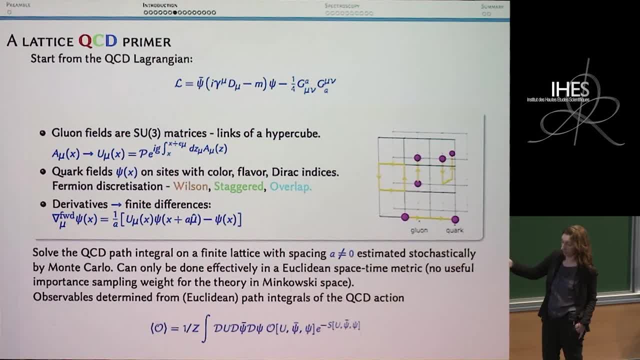 are pros and cons for all of these wilson families. on the first instance, these Wilson Sameans, Tamamians, explicitly facing Sameans, Azer internon, these Wilson Sameans BestWells, Farmy, New Zealand, chiral symmetry. and so some of these other approaches are different. 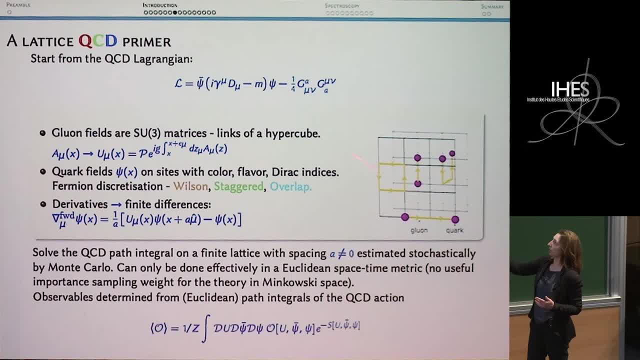 accelerations어요 trainings that are an attempt to rewrite the quark fields with remnant. equations that are an attempt to rewrite the quark fields with remnant Hor. salonけれぐ頰 Wexit policeman, NaF disc doubt the北ment. ребен Herman нужно碰. 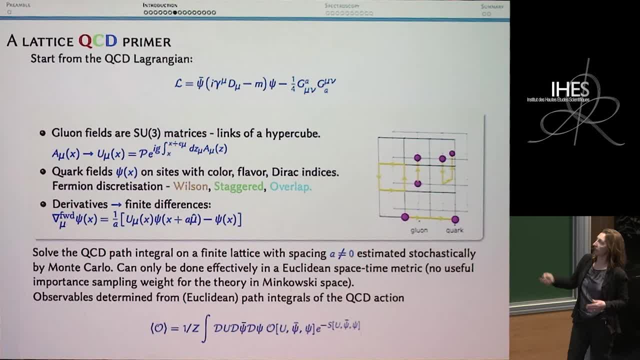 symmetry or indeed in some cases, full chiral symmetry. but they have other disadvantages that in some cases make you favor, Wilson fermions. The point is that if you, however, you do this discretization, once you remove the lattice, so once you take the continuum limit and recover. 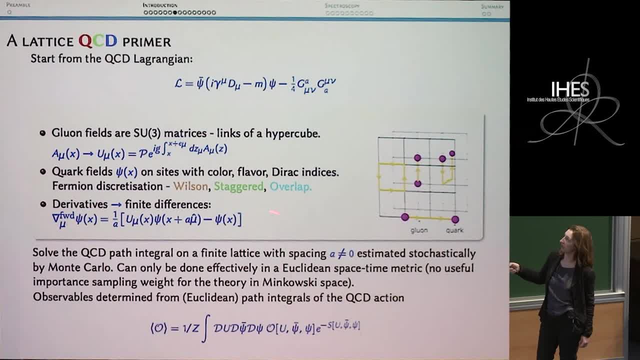 the continuum underlying QCD theory, then these discretization methods should all agree- and that's what you saw in the earlier plot, where all of these different colored dots were from different formulations along these lines- and finally agree. The usual numerical thing is to replace derivatives with finite differences, in this case with the, the link variables, ensuring that you have 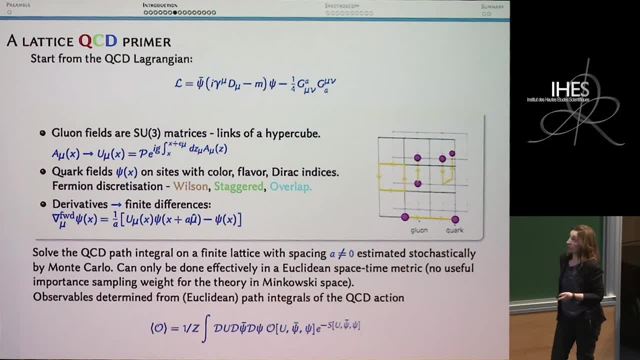 covariant derivatives in the simulation. So that's essentially the recipe. and then you solve the path integral on this finite lattice. so a is typically the, the lattice spacing. so this is non-zero. This is done stochastically using Monte Carlo techniques. The final twist in 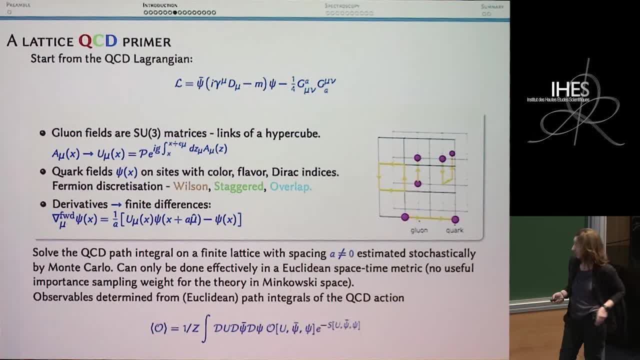 this tale, if you like, is that this can only be done effectively in a Euclidean space-time metric. so I'll say a little bit about that in a minute where you have essentially a probability weight that you can use in these stochastic estimations. but the observable that you might be interested, 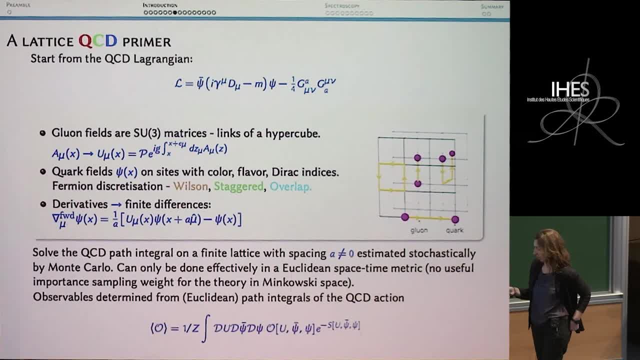 in calculating is essentially given by this path, integral here. so it's the evaluation of this right hand side object that we do numerically. Good question, and I see the term. do you have a way to put it on the lattice? It's a very good question. yes and no is the answer it. maybe I'll come back. 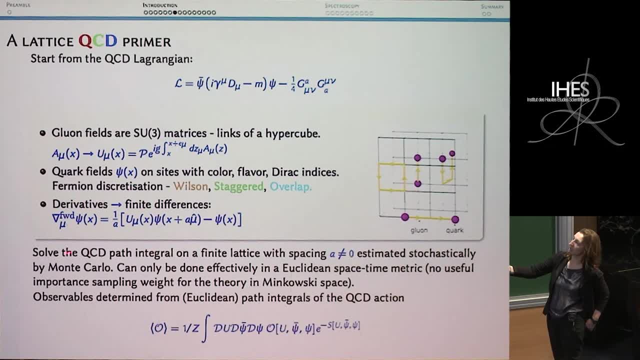 to- I'll mention it when I go, when I go ahead, it essentially me. it introduces a sign term, if you know what that is, and so this basically means that these Monte Carlo techniques don't really work very well, and so you have to find some other. yes, exactly, so you have to find some other way to do that now. 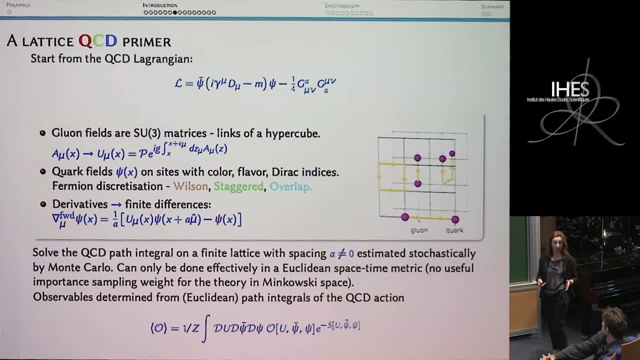 there are ideas about how you might do that for particular choices of theta but not for general choices of theta. I should also say so if you look in theories other than QCD, for example. so in SU theories we can do this with. we can understand algorithms that allow you to introduce a theta term for. 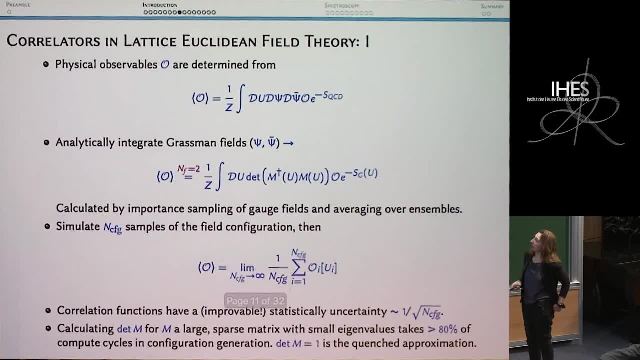 example, but just not in this full theory. Okay, so the observables that you want are determined from the path integral, something that looks like this, and so some subtleties here. the cork fields sine psi bar are Grassmann objects, and so we. these are anti-commuting objects. 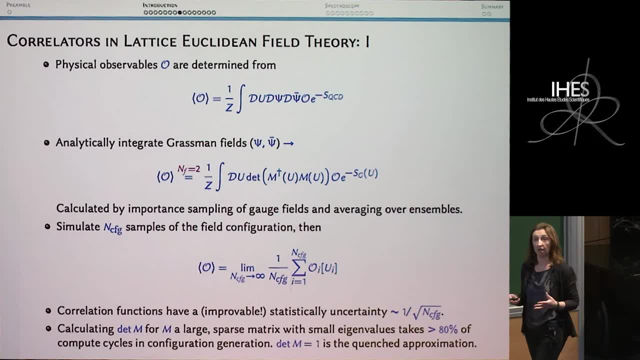 Variables, and computers don't like anti-commuting variables. you can't put these sorts of numbers, these sorts of objects in a numerical simulation, and so what we do is to integrate them out. by integrating them out, you introduce a determinant of the fermion matrix. so this is m here. I've assumed that I have two flavors and those two flavors have the same mass. 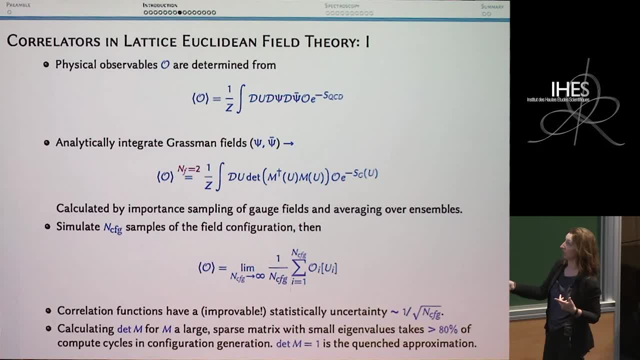 so this is true if you think about up and down quarks, the lightest quarks in the in the QCD vacuum. it allows me to write it down in a rather nice way like this: I should say that we also understand how to do additional quark flavors, so including the c quark in this determinant and also even the. 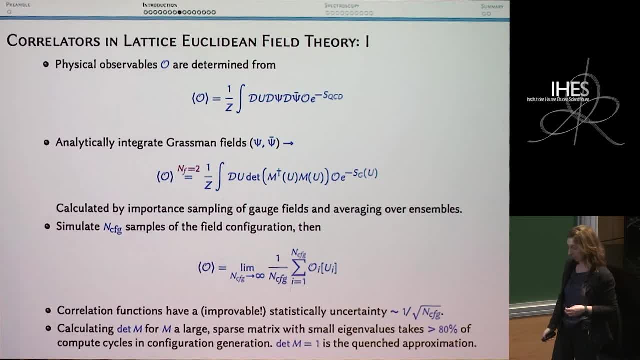 charm quark as well now, but this is a rather nice way of writing it down- in this particular case for two flavors, where the two flavors have the same mass, so up and down. so it is this entire object actually that is determined by important sampling. so the combination of this determinant that you 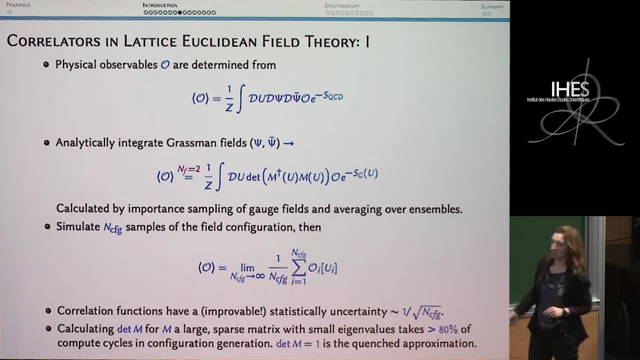 see here, with this gauge, action in the exponent can be interpreted as a probability weight. so to see that here the determinant is exponentiated by introducing some auxiliary bosonic fields and the whole thing is then rewritten as as an exponent, introducing also some conjugate momenta for the link variables. so 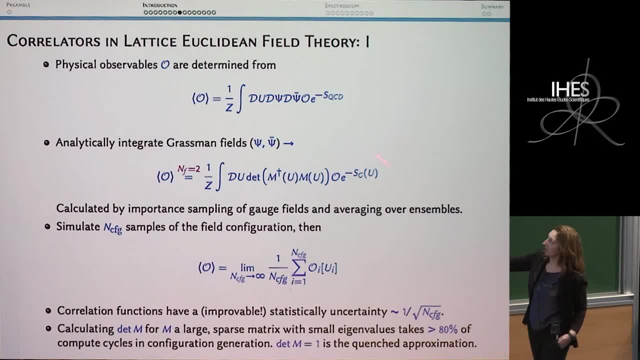 it gets a little bit complicated, but in the end you have something here which is positive, definite, to be able to look at and they can therefore be used in important sampling. so that's the key step to enable you to do that again. just to quickly mention so, this part here, so this determinant piece here that we've 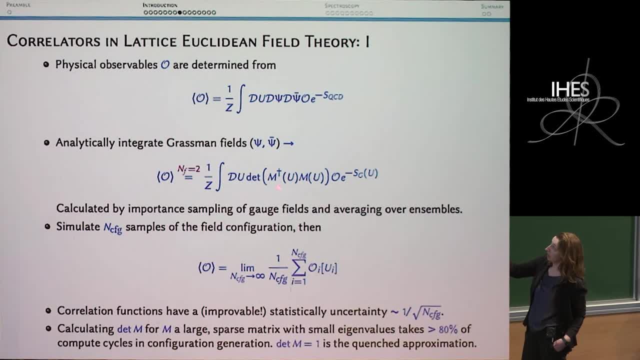 introduced because of the grassman variables, integrating these out. um, this determinant piece introduces non-locality, so that it couples the gauge fields in a non-local way. calculation, which means if, from a numerical point of view, you can't do. if you remember back to any computational classes you did for the easing model where you do Metropolis. 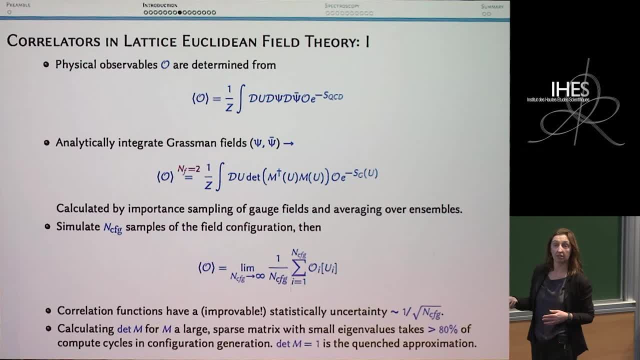 and Hastings and all of these nice algorithms. these rely on locality, And so instead, here you have to. in fact, it was recognized pretty early on. so a lot of people designed a new algorithm, called a hybrid Monte Carlo algorithm, to handle this non-locality. 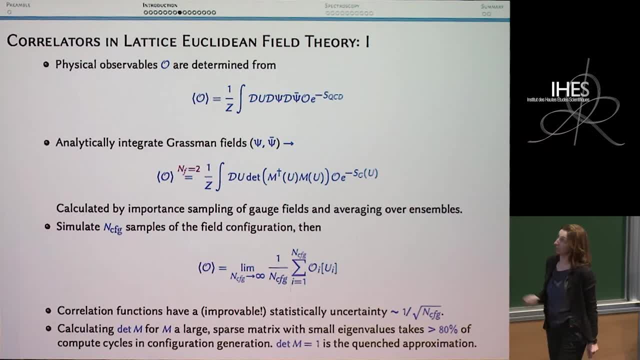 So there's some technical linear algebra that's basically hidden by what you see here. M is the fermion matrix, so d slash plus the quark mass, essentially Okay. so if you do this, so you evaluate this in some stochastic way again for these important 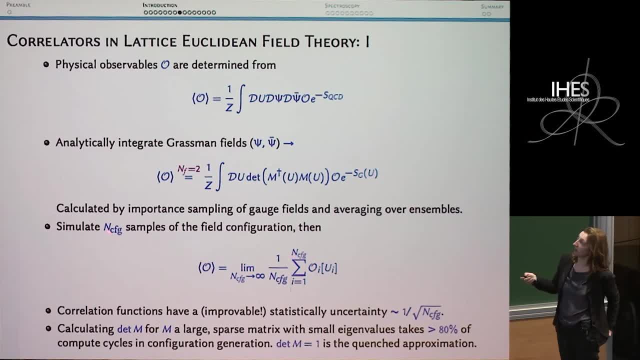 sampling, you have to demonstrate detailed balance and ergodicity in your algorithms. But anyway, if you do that, then the object that you're still interested in here, which is this expectation value of some observable O, can be written As the just the average of the object that you're interested in. so this observable 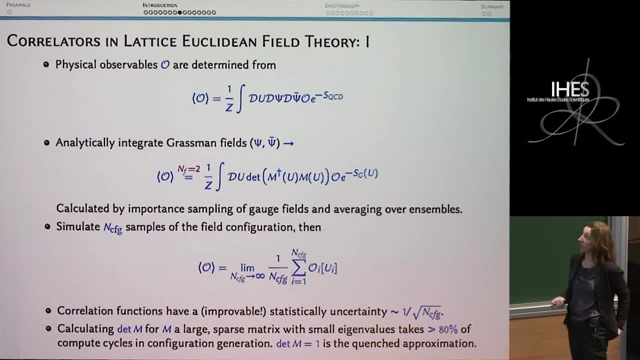 evaluated on each of the stochastic samples that you've taken in the limit where you take a large number of these things, And so you can show that this is again. this is rigorously true, with some correction terms that are understood in the limit where n is not, when n is finite, not infinite. 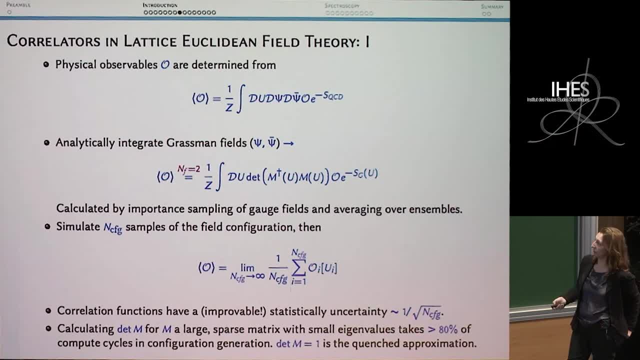 And, in particular, you can show that that uncertainty goes like one over the number of these snapshots that you're willing to do, And so you can show that that uncertainty goes like one over the number of these snapshots that you're willing to generate. So we have a controllable, improvable statistical uncertainty in these Monte Carlo simulations. 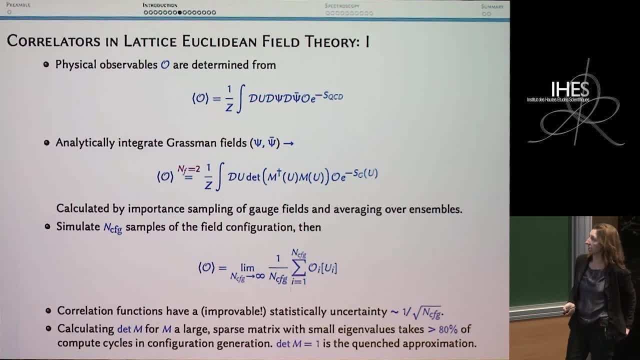 Calculating. this piece that I wrote up here actually is what lattice people spend an awful lot of their cycles doing. So this takes about 80% of the compute cycles in the whole generation process just doing this determinant piece that you see here. So if some people here may remember that in the early days of lattice calculations, people 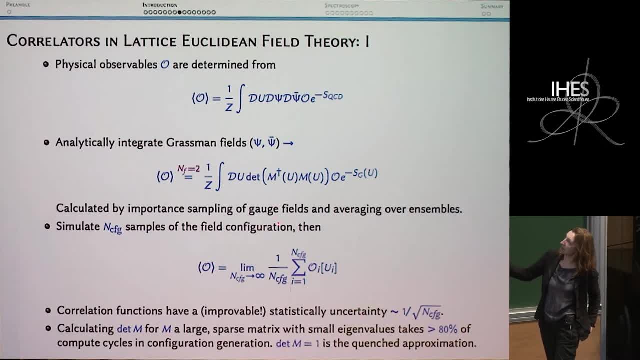 talked a lot about the quenched approximation Lattice calculations. That essentially sets this entire piece here to one and throws it away. so you don't include quark annihilation diagrams in the simulation. But that's completely. we've moved on from there now, so this is no longer part of any. 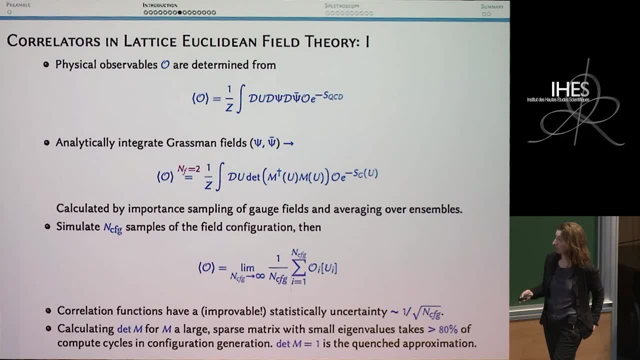 calculation anymore. So this: most calculations are unquenched these days. So the sign problem now is under control. No, No, no, no. So here this is assuming everything here. So QCD here Here means QCD with zero chemical potential. so I haven't talked about the sign problem. 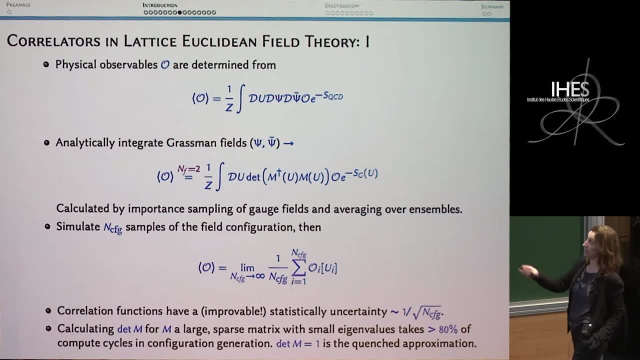 at all. What the chemical potential does is to complexify this determinant piece, and then we don't know what to do, because then the problem essentially is an algorithmic one, not a philosophical one or a physics problem. The problem is that this is complexified and now you have no positive, definite weight. 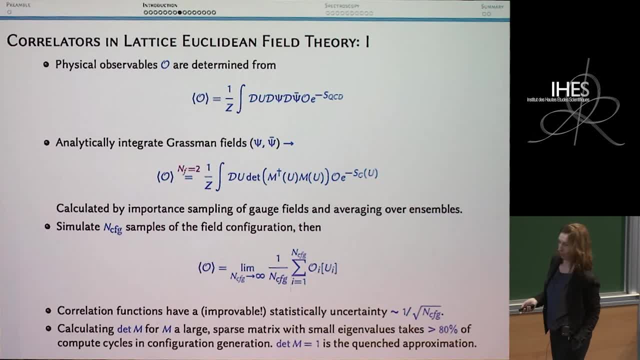 for your Monte Carlo sampling. So the answer is no, No progress. No, No progress to the extent that you can approximate small values of the chemical potential. but that's not an algorithm. That's just an attempt to understand what's happening as you move a little bit out of. 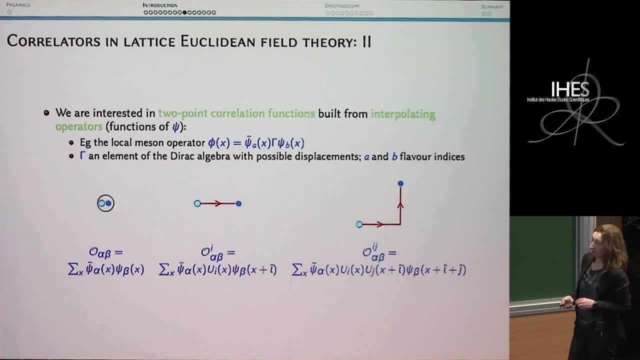 the plane. So no, absolutely, it's an open problem. So everything that I talk about here is in terms of zero chemical potential. Okay, so the objects again that we're interested in are these. let's say, for example, for mesons: 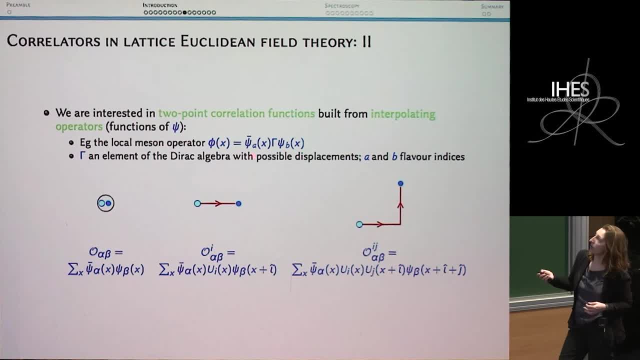 we're interested in two-point correlation functions. We build these out of operators. so this is psi bar psi, With some Dirac structure in here to give you the object that you're interested in. So this gamma is an element of the Dirac algebra, but you can also include rather fancy versions. 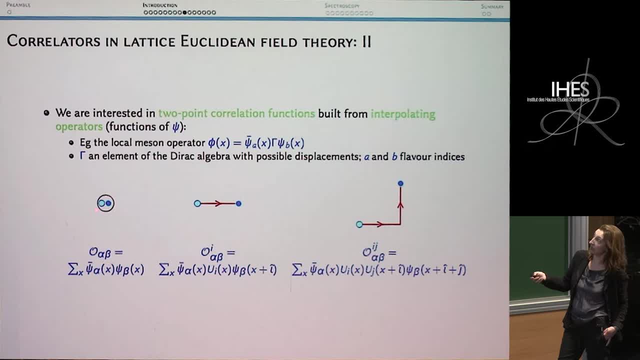 of displacement, so you can have a quark and an antiquark sitting at the same site, or you can pull them apart, or you can do fancier paths like this, and so this is what these operators would look like for these different scenarios. so you're completely free to do. 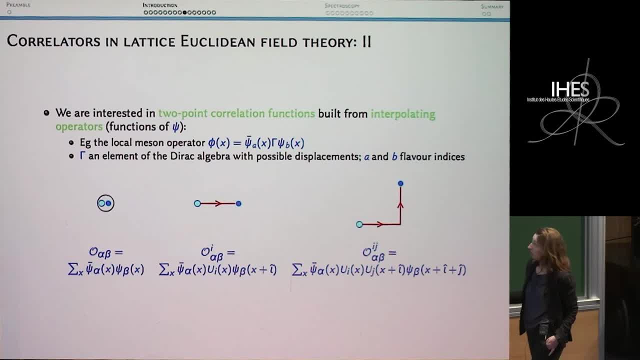 this. All of these will have particular quantum numbers that they overlap with, and these all form part of sort of a calculation that we do. So there's an immense freedom to design operators in this way, so you don't just have to sit with everything sitting on the same site. 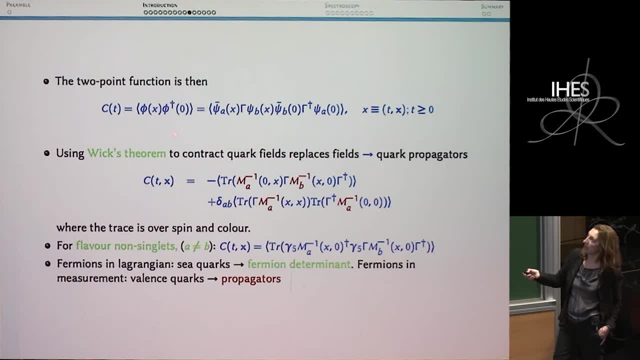 The correlation function. the two-point correlation function, then, is the expectation value of this creation and annihilation operator which, in terms of the quark field- so for some flavoring- which I've just written here as a and b- I've suppressed the other indices, just for clarity. 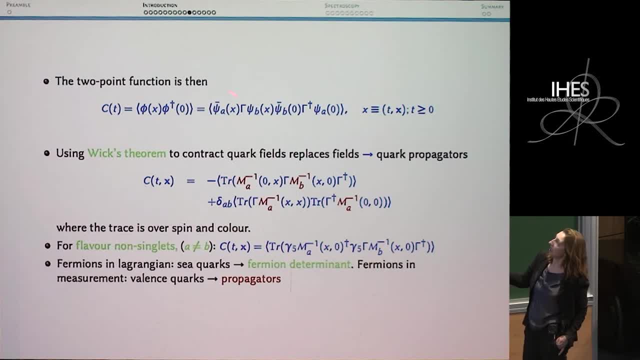 So you have psi bar psi at some value, x psi bar psi at zero, and this object is what you want to evaluate for each of the stochastic ensembles that you've already generated. So to make some progress here, we use Wick's theorem to contract the quark fields. that 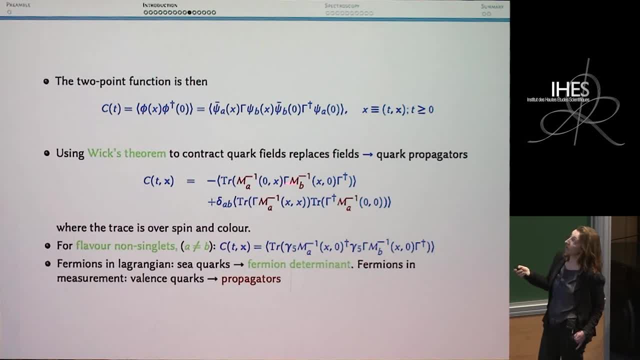 you see, in this correlation function. so by contracting the quark fields, we replace them with quark properties. Okay, propagators. and so you see this is the same capital M. so this is now the inverse of the fermion matrix. so d slash plus m appearing in here for some flavor that you get to choose. 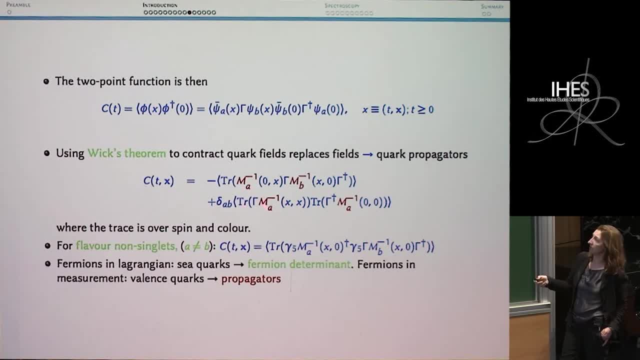 so A or B in this case, And the trace is over spin and color indices. So for non-flavored singlets, when A and B are different, this simplifies to this expression here. However, when A and B are the same, you can see that this term here in particular remains. One thing just to maybe. 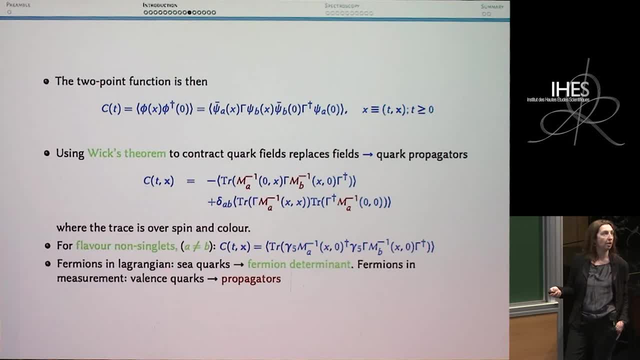 emphasize here is that the fermions enter in two different places in these lattice calculations. So they enter in the previous slide where I was talking about the determinant and the evaluation of the determinant, and then they enter again here when we talk about propagators. So here: 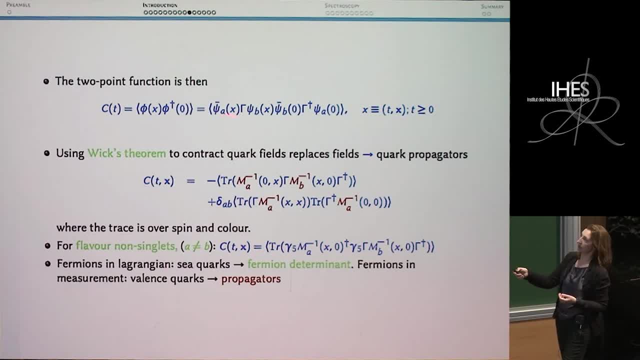 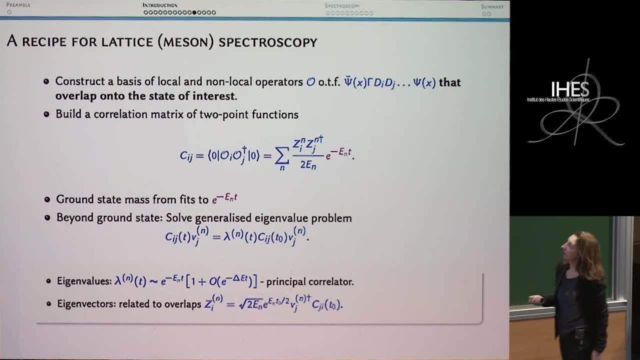 for these correlation functions which are built out of quark fields which can be of any flavor. Okay, so then, to actually evaluate this again, this correlation function, we, in principle, or in practice, sorry, what we do is to build many of these operators using the. 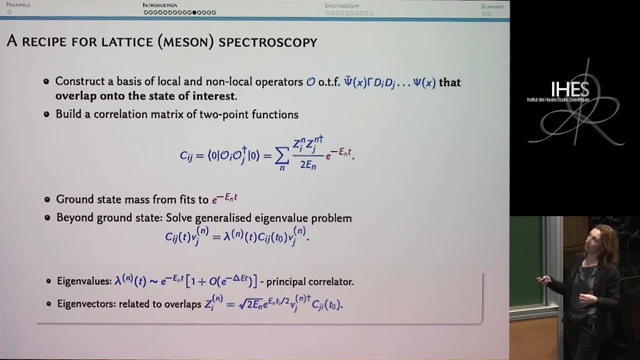 cartoon that I showed you a little while ago as a sort of a motivation. So you can imagine having a quark and an anti-quark on the same side, pulling them apart, doing random different paths like that with them, and you build up a matrix of these operators and you can see that. 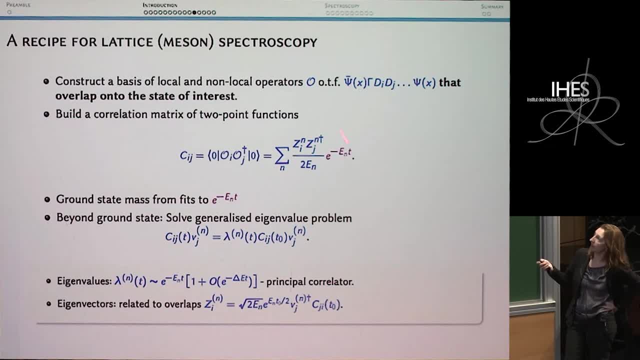 if you build a very complex case like this, then you don't get any of these racist problems. Now, in general, if you look at the very basic elevators and again in this euclideanized field theory, you can show that this: 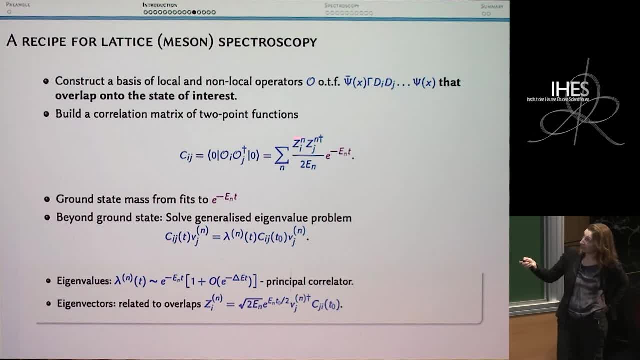 correlation function that you have written down essentially has this structure here. So it's a tower of exponentials with some stuff, some amplitude in front, which for the moment we won't worry too much about. The main thing to note here is that you see, there's an exponential. 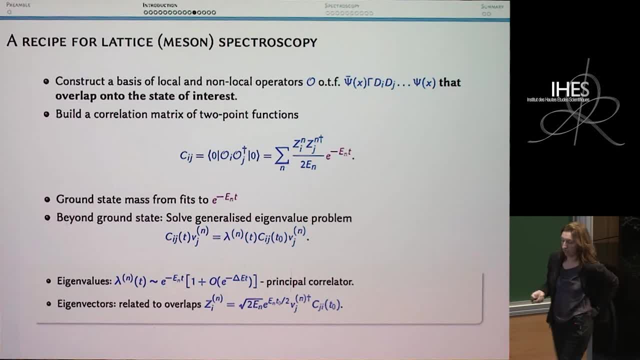 which has the energy that you might be interested in upstairs, And so with a factor of T, And so if you were interested in some of the Dos'S, look you have a. if you were interested in the ground state, so the lowest lying state in this particular channel. 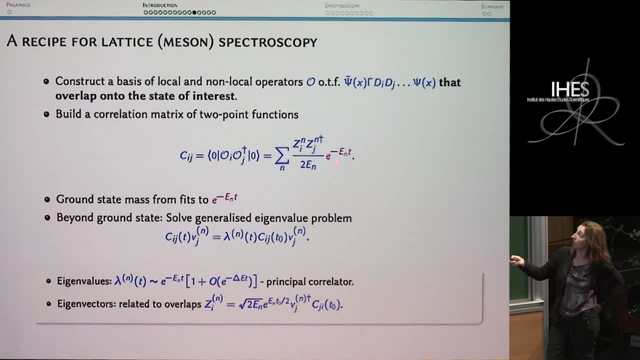 then you just have to wait long enough and then the ground state exponential, the lowest exponential, will dominate in the correlation function. If you are interested in other things beyond the ground state, then we solve a generalized eigenvalue problem with this matrix of correlators. 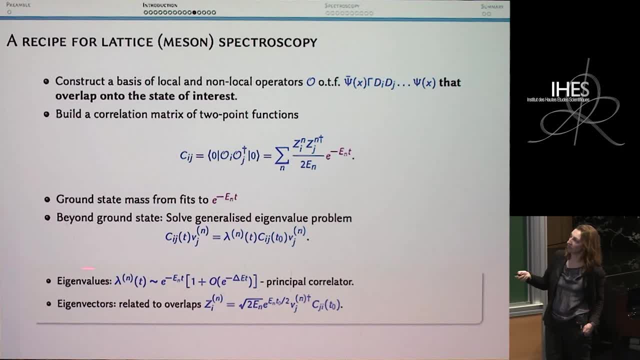 and by diagonalizing that correlator matrix you can extract eigenvalues and the eigenvectors, and the eigenvalues are related to the energies. again, it's the same energies that you see here, but in a more straightforward way, so you can. each of the eigenvalues is then associated with one of 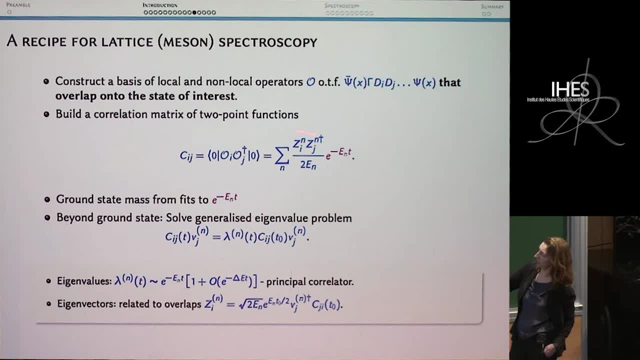 the energies in the this tower that you have here and the eigenvectors are related to these overlap or these amplitude factors that you see in front here. So there's been a huge amount of work in the field actually to understand how that this, how this actually works. so there's- there's a number of different issues which i haven't, which 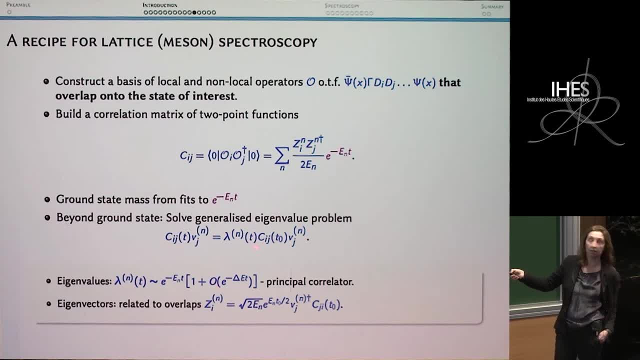 i'm glossing over here. one is: how do you actually construct in some sensible way these matrices of operators? the second is to understand what the uncertainty is in this generalized eigenvalue problem, in this solution. so how do the energy eigenvalues relate? how do the eigenvalues relate? 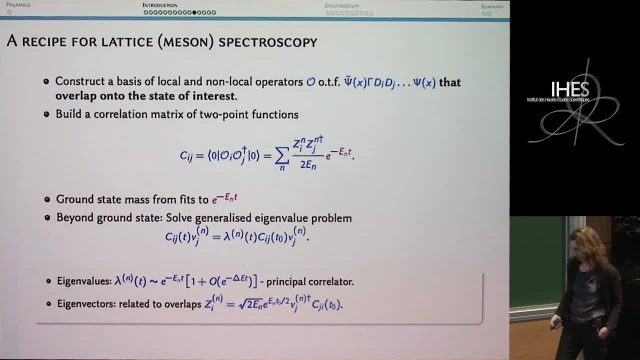 to the energies that you're interested in, and with some correction factor. and then the final piece of work that has only recently happened is to understand how to use these overlaps- previously we just sort of threw them away and didn't worry about them- is to use these overlaps, in fact, to help you to identify. 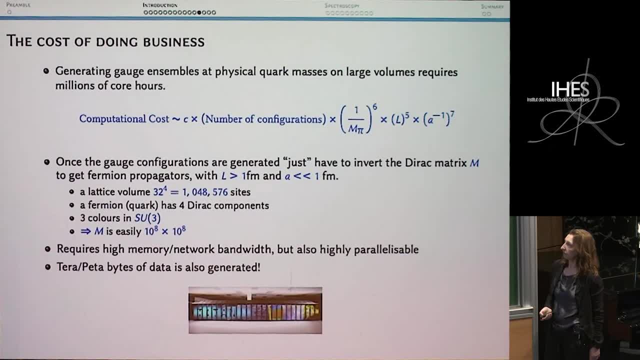 states in the lattice calculation. Okay, so very often you hear a lot of people- in fact i've already been doing it- talking about: oh, you know, we need big computers and everything takes a long time. um so, um. so this slide is just an attempt to sort of say why, or show you at least what's. 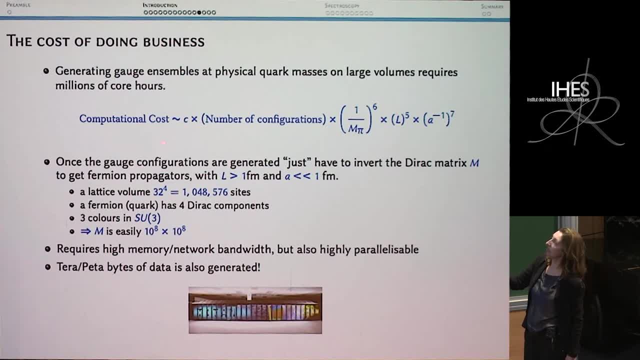 happening. so this is a the computational cost of some lattice calculation, in particular of the part where we're calculating the determinant. so there's a couple of slides ago. so of course it depends on the number of these stochastic samples that you're going to calculate, but that's actually not the. 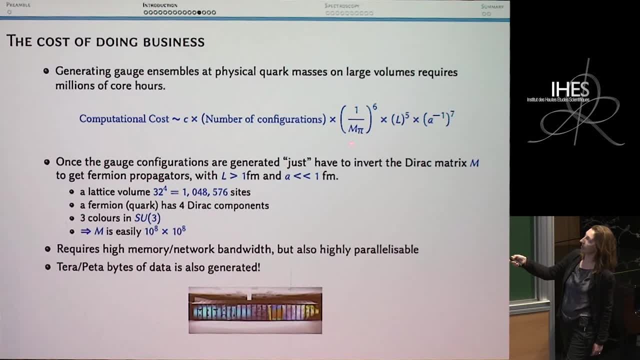 problem. the problem is over here, when you start to think about how it scales with some of the things that you control. okay, so you control, for example, the size of the box in which you're willing to do your simulation, but the cost scales like the volume to well, L to the power five, so the size of the box. 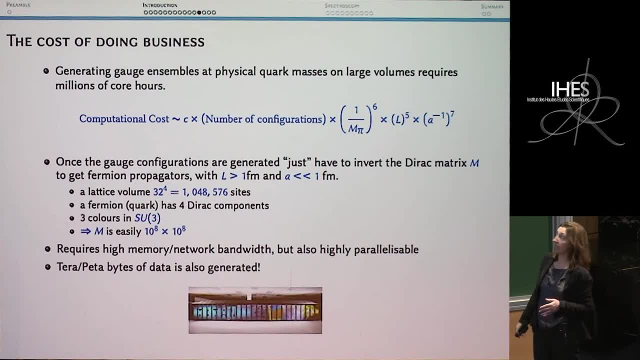 with a fifth power, It also scales with the lattice spacing. Again, that's not unexpected, but it scales rather badly with the lattice spacing. So it scales with this seventh power. here A inverse A is the lattice spacing, remember. So as you decrease the lattice spacing, 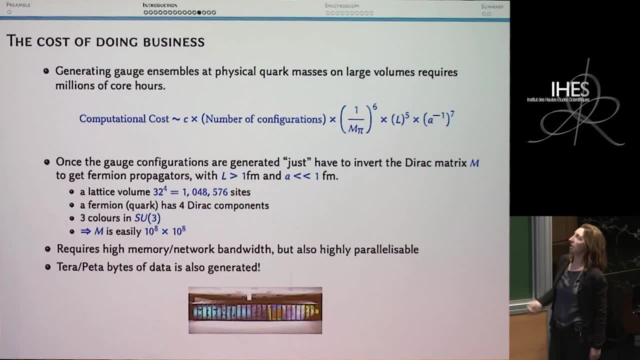 which is moving towards the continuum theory. the cost is growing by a rather enormous factor And finally the cost also grows with. so m pi. here the pion mass is a proxy for the quark mass in the determinant. And you see again that this, as you go towards physical, to very 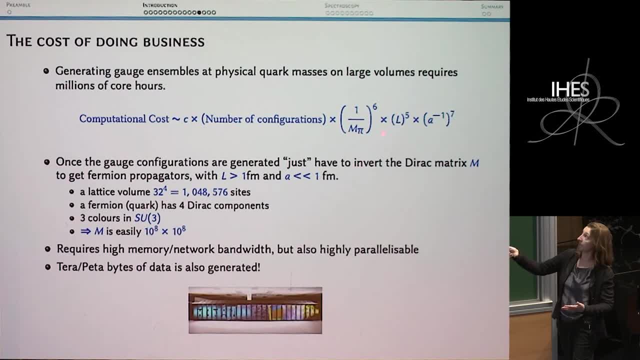 light values of the quark mass, which is like physical pion masses. this scales again with a very uncomfortable factor of six upstairs. The combination of this scaling, which is built from some of it, is certainly physics. so m pi for example. 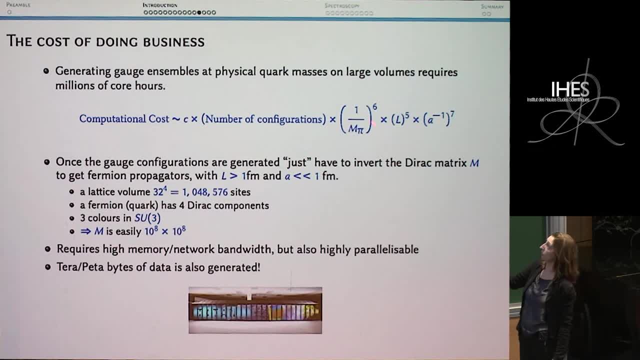 scales like the square root of the quark mass, but some of it is algorithmic and some of it is geometric scaling, But the combination is essentially what- the 80% of the computational time that these lattice calculations are doing, where it's going to. This has a name, so this was. 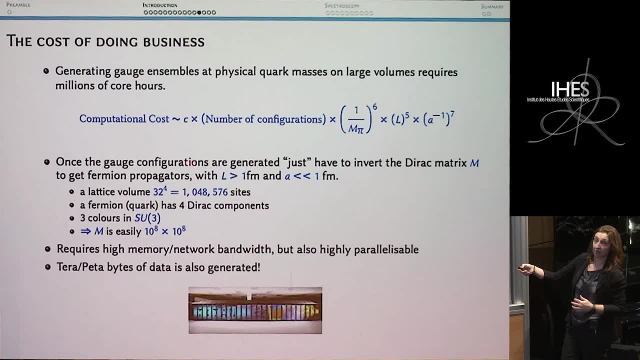 called the Berlin Wall mostly because it was discussed at a lattice conference in Berlin, so it's a little bit dull in that sense. But actually the wall was the, the wall that you hit in this computational cost as you try to scale down in to light pions. 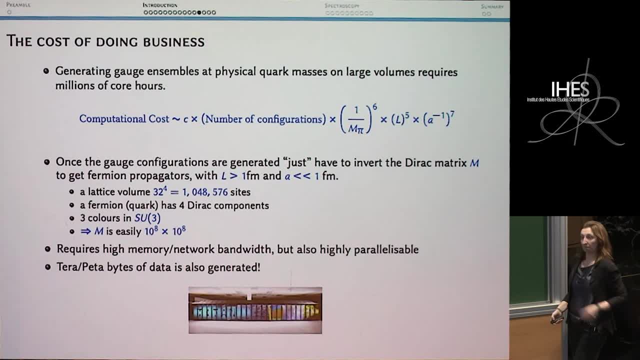 large boxes and small lattice spacings. So why isn't L over A to the fourth the correct scaling? It's algorithmic. So there's a. so there's a, there's a. there's an additional factor again, partly because of the nonlocality in the determinant, So that 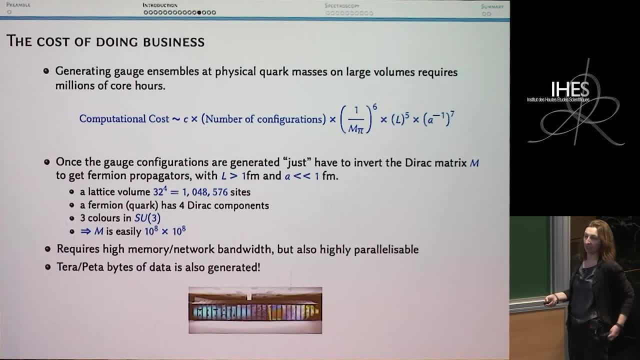 affects sort of everything. I mean it brings additional. the way you handle the determinant brings additional factors of A and L into this. Excuse me, why? why the combination of the parameters is dimension full. No, sorry, sorry, the C, yeah, so the C. here is some parameter that is. 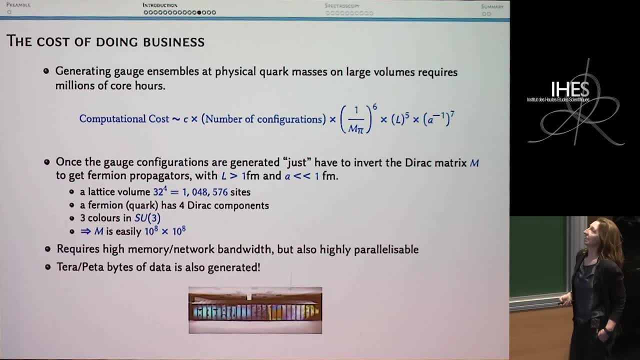 will have dimensions to. yeah, to fix that. yeah, Sorry, I should have said that. Okay, so so this is the Berlin Wall, essentially. I'll show you in a little while that, that the wall has come down And in fact, we at least understand how to. 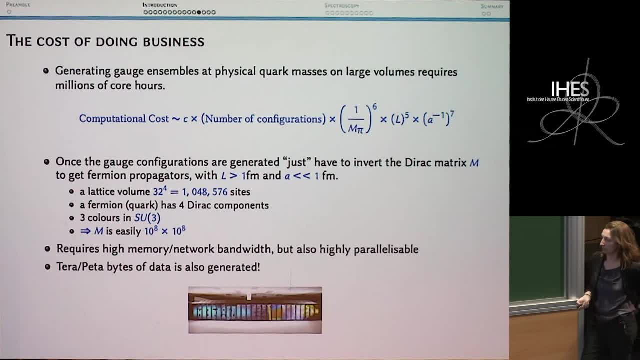 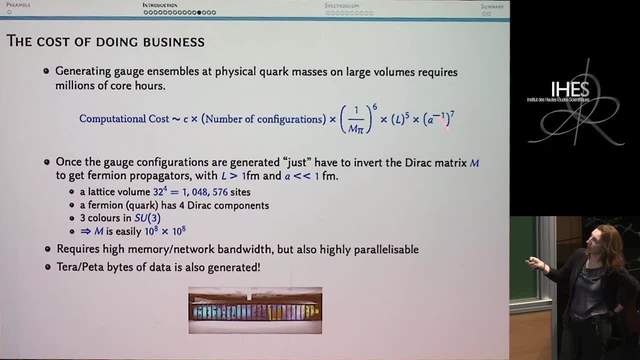 However, it doesn't actually stop at that point. So once you do all of this work up here, then you have to do the calculation of the correlation functions, which again requires you to invert this fermion matrix, as you saw a couple of slides ago. 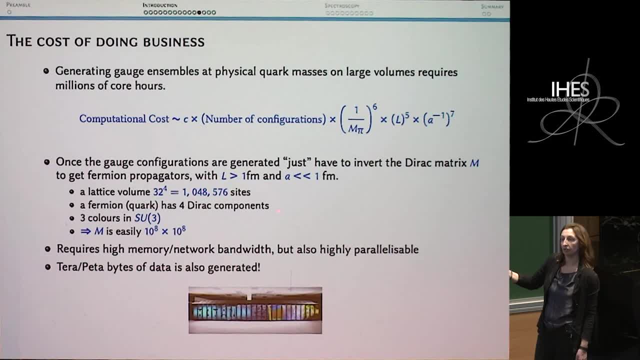 And so you have some things that you need to worry about. you need a box that's big enough for whatever it is you're trying to calculate, or some beyond the, you know, larger than least one Fermi- much larger usually these days- and you need to have a lattice spacing, which is 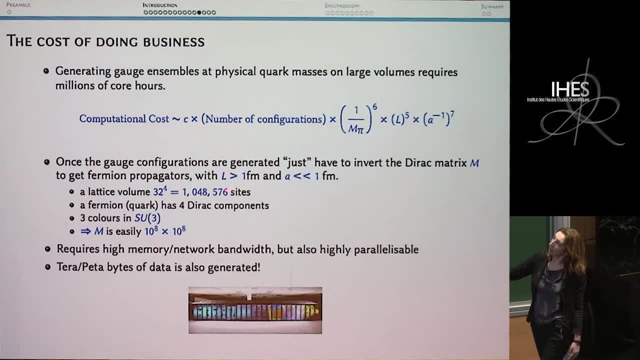 much smaller than the volume of the box that you're simulating. So a typical sort of volume might be 32 to the 4, that's already over a million sites. and of course your fermion fields have Dirac components, colors, and then the combination. finally, in this Dirac matrix is usually 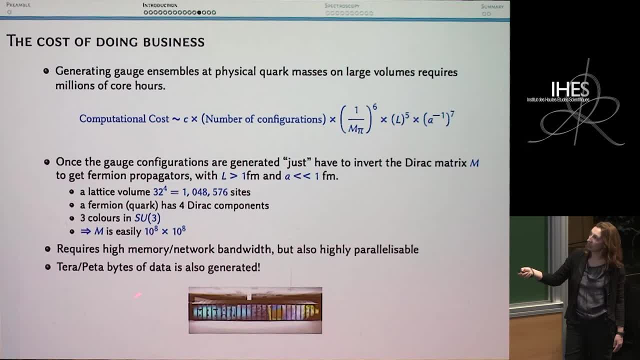 or easily. sorry, is this sort of size. So this is the matrix that you have to then invert on each of the configurations that you generated at this cost up here. So the whole thing is an enormous, hugely intensive computational cost, but it's also highly parallelizable, so it's very 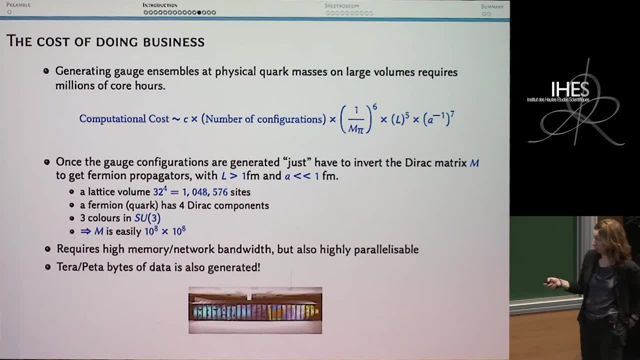 suitable for these sorts of machines. This is Titan in the US where a lot of the calculations have been done. so it scales very well on these large machines And, just to prove, it's been around for a long time. so here's a. 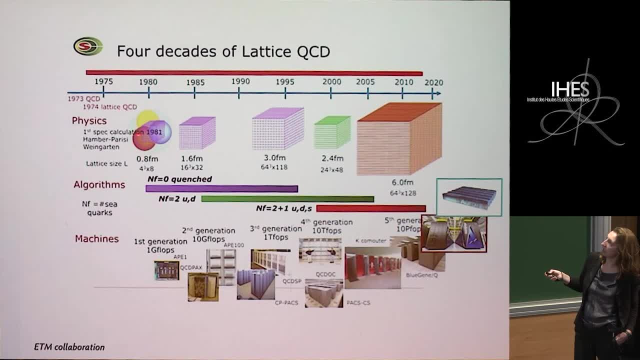 snapshot of QCD from the early days, lattice QCD, from the very first numerical simulation. so everything was quenched. you can see the boxes were relatively small. So we're up here. and then the machines are somehow keeping track of all of this as well. so the boxes get bigger as the machines get bigger and 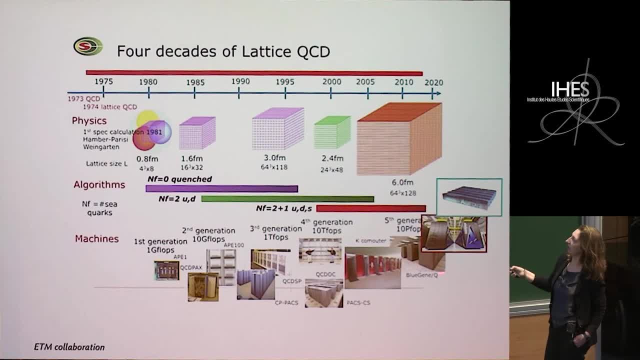 here you see that the box now is about six Fermi and is rather large number of sites and this is at the stage of what they call the fifth generation or blue gene, IBM's blue gene machine. So more recently, this is Summit. this is in the US. this is an almost exascale machine, so this runs at a few hundred. 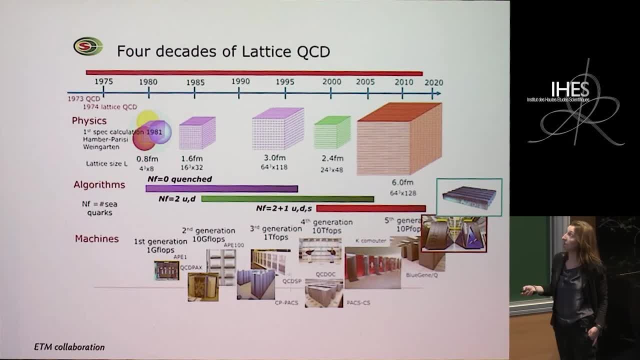 petaflops, where a petaflop is about 10 to the 16 floating point operations per second. So this is at least last year was the top- was the fastest supercomputer in the world. it's also one of the greenest supercomputers, so that's also quite nice. No, no, seriously. 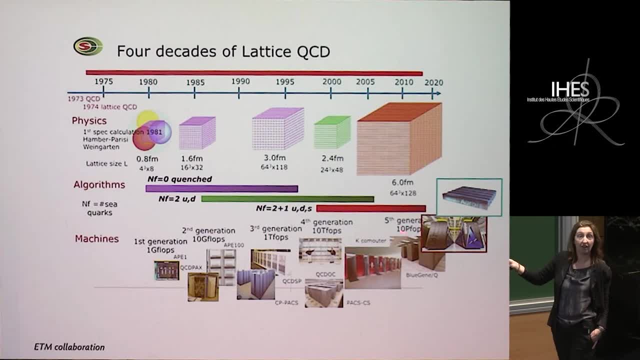 this is a big thing now. so these machines have to be not just fast, but green as well. they have to be energy efficient, because they use an enormous amount of power, And then this one here in a box doesn't quite exist yet. this is coming in 2021, this is the first exascale machine. 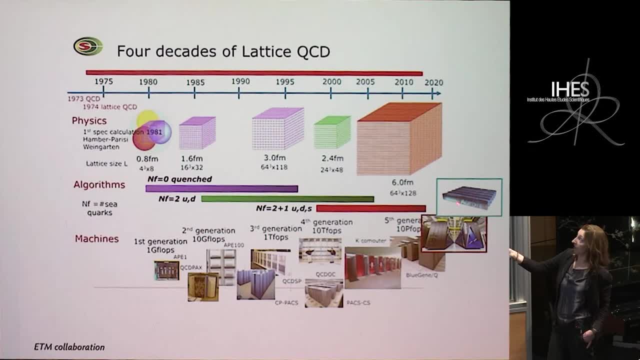 this will be doing 10 to the 18 flops, so floating point operations per second and to go from here so this is about 200 petaflops to over a thousand petaflops in three years is the ambition and it's really rather significant to try to imagine how to. 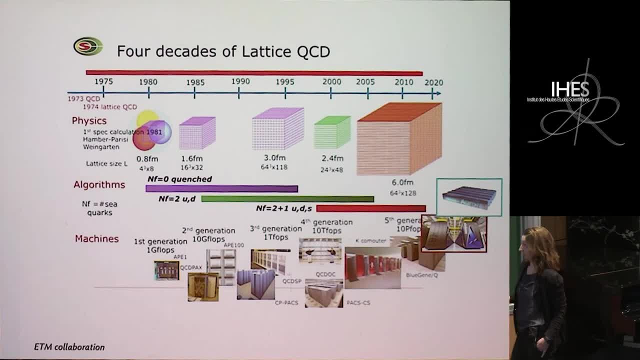 make that transition in these sort of numerical calculations And the final goal is to compute some matrix element or what's the For lattice people. Yeah, so maybe I'll say at the end: but yeah, so I mean we've moved long beyond just reproducing what experiment does. that's already. 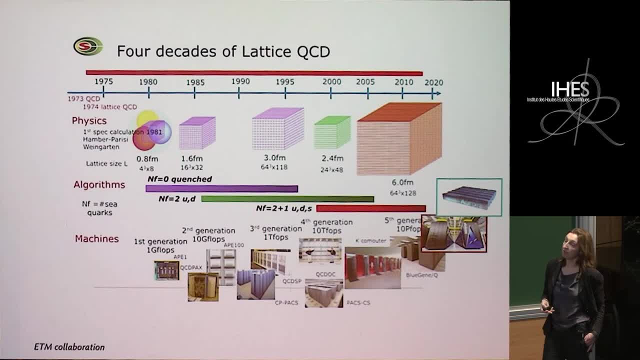 sort of you know, I would say proven So- matrix elements are already calculated and they were part of, for example, that plot that I showed you for the CKM matrix element. But there are many other similar quantities, for example contributions to G-2,. 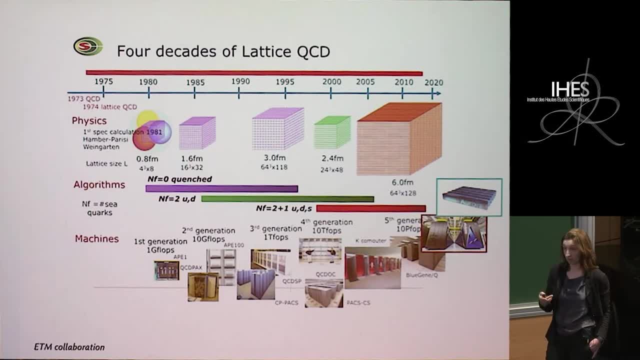 the anomalous magnetic moment of the muon, where there the matrix elements are rather complicated objects. they have a light by light structure in them and they're extremely difficult to calculate. They have many. they have vacuum polarisation diagrams as well. so this is a 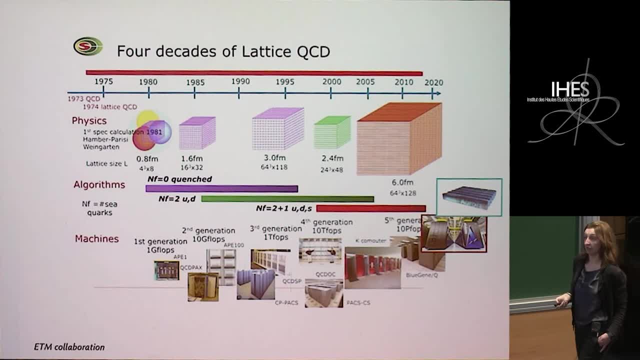 very difficult problem And this is, I'd say, the early lattices, at the early days of these, and I'll show you some other things where we're at the early stages of trying to understand how to make the calculations. So these, of course, 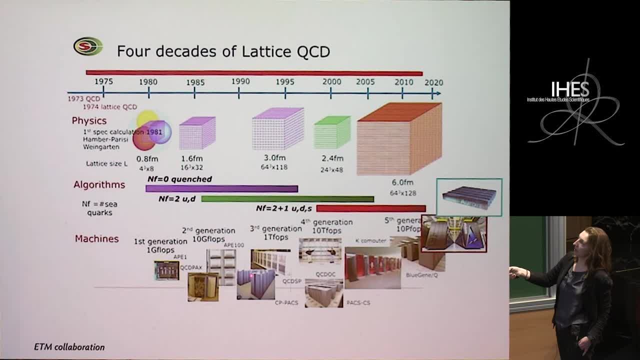 the bigger computers help. but as you saw maybe in the earlier slides, you also have to be quite clever about how you do the algorithms, because if you just wait for these big machines, then you won't really make very much progress. you have to also improve the algorithms as well. 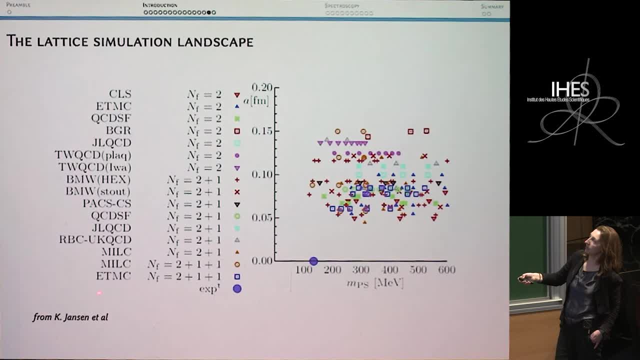 Okay, so this is a long list of lattice collaborations, which is not important really, but just to show you that this is the Berlin Wall coming down, although maybe not as so obviously. So here's the physical point. this is the pion mass. 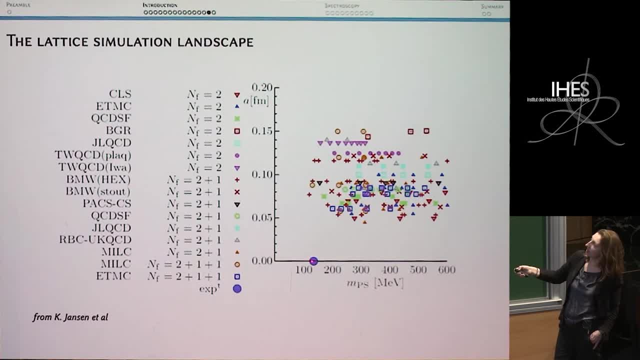 and this is the lattice spacing here. So you want to be down here, right? this is the pion mass in MeV at zero lattice spacing and the lattice calculations are all up here. So of course they're not at finite lattice spacing, which would be down here, so they're still at. 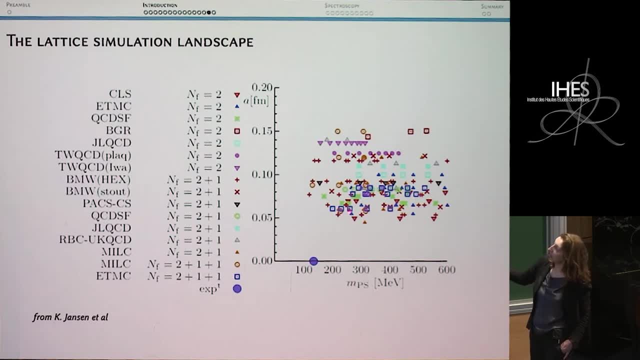 fine, but not close to zero yet. But they are at physical pion masses. so I'm not sure if it's so clear, but there are certainly some points which are very close to the pion mass. there are some points which are at the pion mass and there are some points which are actually even lower than. 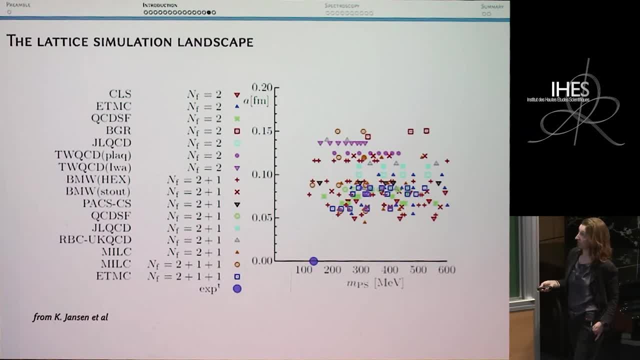 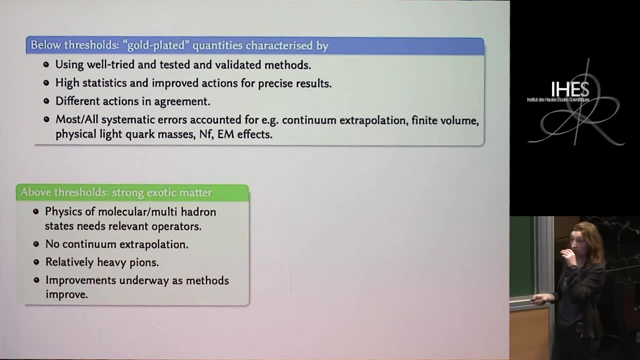 the pion mass, Because, again, you can dial this number up and down in your simulation if you want to. Okay, so what can we actually do? So this is a little bit maybe, towards your question, So you can think about lattice calculations in maybe three different boxes. so here's two of them. 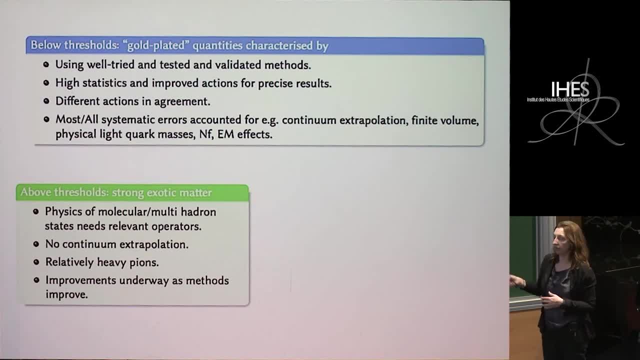 at least So below thresholds, strong decay thresholds. everything behaves nicely. you have bound states. you can use well-tried, well-tested. everything works very nicely typically. you have high statistics, Highly improved actions. everything is very precise. you get rid of all of the systematic. 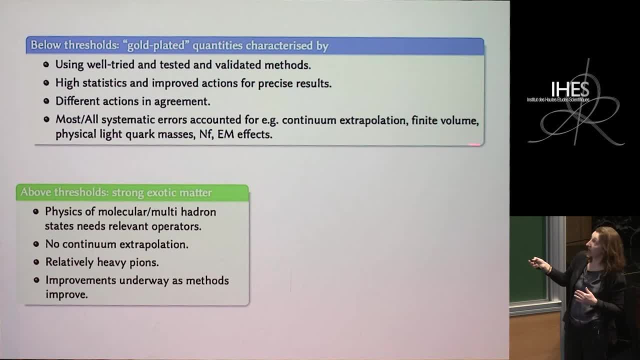 uncertainties. you take continuum extrapolations, you take volume extrapolations, you work at physical light quarters, you sort of take care of everything. So this really is- these are, as I said, the gold-plated things- and even to the extent these days where you can include QED, really put. 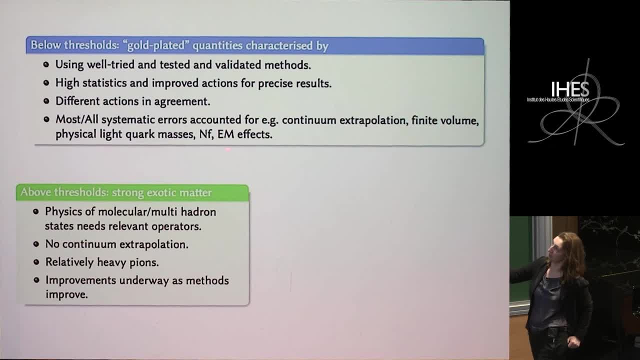 QED and non-compact QED in the simulation as well. Above thresholds, then life is a little bit more complicated, of course, So here's a little bit more complicated, of course, so here's a little bit more complex. so here's a. 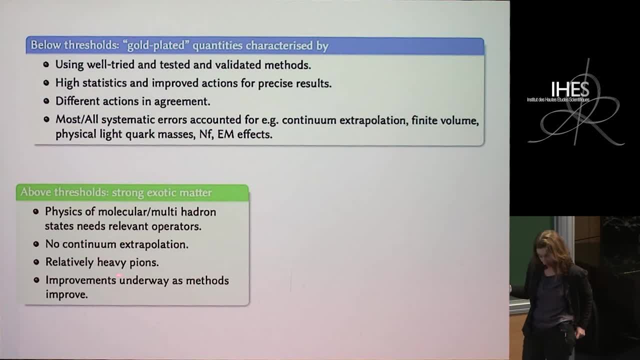 little bit more complicated, of course. so here we need to have many more sophisticated and different operators than we've had in the past, and there's been some developments there. Typically, this is sort of a little bit like seat of the pants stuff. you're trying things out. 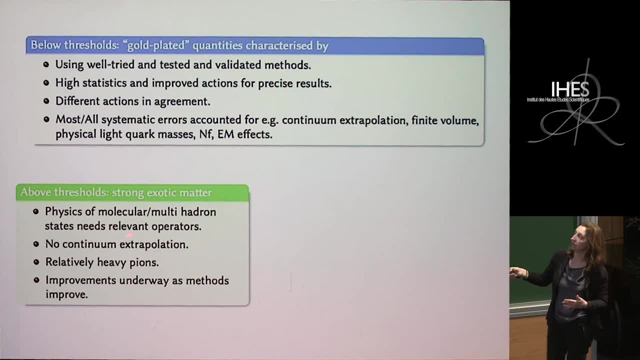 you're trying to understand new methods and how they work, to get you to understand, so that you can understand resonance physics. Typically there's no continuum extrapolation. everything is done with non-physical, unphysical, pion masses and of course you try to make 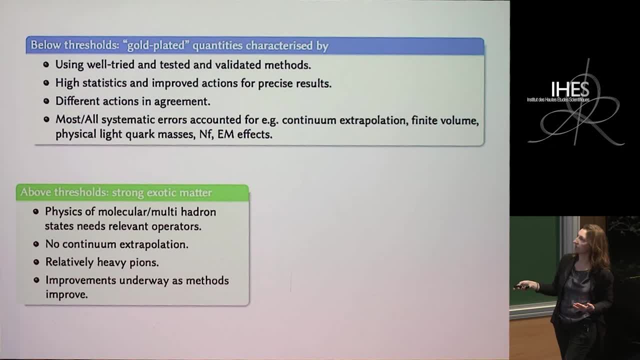 things more complex. So, like if you're here in the Middle East, you can't really do that. you don't really know what's going on here, but you can't really predict the speed of the temperature. So you try to understand the speed of the temperature. 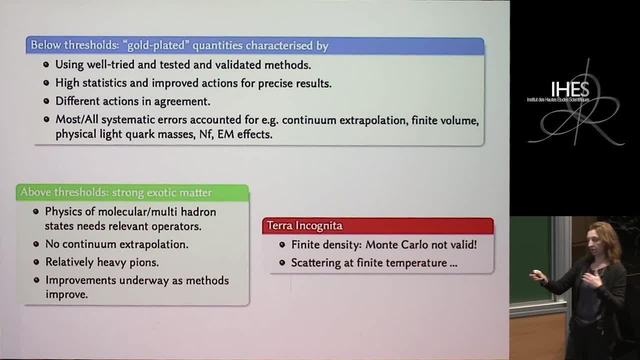 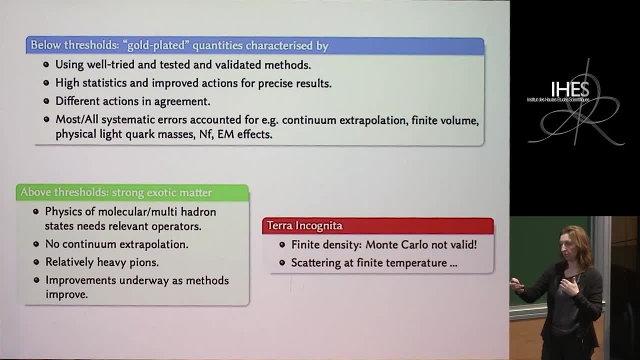 these calculations, but they're rather different to what's going on here. And then there's this piece formulations, so that you identify the temporal direction with the temperature and so you change the temperature by squeezing the box, essentially, and understanding how you do. scattering in that scenario is again terra incognita. 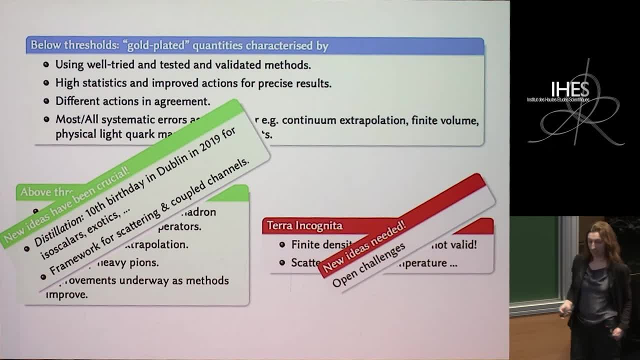 So here new ideas that we've already had in some sense. so new ideas have proved absolutely crucial here. so making progress in the threshold in resonance physics has not been because the computers have got better or bigger or faster. it's because we have much better algorithms that actually are tuned to. 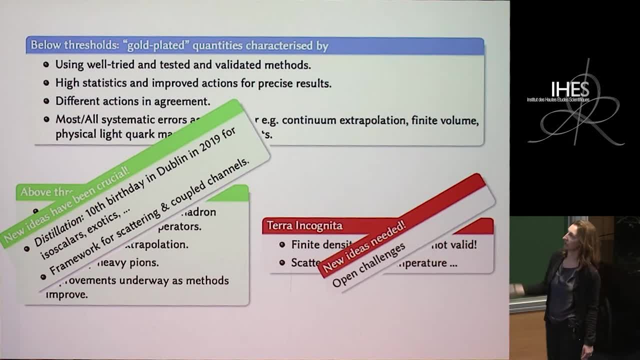 allow us to do these sorts of calculations. So distillation is a beautiful example. so this had its 10th birthday in Dublin. it was invented in Dublin, so we celebrated it last year. it gave access to a whole range of exotic physics that hadn't previously been accessible and set up this whole field. 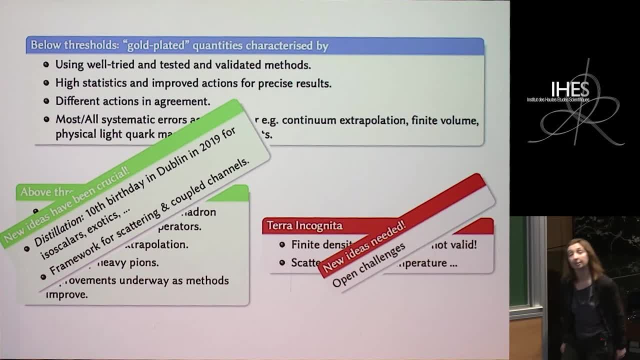 of scattering physics in lattice calculations, The temperature is very important. what's the- I mean the real temperature- which are necessary in QCD? what's what it is like 20 Kelvin? Oh well, the. so the phase transition is at about? it's about 157 MeV. so I, yeah, yeah. 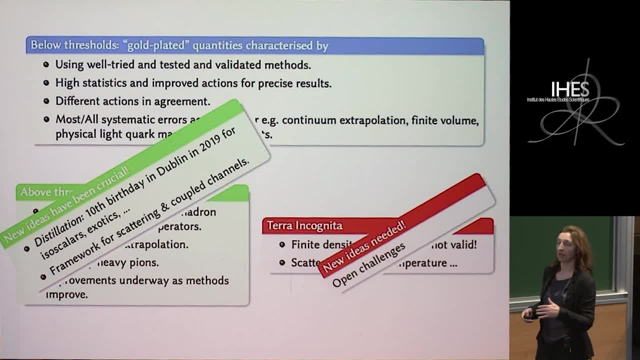 so. so we can go from- essentially it's not quite zero but close to zero temperature all the way up past the phase transition and to maybe about 2 TC. in these calculations It's 10 to the 10th degree. Yeah well, one EV is 10 to the 4th degree, and then you know. so this is cosmological temperatures to every unit. 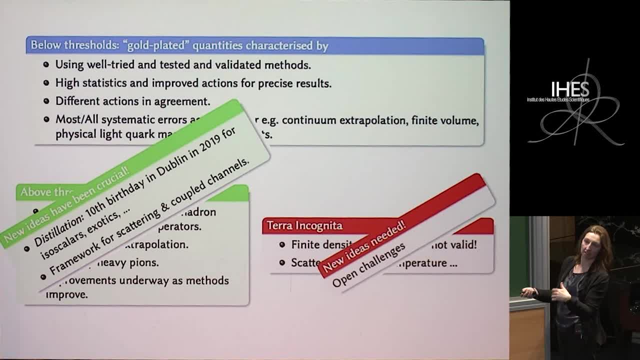 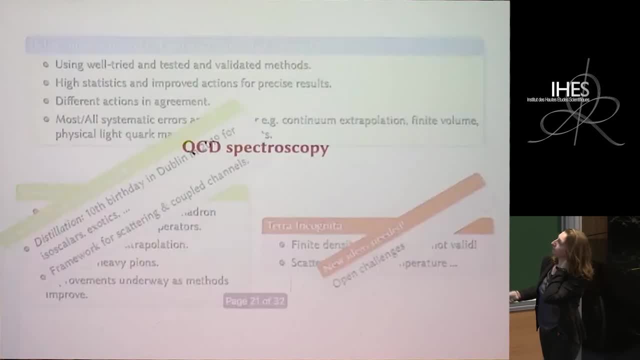 Yes, well, yeah, I mean- these are the calculations- that most of the calculations I'm talking about are at low temperature, so they're well below that transition temperature, but then as you go up, that's right. Okay, so let me show you some spectroscopy then. so these are. 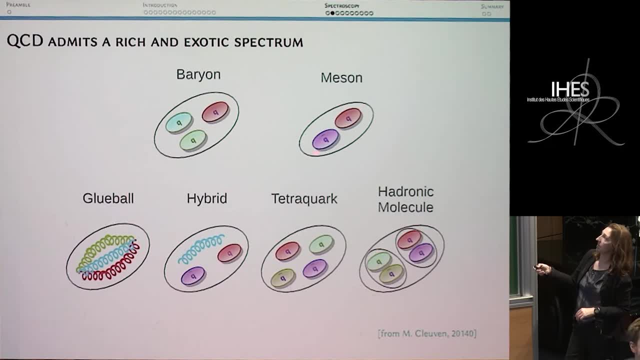 the familiar things that you would want to talk about. so there are mesons and baryons built from quartz, So you can build quarks and anti-quarks in the usual way, but QCD of course doesn't isn't restricted to these combinations, so you can build hydronic objects observables. 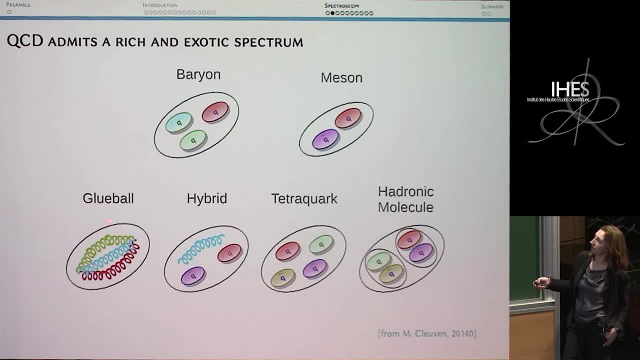 in many different ways, including from glue balls, from gluons, gluon fields. only you can have combinations of quarks and anti-quarks with excited glue. so these are hybrids, tetra-quark objects and molecular objects, where you have these tightly bound structures within some sort of looser molecular object. 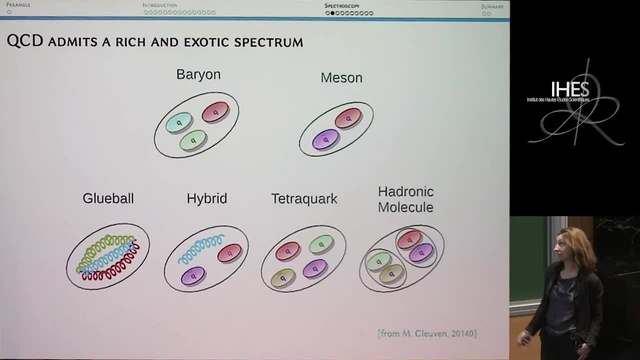 I'm going to click on that. Okay, I'm sure there's a joke in there somewhere. but yeah, they do actually. yes, They have the same effect Maybe. yes, well, you'll have to tell me that. I obviously can't comment on that. 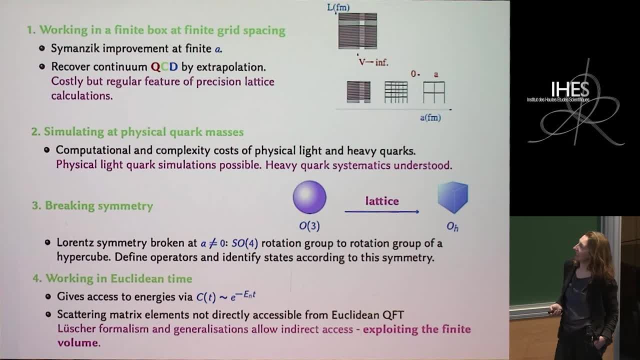 Okay, so now this is a little bit technical as well, but just to give you a sense of the things that you have to think about again in these lattice calculations. so you know, of course we work in a finite box, at a finite grid spacing, so so somehow, sorry. 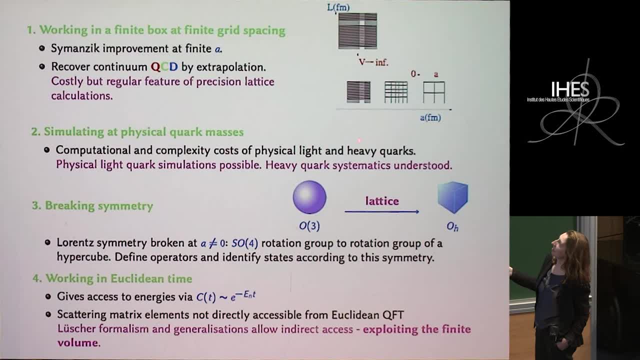 these the graphics have come out a little bit funny, but this is the picture that you should think about. so if you wanted to reach the continuum, then you need to understand how you relate, how you change the box size. so you go in, for example, from a rather coarse lattice to finer and finer, but then you also want. 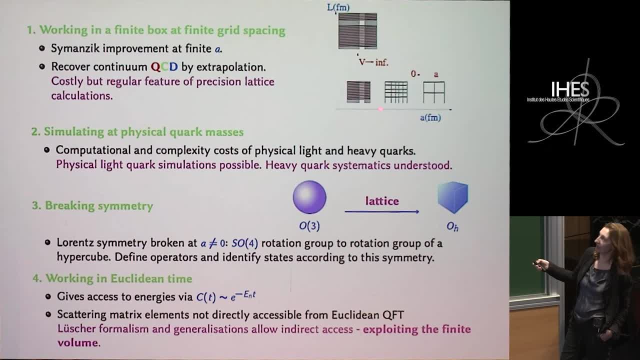 to take an infinite volume limit where you keep the lattice spacing, the grid size the same, but you increase the box size. So those are the two limits, Okay, The limits, the relevant limits. one can sit at finite values of the lattice spacing and use, for example, semantic improvement procedures to reduce the size of the discretization uncertainty. 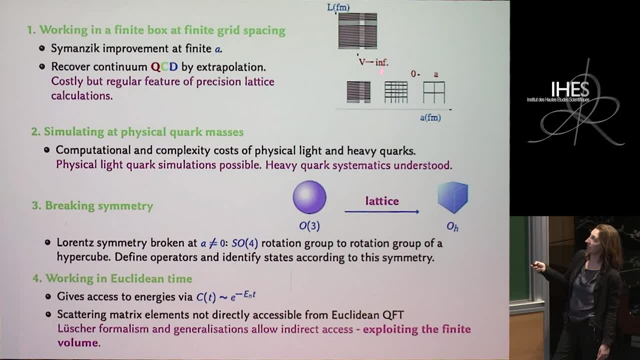 by introducing irrelevant operators at finite lattice spacing, and that's again a well well trodden path in these lattice calculations. but ultimately you want to demonstrate that you can take this continuum limit, So of course it means that you have to repeat the calculation many times. 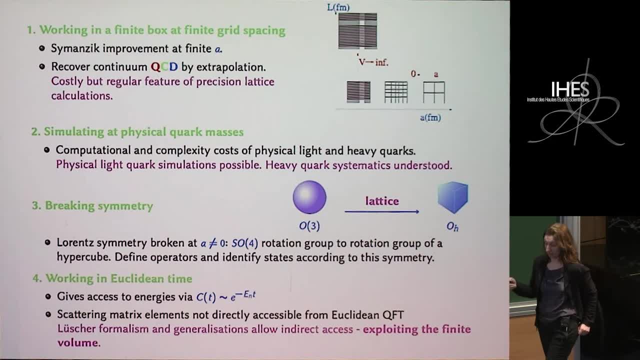 But it's necessary for these precision physics that I talked about a little bit. Okay, so maybe more interestingly, you can, you need, would like to simulate at the physically relevant quark masses. this comes at a computational cost, so I mentioned, at least alluded to the light quark cost where the light quarks appear. 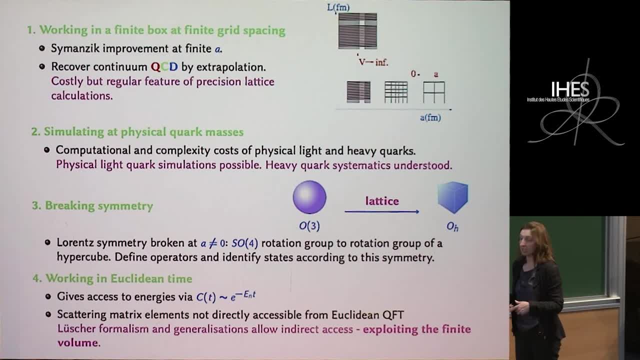 in the fermion determinant and so, in fact, the condition number you have to invert that matrix, and the condition number of that matrix scales with the, the light quark mass. So as you reduce the light quark mass, the condition number of the matrix that you're 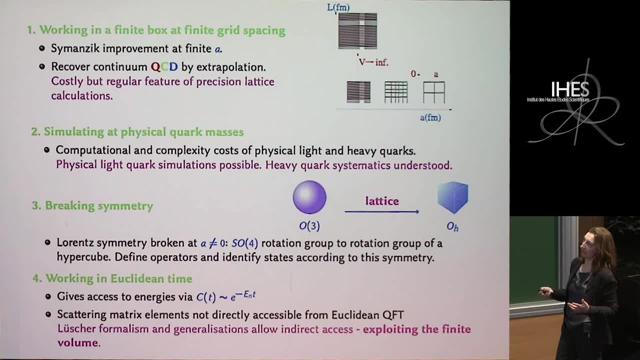 trying to invert gets larger and larger and quickly becomes a very difficult problem. So that's an algorithmic issue with light quark simulations For heavy quarks. those heavy quarks have a scale again with a, have discretization uncertainties that are proportional to the lattice spacing. that's true in the light quark sector too. 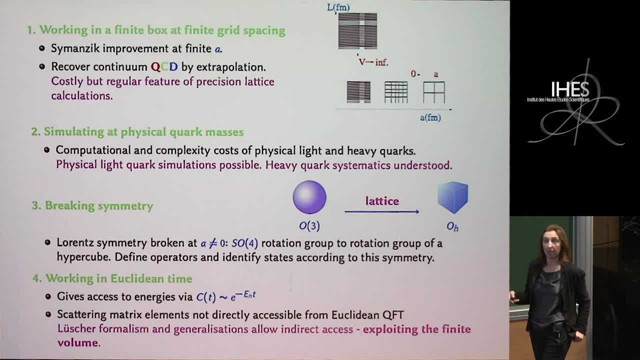 but a times a small number is not so bad, but a times a big number, if it's a bottom quark, is a problem, And so you have to quickly swamp your calculations. so you have to understand the heavy quark systematics, which is often done through effective field theory methods like non relativistic. 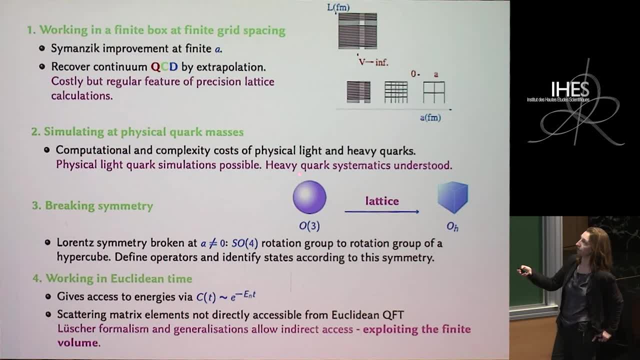 QCD or even static approximations, for example. The last relevant point here: I've already talked about the working in Euclidean time, but the Lorentz symmetry is of course broken at finite lattice spacing. so that means that the relevant symmetry group to classify, for example, hydronic objects in terms of the irreducible 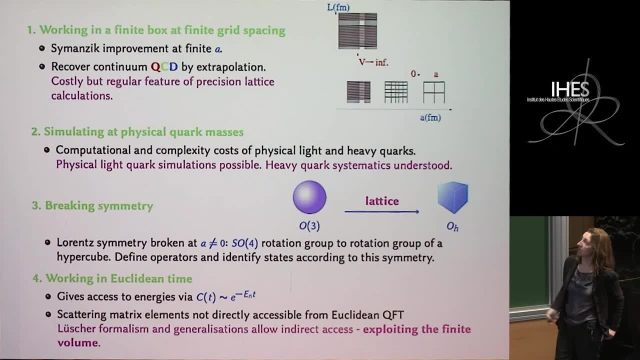 representations is not the continuum group. It's the continuum group But instead is the symmetry group of the cube, so OH or O3, and we have to define operators and identify states according to the symmetry group of the cube rather than the symmetry group of the continuum. and then there's a piece of work that allows you that you have 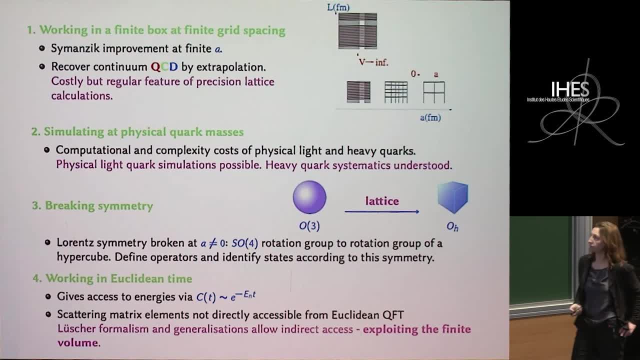 to do to understand how to go from here back to here. essentially, So again, if you essentially, the problem here is that here you have an infinite tower of spin values Which correspond to the irreducible representations of this continuum group, but the cubic group has five irreducible representations. and so all of those spin values, all of the J values, 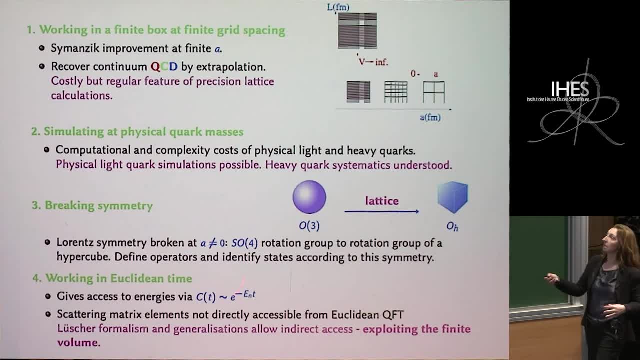 are mapped onto the five irreducible representations that characterize this symmetry group, and so you have to understand how to disentangle all of those degeneracies so that you can relate a state on the lattice to a state in the continuum. so it can be tricky. 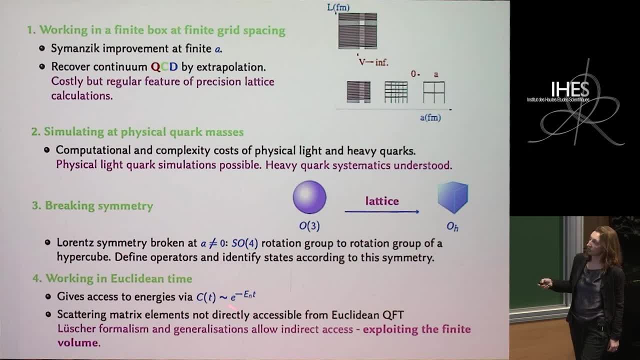 And then this: I already said: we're working in Euclidean time, So that we have this positive definite weight and can do these Monte Carlo calculations. and this also gives you access, allows you to write the correlation function as this sums of exponentials, but it also means that you lose direct access to scattering matrix. 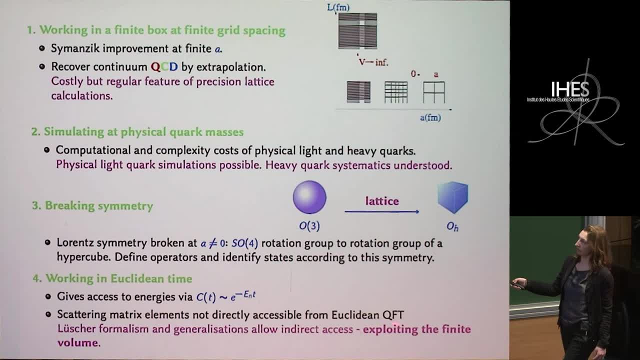 elements in a Euclidean field theory. so this is, of course, well known. but there is an indirect approach to this now through the work by Luscher and others that followed. But this is only if you, if you're gauge fixing right, but this is a gauge invariant. 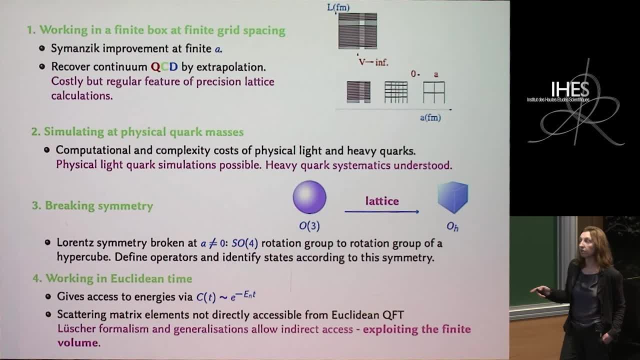 theory, so you don't need to gauge fix. no, no, so you only need to gauge fix if, for example, you're interested in the gluon propagator. if you're interested in the gluon propagator, then you have to gauge fix. and there you have to be careful about Griebov copies, for example. 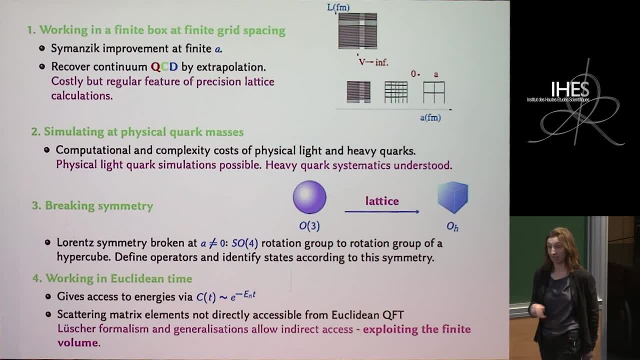 in fact. so one of my thesis projects was on an algorithm to specifically avoid these Griebov copies in gate lines. So if you're doing that, then you have to gauge fix. yes, so for gluon propagators, for things like that, then yes, indeed, you have to gauge fix. but typically all of this is 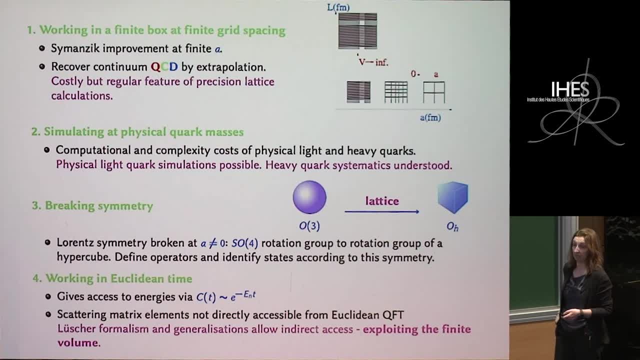 gauge invariant right, and so when it's gauging very, you don't need to worry about that. You have to sound for all the possible U configurations. Yes, And there's a huge redundancy. so how do you avoid summing over the same things? 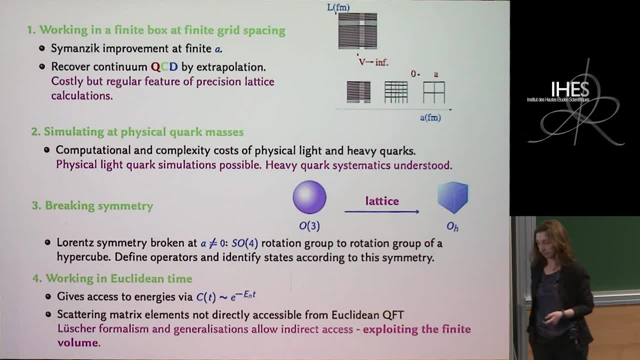 Maybe. so say that again, sorry, I don't Like. given configurations of U's, maybe gauge equivalent to another configuration of U's. We are over counting. The volume of the gauge group is a factor, So you're summing over U's right over all the possible link variables. 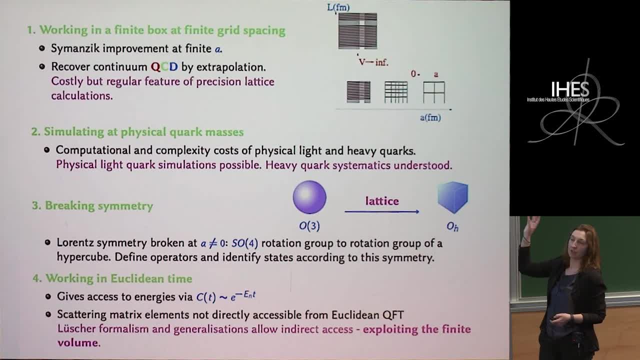 But the space of link variables has a huge redundancy. Yeah, no, no, but you. but you're stochastically sampling. so, But maybe, Yes, The power of sampling, it doesn't matter, right, Yeah, The partition function factorizes out. it doesn't matter. 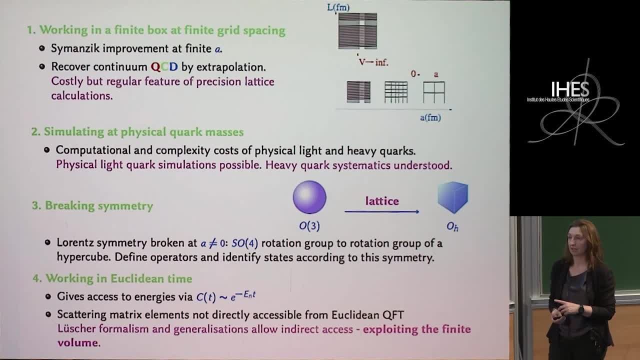 Right, so you can maybe cut out a huge number of things that you're over counting. Maybe you're Well, but I mean so, yeah, Maybe you want to only sample over gauge non-equivalent link configurations? no, Probably, when they divide them by partition. 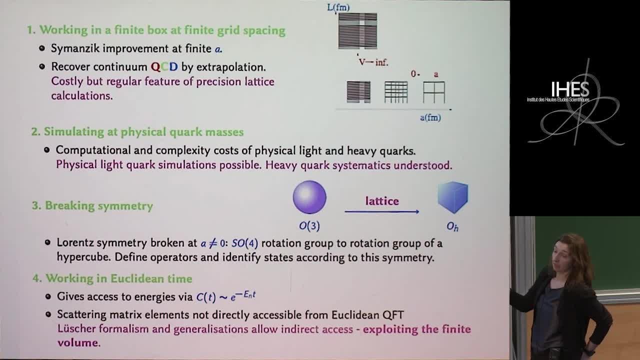 Yeah, but it, it, yeah. so They divide by partition factor, right, Yeah, yeah, But I think it's a. I'm not quite sure it's the same problem, because in the Monte Carlo calculation You're not quite summing over all the gauge link configurations. 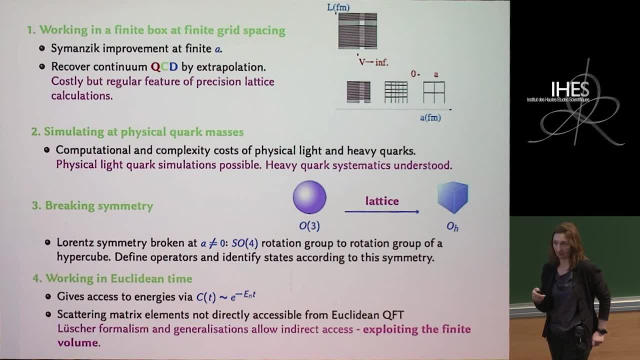 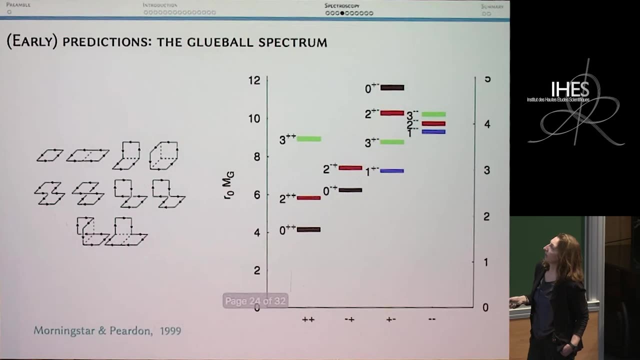 It's weighted, don't forget, with a probability distribution. So you're sampling from that weighted set of link variables. So I think it's probably not quite the same, but I'm not. yeah, I'm not sure. Okay, Well, actually Gregory mentioned glue balls, so I left. I'm glad I left this in. 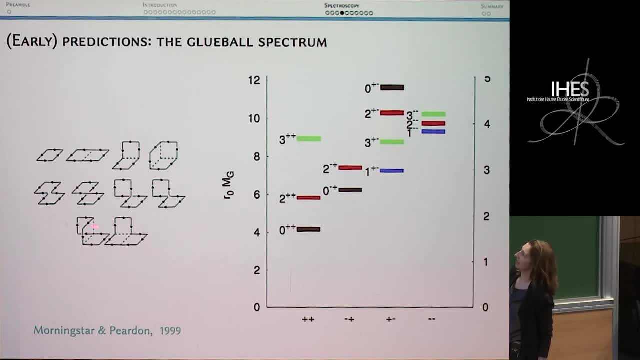 But anyway. so this is an early success of all of these lattice ideas. So here are lots of different operators in this Young-Mills theory And you see, indeed, that you can extract these very nice spectrum of states. This is from a very long time ago now. 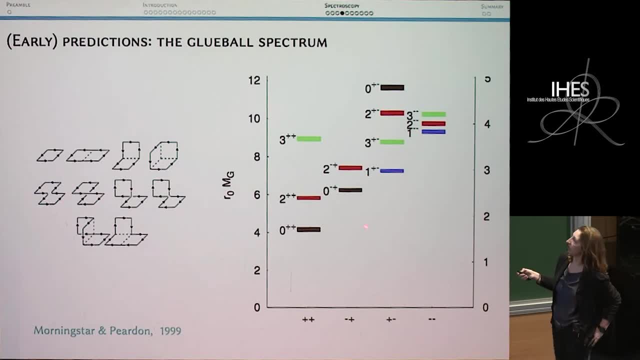 This is actually even a quench calculation, So it's quite ancient history, but still somehow relevant. This is before man came to the trinity. Yes, Yeah, yeah, yeah, Yeah. This I won't dwell on because it hasn't come out very well. 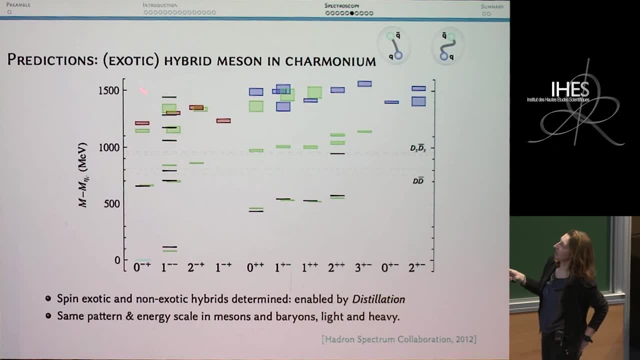 So let me show you this one instead. So this is a more recent work where we can then determine what an exotic meson might look like. This is with CC bar contents or Charmonium states. So here's a regular CC bar And here is a sort of a cartoon of a hybrid, where you have some excited gluonic content in the between the Q and the Q bar. 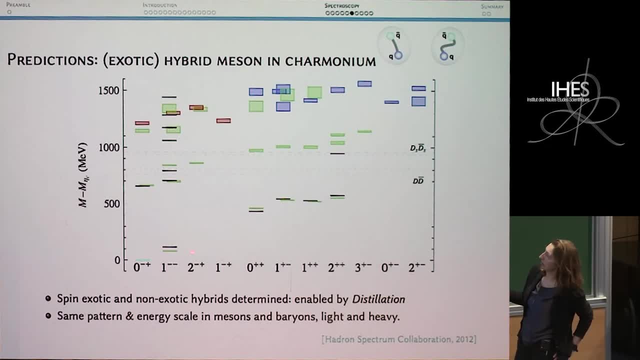 And so what you see here is a rather busy plot. But first of all The black lines are what we know experimentally. So you see that you know some things experimentally, But actually you don't know very much experimentally. And then the rest are the results of lattice calculations. 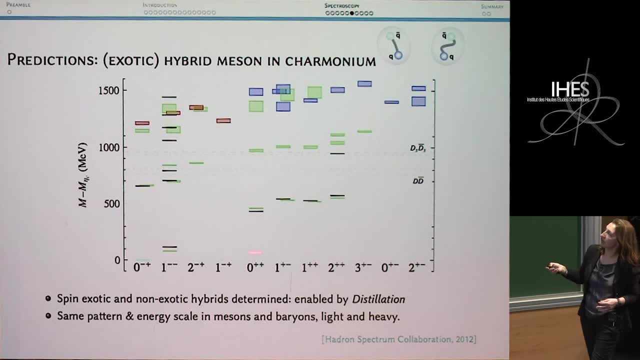 So the green boxes are simple QQ bar type objects And then the colored in either red or in blue are states that we identify as hybrids. So these states that appear, if you again, if you know your QCD nomenclature, You'll see that these are. 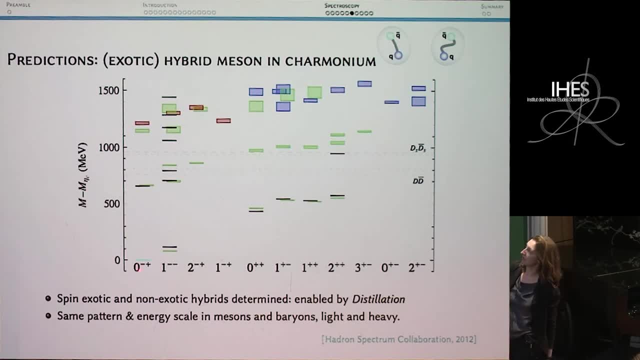 Regular quark model states with JPC values, But also an explicitly exotic channel, which is this one minus plus and is not allowed in quark models But is allowed by QCD, for example. So you can calculate what a state would look like in that particular exotic channel. 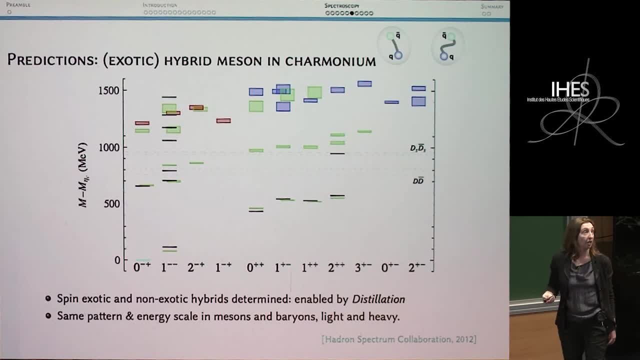 And you see that there's a plethora of these things which you can calculate in the lattice, Which await some experimental input now to understand whether they're real or what the values of these things are, Or indeed what the structure of them is. Again, there are some faded lines here which are indicating the thresholds. 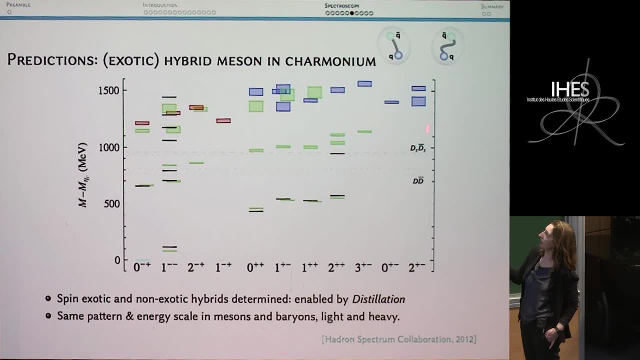 The thresholds for strong decay in charmonium to DD bar type states. But in this sort of naive approach we've treated everything as a bound state. So here are some current challenges. Yep, nearly done So if I wanted to go beyond, so here let me just again just say: 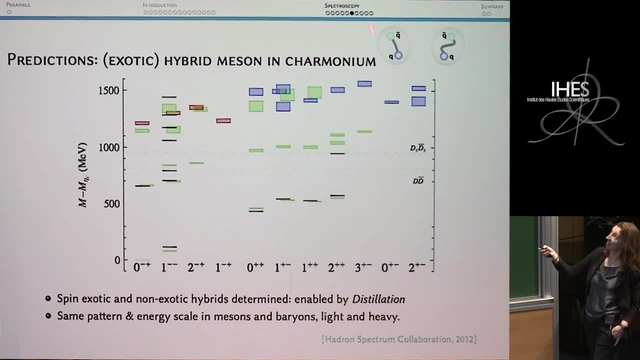 So everything here is the assumption is it looks like this. So it is sort of QQ bar In some bound state configuration like this. You might put some exotic things in between the Q and Q bar, But I don't worry about the fact that I'm sitting above decay thresholds. 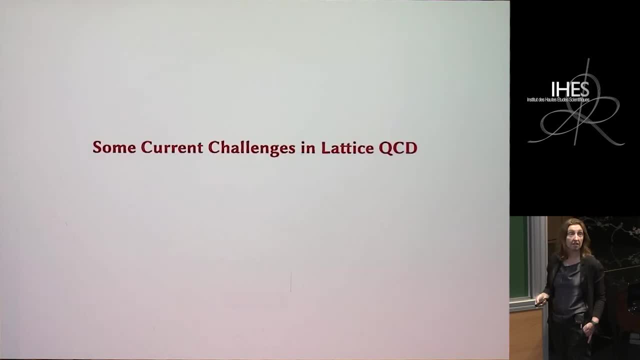 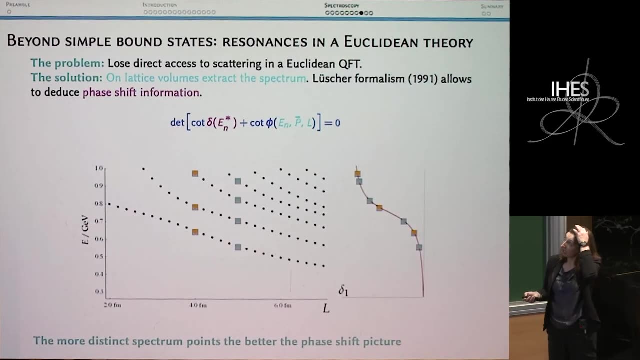 Or I don't allow that to affect the calculation. Of course, that's not actually reasonable. Everything is more or less. all states are resonances, And so what we need to understand is how to calculate these spectroscopy: The spectroscopy in the presence of or allowing for, resonances, and scattering states. 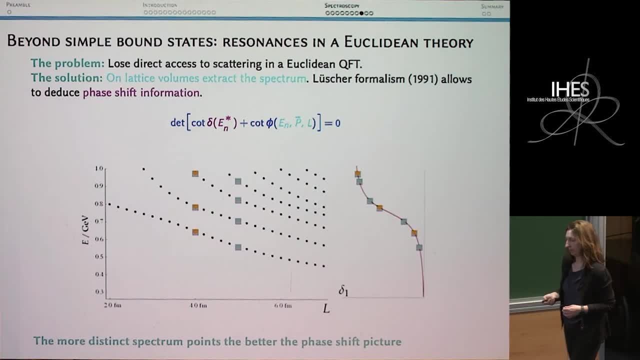 And I mentioned previously That this Euclidean theory, essentially you lose access directly to the scattering matrix element, And so the solution to this is in fact found initially by Lucia. It was written down in 1991.. There was earlier work by others in non relativistic quark models, for example. 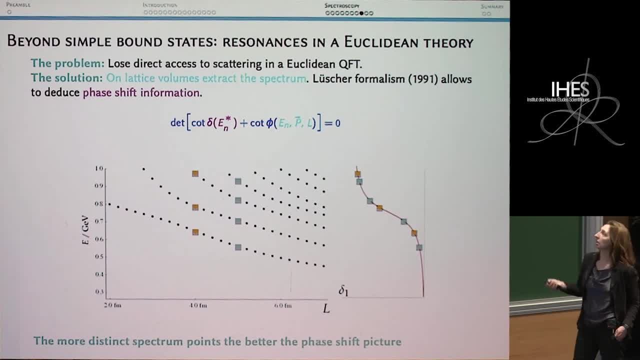 But Lucia was the first to formulate this, at least for a QCD application. And so what he? what he showed Is that you can relate, You can turn the fact that you live in this finite box, With the discrete spectrum of energy levels, to your advantage. 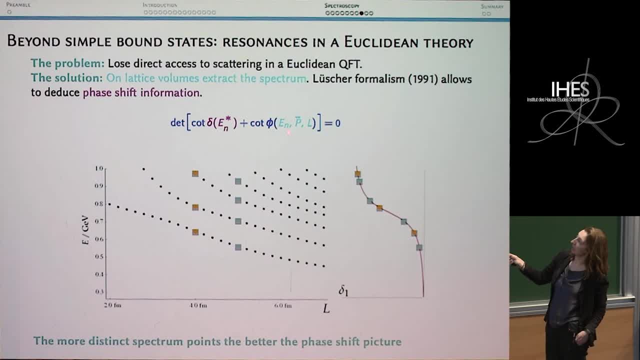 And relate the information that you extract in a lattice calculation, Which are essentially these energy levels at some particular box size L, or momenta P, Where that's the overall momentum of the system. You can relate that to phase information, The phase shift in infinite volume. 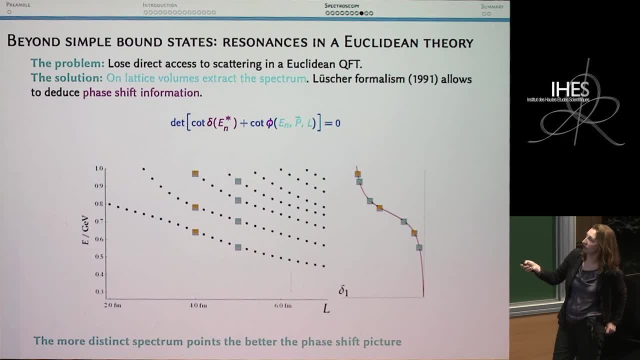 So this relationship, This relationship is through this function, phi, Which is some generalized zeta function Which you wrote down. Practically what that means is that you calculate lots of energy levels, So lots of these energy levels at lots of different values of L. 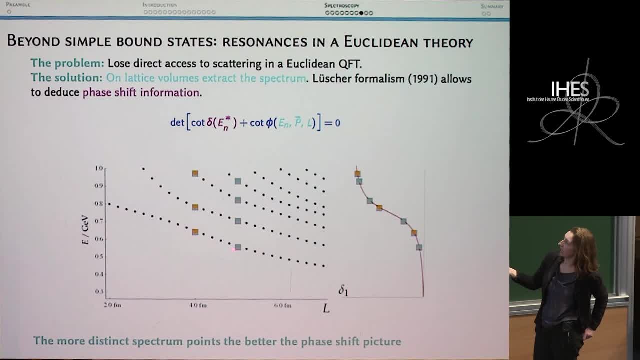 And the more points you have. You use this formula then to allow you to translate from these energy levels to the phase shift, And so you see that the more points that you have in this calculation, The more points you have in this phase shift. 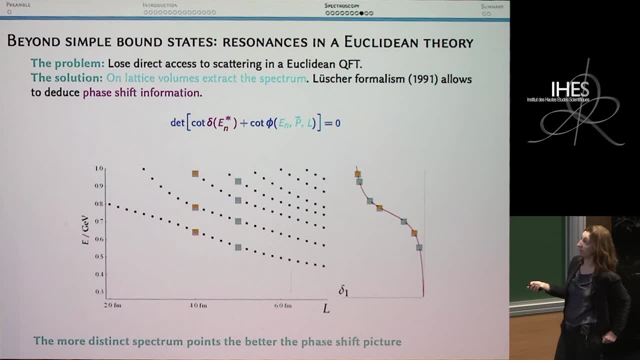 And so you map it out much more cleanly. So that's the basic idea. You might wonder why it's taken so long to actually do this. So from 1991 nobody did anything for a very long time. So people tried at the beginning in the early 90s, to do something. 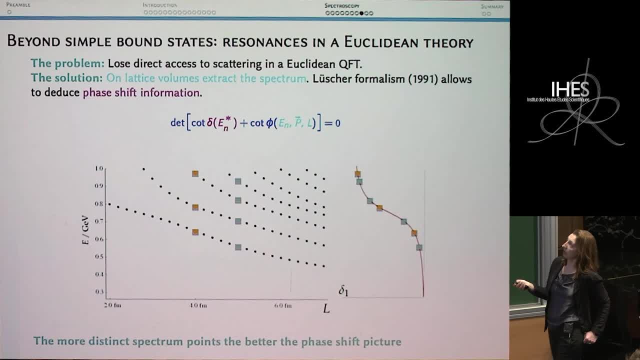 And it didn't work at all, And then nothing happened until about 10 years ago. And so, about 10 years ago, this distillation algorithm actually opened the door to this By allowing the determination of these energy levels in a very precise And rather beautiful way. 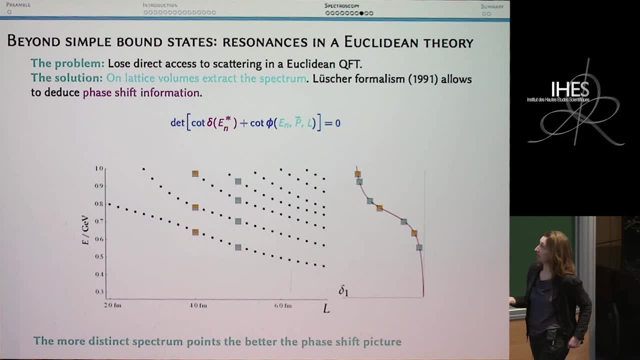 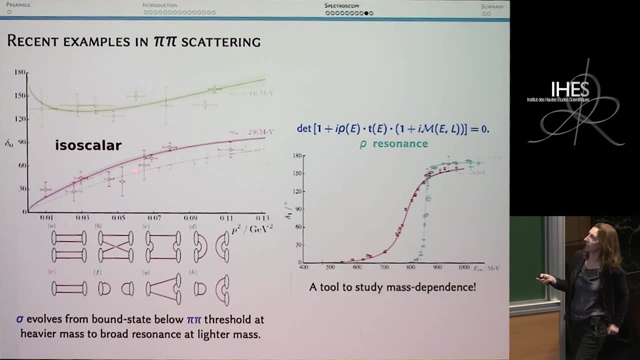 Which meant that you could finally implement this Luscher method. So that's been a real growth area. So there's lots of. I picked two particular examples which are interesting. At least as a lattice person they're interesting. So this is an isoscaler in pi pi scattering. 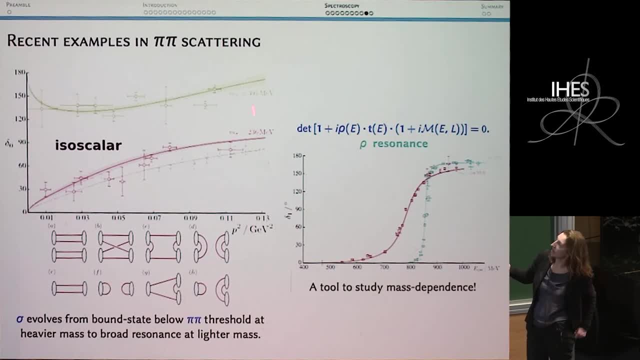 It's a little bit tricky to see here, But again so I apologize. So these are two different quark masses. So remember that we have complete freedom to dial the quark mass up and down, And what you see here is that. So this is the heavier quark mass. 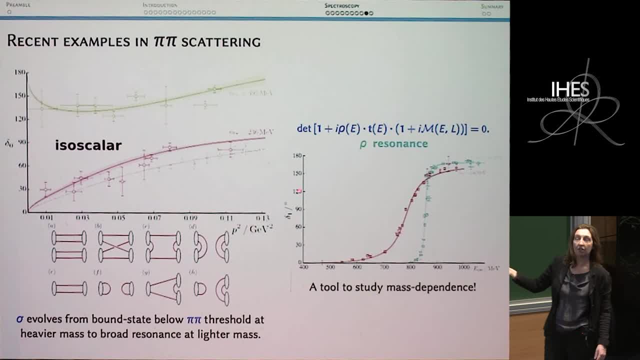 And this is the lighter quark mass. You see rather different behavior for this particular state Depending on the quark mass. So we see this is the sigma. It evolves from some bound state to a resonance at lighter masses. So this is what these pictures are showing you. 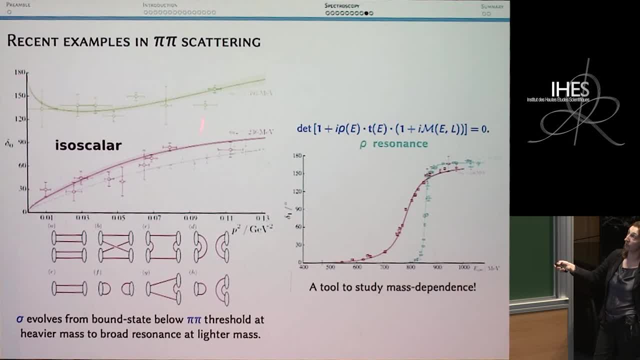 But you see that you can understand some of the resonance physics By just changing the quark mass in a very nice way, And these are some of the wick contractions that you have to do, But that's less interesting perhaps. So here is the row: resonance. 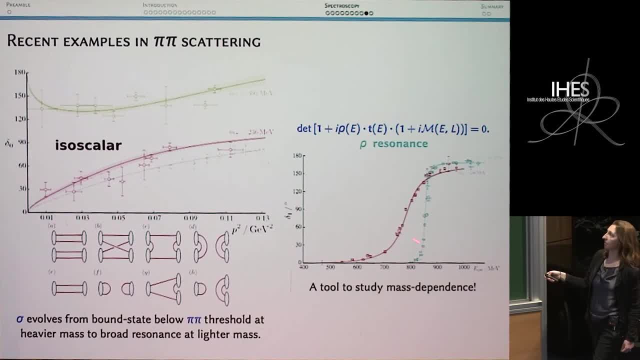 Something that everybody has seen, hopefully, before. This is a very well determined thing, experimentally, of course, And here again you see the effect of different quark masses, So you can change the quark mass And see the row resonance really appear in the calculation. 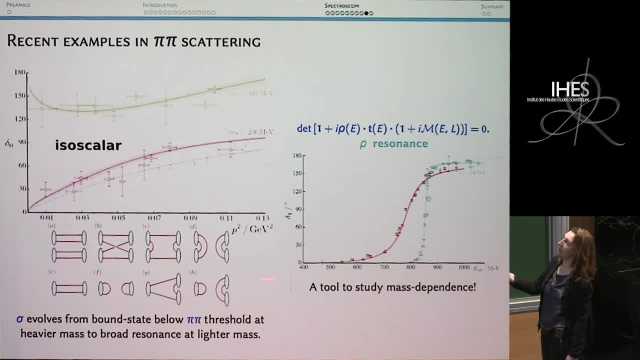 So of course this is interesting to see when you know the answer. It's even more interesting when you don't really know what's happening, To see how the resonance behavior depends as a function of the quark mass When you change the quark masses. 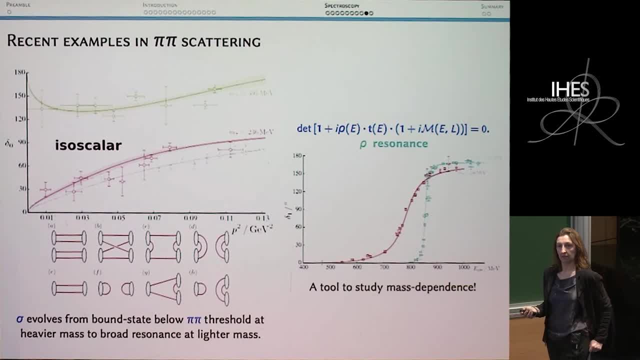 You keep the condensate value constant or you also move. that, Yeah, so that also moves. No, sorry, Yes, it does, It also moves, Although it doesn't play. I'm not sure what role it would play here. 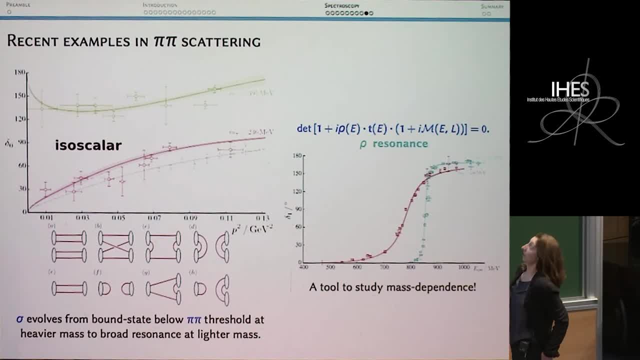 Well, in the row, it will play. In proton it will play even more. so Yeah, Yeah, I'm not sure. So it definitely changes, But I'm not sure it's been tracked in any systematic way. The condensate itself hasn't been tracked. 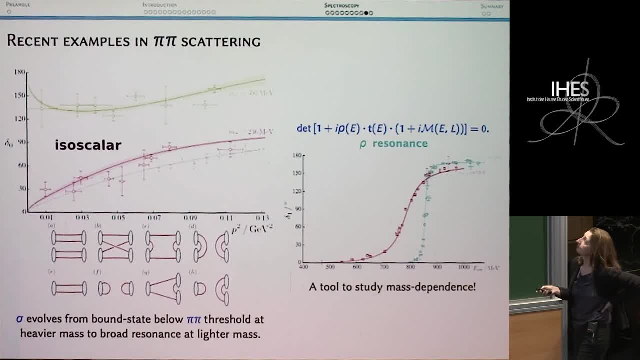 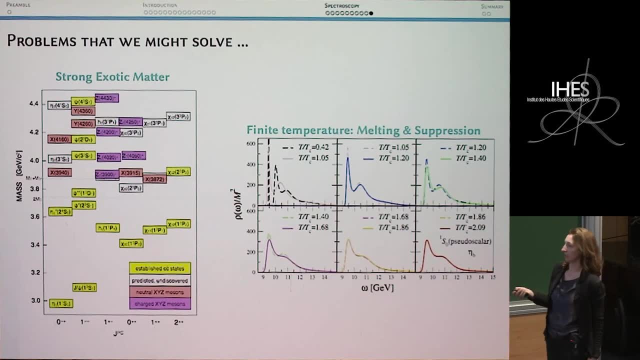 No, it's a good point actually. Okay, so let me just finish, then, with things that we might do, And then, finally, things that are more speculative. So here's something that I think is reasonable to imagine doing, Given the slide that I just showed you, where we can understand how to do scattering. 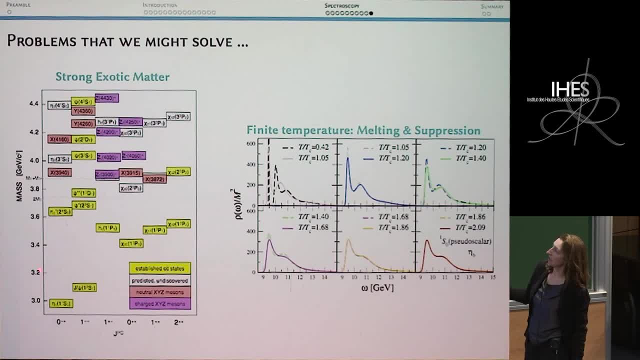 This is nothing to do with the lattice calculation. This is the set of experimentally measured Or expected masses in the Charmonium system, Which it is assumed is reasonably well understood, through potential models, for example. And so the different colours are: The yellow are things that are established and measured. 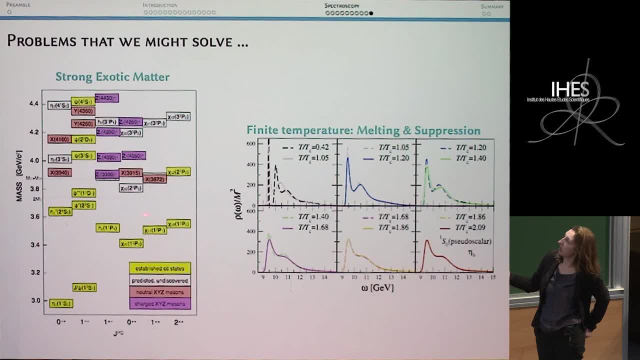 Predicted by theory and measured. White boxes are those which have been predicted in some quark model calculations but aren't discovered yet, And everything else is new, undiscovered, unexpected and to some extent possibly unwanted. So these were discovered in experiments from about 2003 onwards. By Bell, then Best, then LHC. They are sitting above strong decay thresholds. It's completely unclear what they are, So one might imagine that they could be some molecular states. Even some tetra-quark states are postulated, But interestingly, most of them are also extremely narrow. Which would mean that they're not necessarily a loose sort of conglomerate, A sort of conglomeration of di-quarks, for example, But rather have some much more tightly bound structure. That is not what you might expect above the decay thresholds. 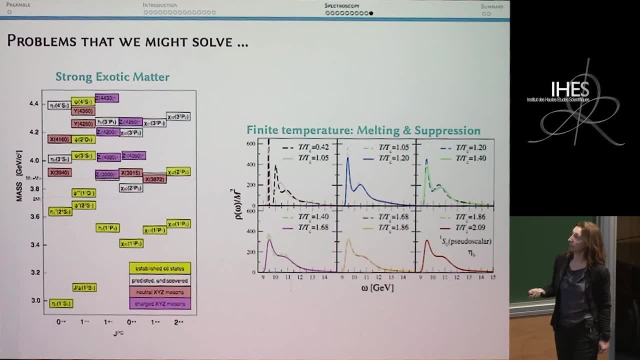 So this is completely unknown, At least at the moment. We don't understand what these states are. This is a perfect place for a lattice calculation to actually make some progress To understand what these are, And these are a finite temperature calculation. So here, what we looked at was the Bottimonium spectrum. 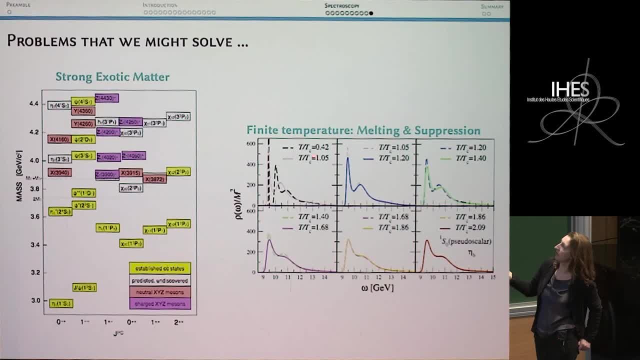 So BB bar spectrum as you dial up the temperature. So this is T over TC And you can see in each pane as you move from left to right and top to bottom, The temperature is increasing. from T over TC is about 0.4 to 1.. 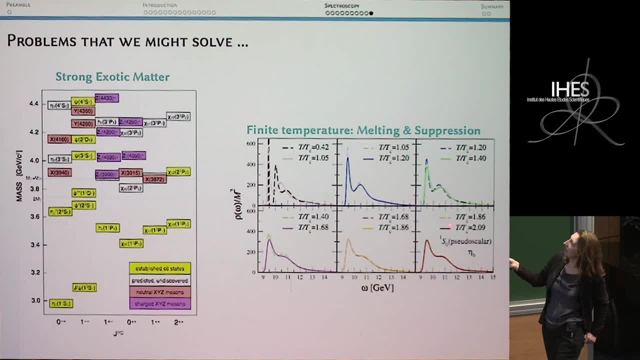 And then up to higher and higher values of TC Until you have T over. TC is about 2.. And you see that the main points that take away here are: the peak, Which is the ground state, here is shrinking And broadening, Which is commensurate with melting and suppression of the state in the medium. 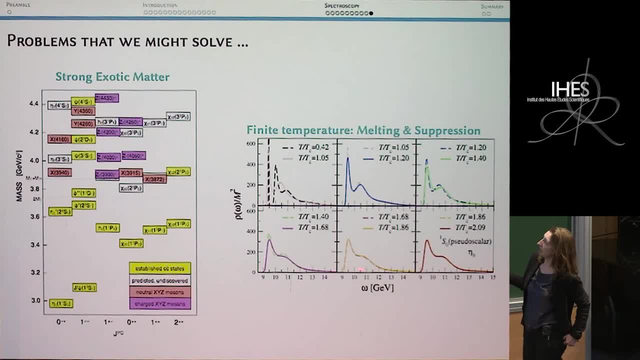 In the quark-gluon plasma. What we don't understand at all is how, for example, such a state might scatter. How do you understand, if this is a resonance, not a bound state, How this behaves in the plasma? So these are completely open questions. 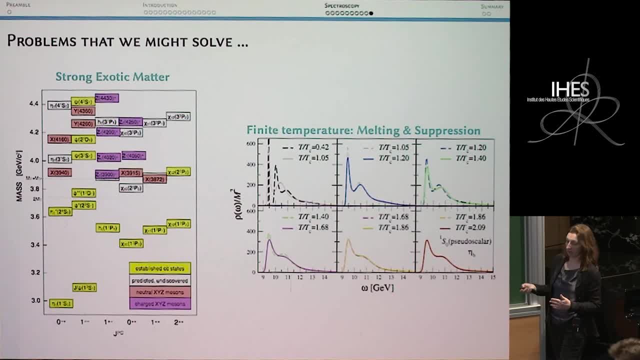 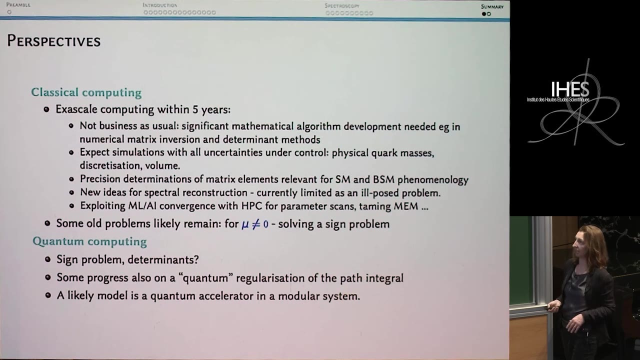 Very interesting questions there are, And a lot of subtleties here about recombination effects from melting And how that feeds into scattering calculations Which, again, are only beginning to be discussed by in a lattice setup. So, since coffee and I didn't know, I'm standing between you and coffee. 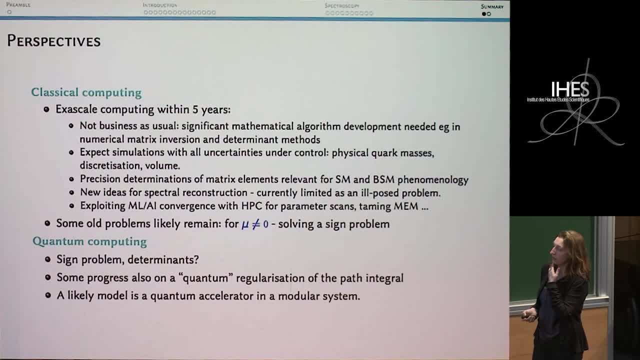 So maybe let me just finish with some perspective. So I split this into along the lines of computing, Because lattice people are always expected to talk about computers. So I thought I would say something about the two sorts of computing that I see on the horizon. 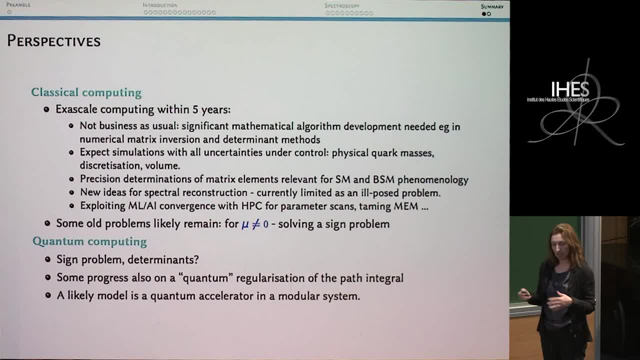 We are sitting somehow at an amazing point where computing is really radically changing, Both classically and in terms of quantum computing. So at a classical level, this exascale computing that we'll see within two years Is absolutely not business as usual, So we cannot just take the code we have. 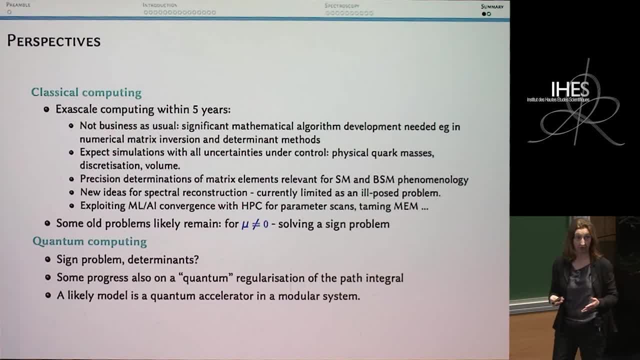 Put it on the big machine and press go. It will not work. Nothing will work. We need new algorithms. The workflows will be different. Everything is going to be very different on these machines, So this is, of course, a huge challenge, But it brings with it many, many exciting possibilities. 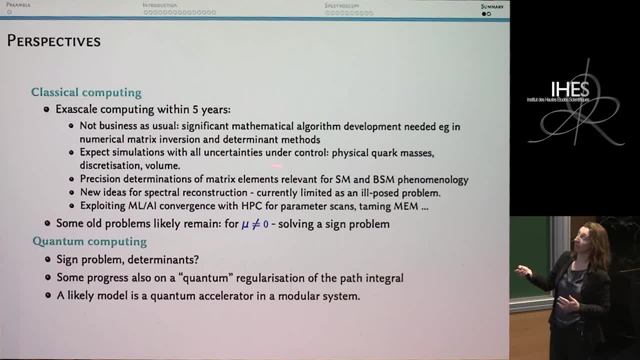 To do, of course, more precision determinations of matrix elements, To calculate matrix elements that we simply cannot do at the moment And to understand, for example, this spectral reconstruction problem That I showed you a little bit in finite temperature just a while ago, Which is currently limited because it's an ill posed problem. 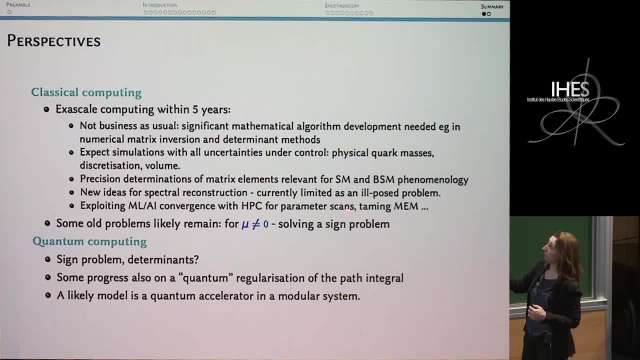 So this is a transformation from How you go from an object where you have a limited number of discrete points To a continuum object, which is the spectral function For these finite temperature states. So all of this is somehow, I think, a really exciting time. 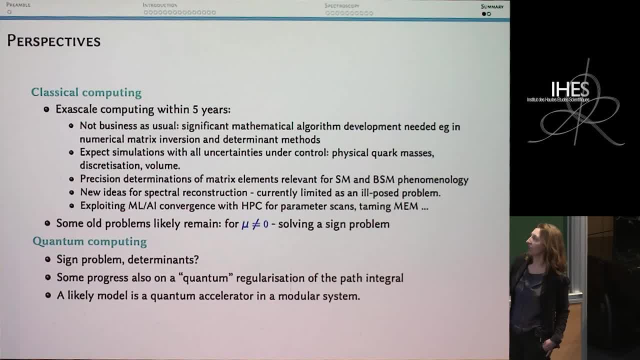 Just from a classical perspective, And since again, everybody always mentions these words these days, So a lot of people, of course, are also using or investigating How we might use machine learning techniques and AI In convergence with all of this HPC business To improve what we're trying to do. 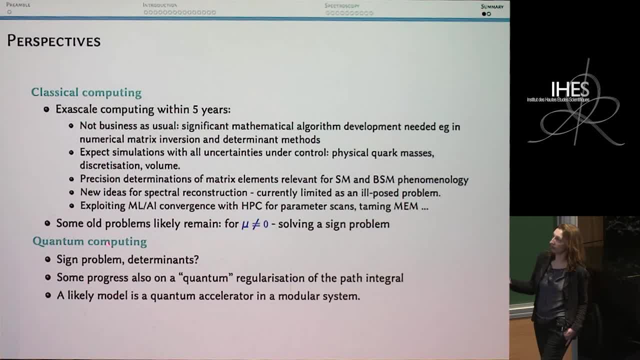 Quantum computing is, of course, a further horizon, But nevertheless an increasing prospect for numerical simulations. No, I know it's yeah. I don't think so. I mean so IBM has a machine now with 53 or something qubits. Google has 70 or so. 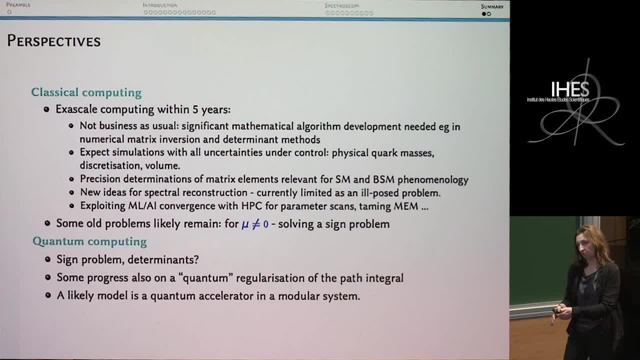 I mean these machines are getting bigger and bigger. There are many really interesting problems to understand. In particular, quantum error correction is a huge problem That I don't think is fully under control yet at all. Reproducibility is a problem. I mean there are many really interesting problems. 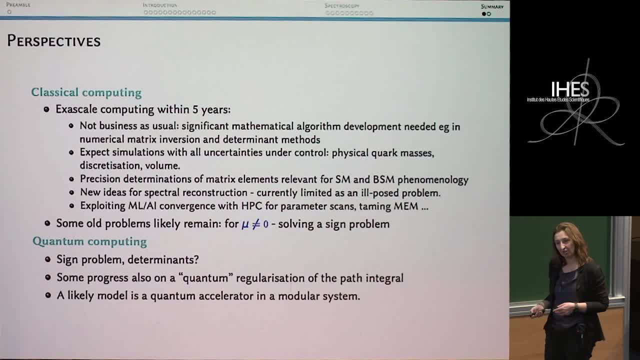 But the possibilities are also very interesting, Because this sign problem, for example, Maybe a very nice problem that you can reimagine In this quantum computing scenario, And in particular we might, for example, make some progress In the Grassman integration, Where those variables would be something that we could imagine. 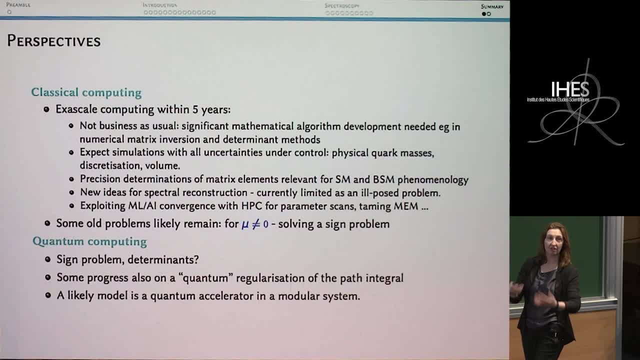 That integration we could imagine doing In a quantum computing way That removes the determinant part. So the determinant came because of the Grassman integration That we did analytically. If we now numerically evaluate these Grassman integrals, Then there's a possibility that we can sort of subvert. 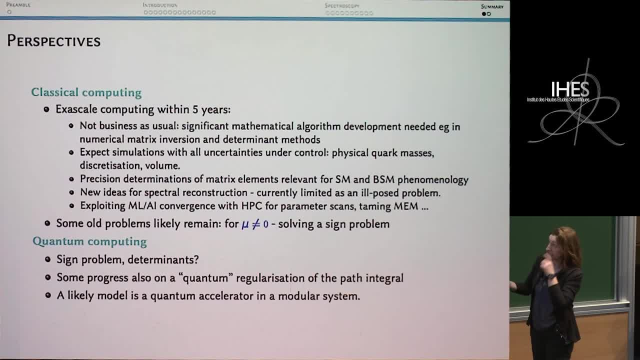 The determinant calculation And therefore understand a little bit more, For example, about the sign problem And indeed how we calculate these determinants as well. So this is a- I mean, this is very speculative, I should say, But it's a real, very interesting question. 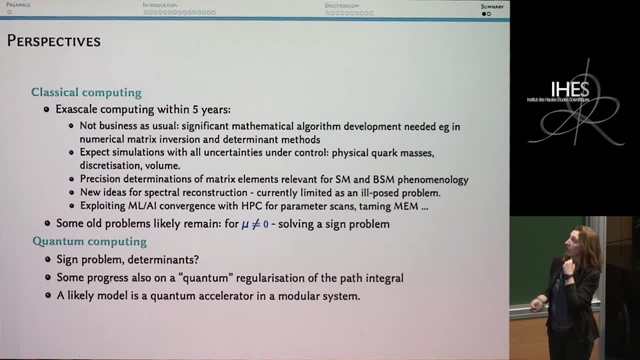 For lattice calculations. There's also been some work on regularization, Alternative regularizations of the path, integral, Using zeta functions, And a very likely model is that you have a quantum accelerator In some sort of classical system, So you send a bit of your calculation off to the quantum computer. 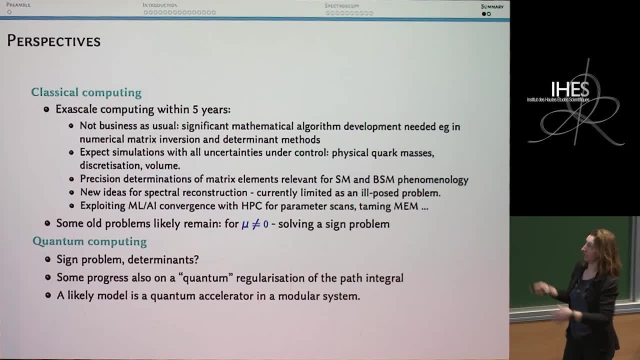 And you wait for it to come back And then you go on and do your classical thing. But, as I said, these are perspectives. I'm not quite sure what's going to happen, So it's very interesting. Okay, last thing, Samson. 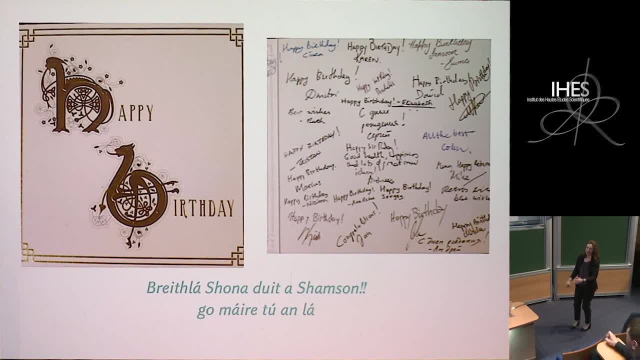 Happy birthday. This is a birthday card That, because I'm so useless, I actually forgot to bring with me, But it is sitting at home on my desk. I did manage to get it scanned, though, So you can see what it looks like. 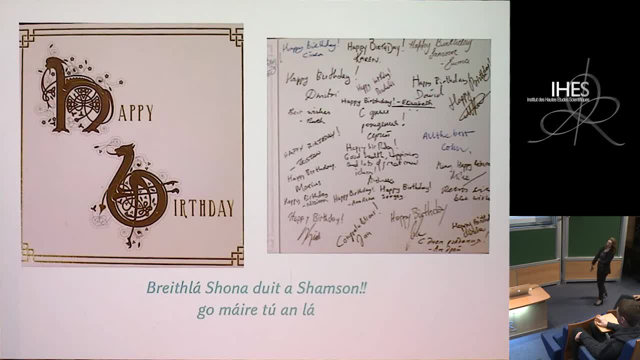 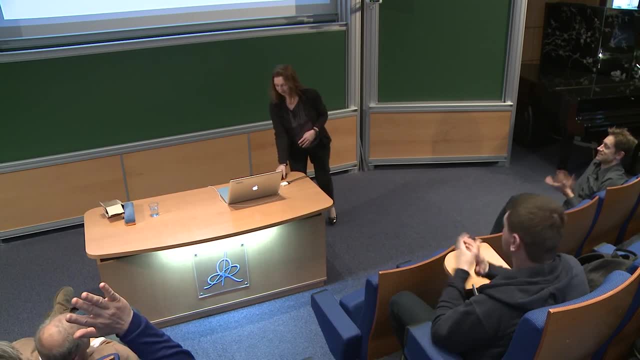 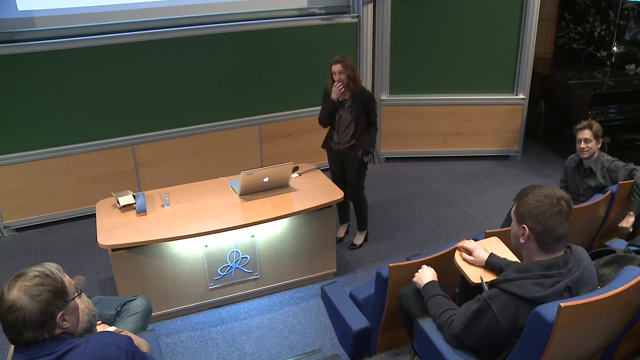 So this is the front of the birthday card And it's been signed by all your colleagues in the school of maths. So happy birthday, Samson. Question. You say Euclidean formulation is difficult to refer to Minkowski. To go back to Minkowski, 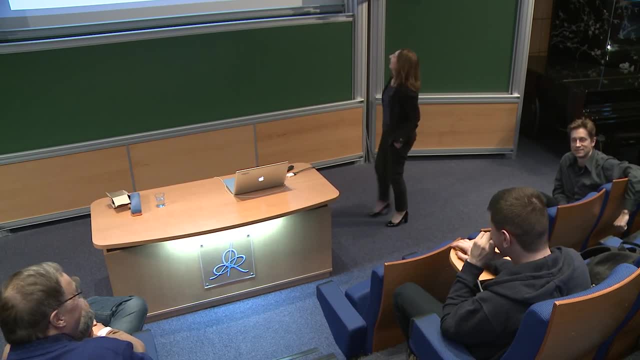 So So we typically, You typically don't. I mean you can No way, right. Well, no, You can formally at least understand how to do it, But numerically not. But you can also argue that you don't need to. 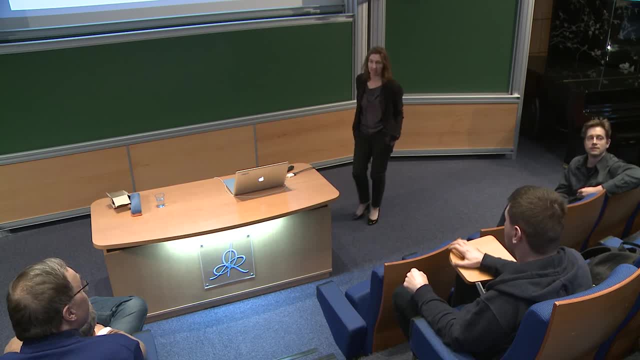 Because you satisfy the positivity constraints And so Well, it's not an interesting dynamic equation? So that Yeah, The elastic kind of thought, and go for better, Exactly, And then take away, you know, quaint. So there are. There are some really interesting questions. 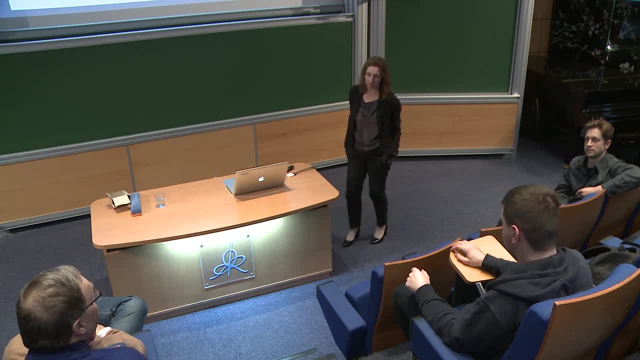 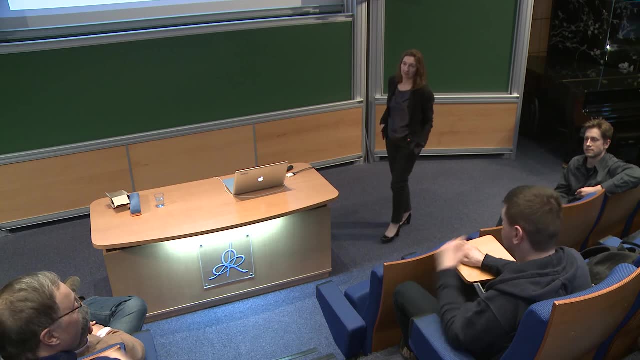 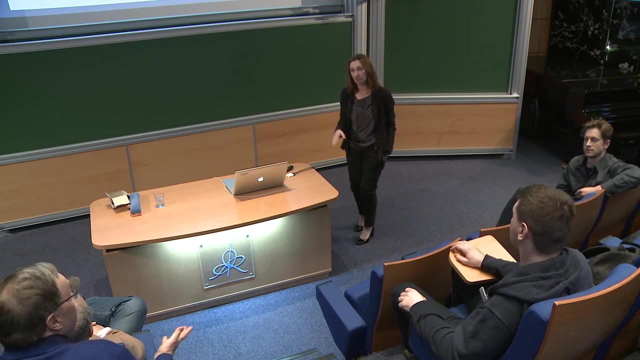 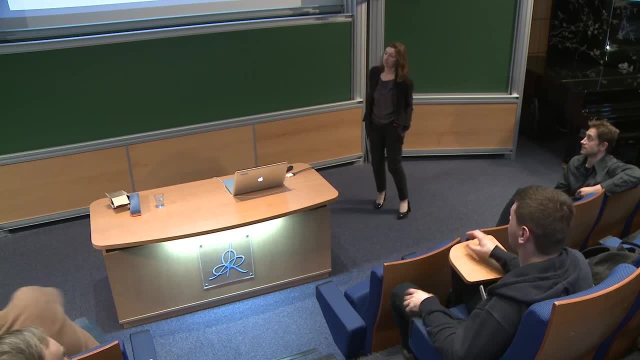 That this Euclidean formulation sort of rules out, at least at a direct way? Absolutely Yeah, Thank you, Thank you. Questions, If it makes sense to make a relation just perturbative. Yes, Yes, I didn't mention it here. 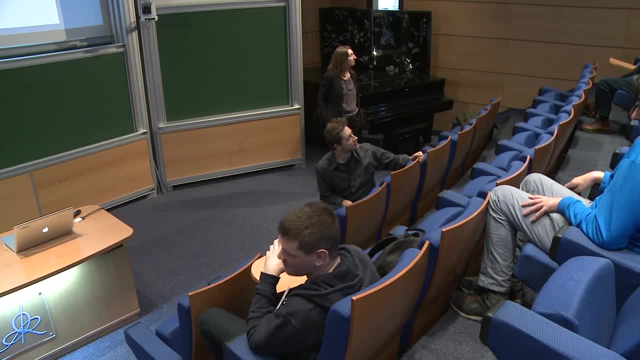 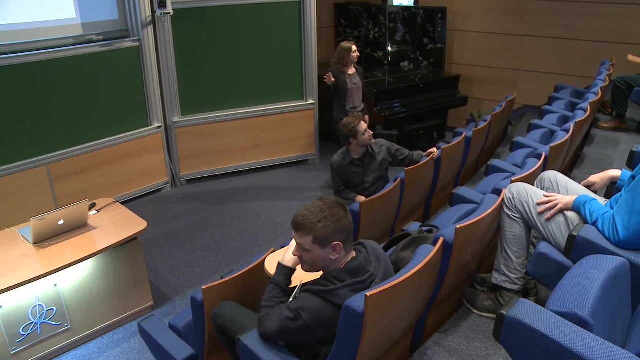 But there's, So for sure there's a, There's a Synergy between perturbative calculations- Yes, It's, I mean It's, It's, It's, Yes, Yes, It's perturbative calculations, and they're, they're used extensively in lattice. 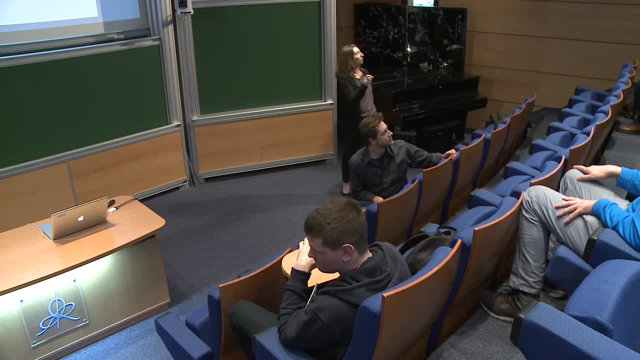 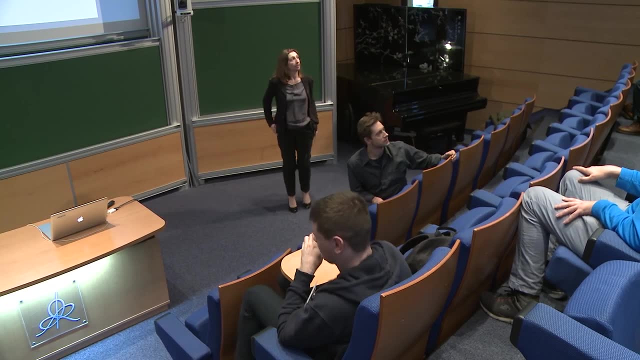 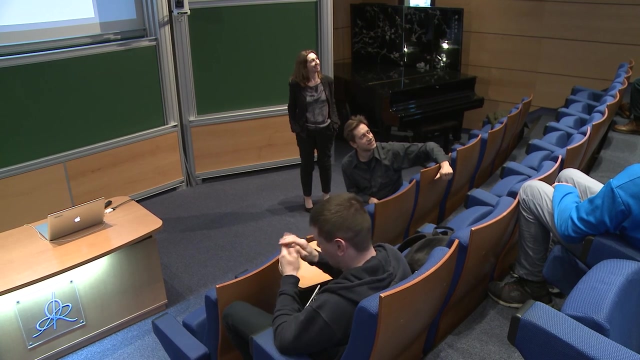 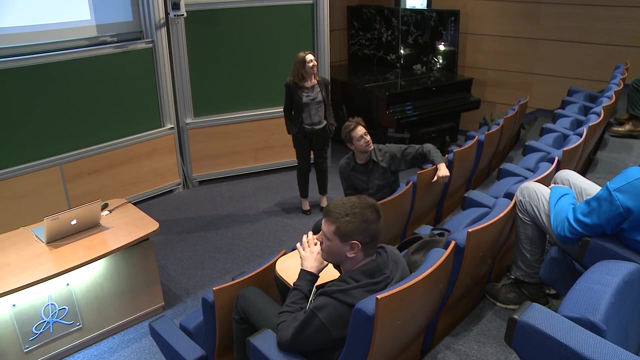 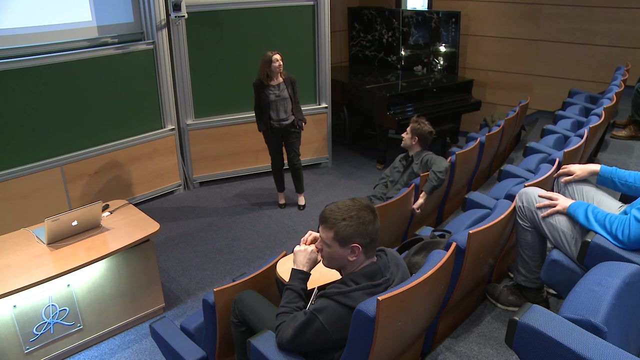 calculations as well, both as ways to calculate the coefficients of improvement terms, for example, and matrix element renormalization factors in matrix elements. so there's absolutely it's a whole question about the sociology it's so since there are no other lattice people here, I can say it's. 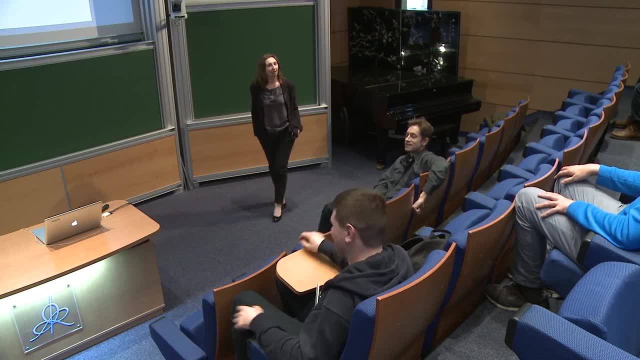 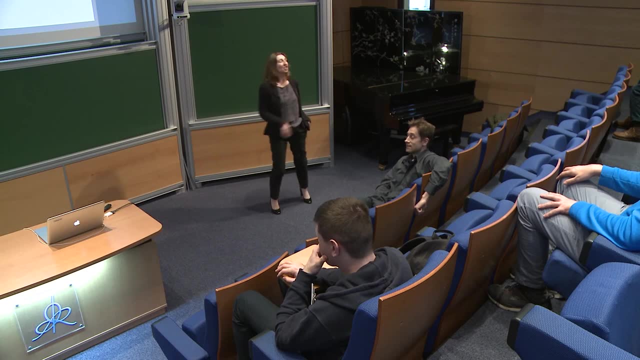 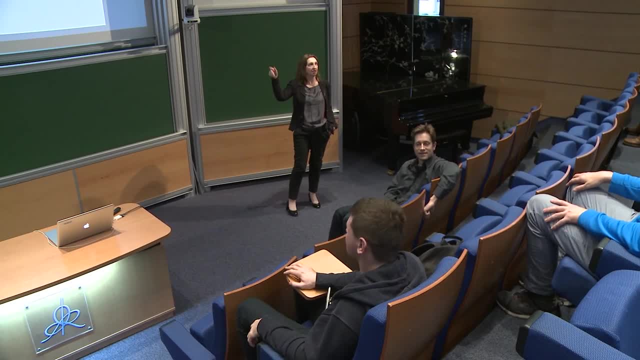 collaborations and they will work on different formulations. so in the very different formulations, so in the very different formulations. so in the very early slides I had Wilson staggered early slides. I had Wilson staggered early slides, I had Wilson staggered overlap from its, etc. so these are all. 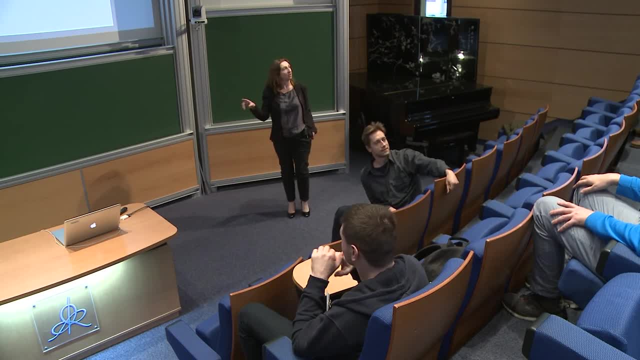 overlap from its, etc. so these are all overlap from its, etc. so these are all different groups doing different different groups doing different different groups doing different approaches to the same physics, for approaches to the same physics, for approaches to the same physics, for example. and then, of course, they check to 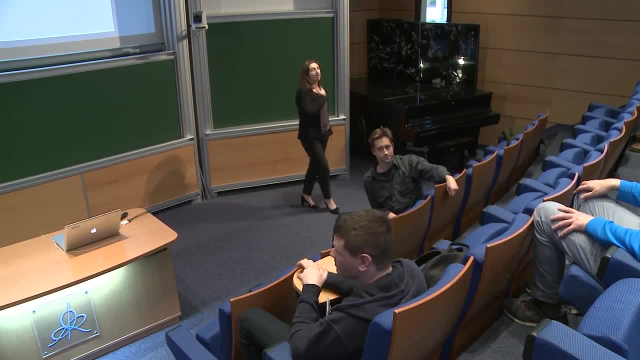 example, and then of course they check to example, and then of course they check to see whether they get the same answer. but see whether they get the same answer, but see whether they get the same answer. but also there are fundamental sort of more. also there are fundamental sort of more. 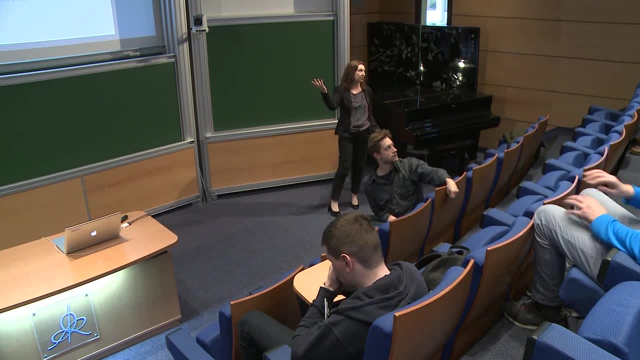 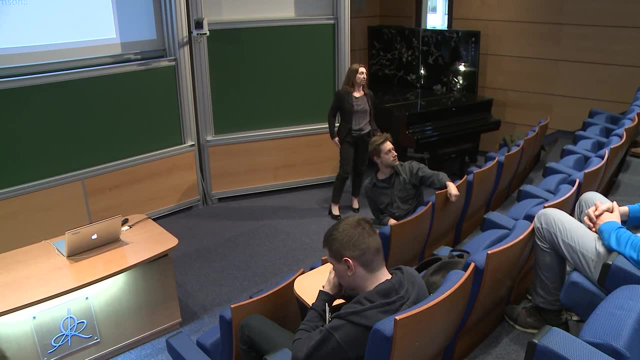 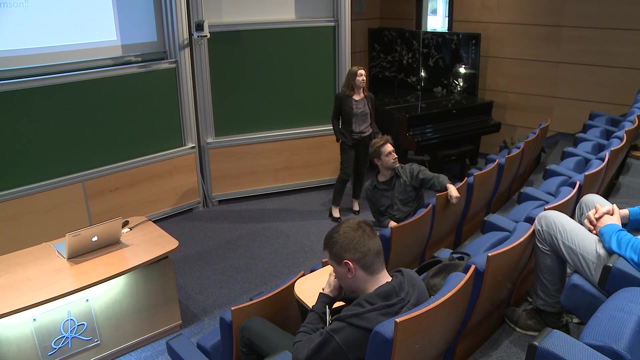 theoretical arguments about whether aspects of, for example, staggered fermion formulations are really and you can really formally show that they recover QCD in some continuum limits. so there are long-running arguments, I would say, about these sorts of implementations, including also the implementation of how you understand chiral symmetry, how you understand heavy quark physics and 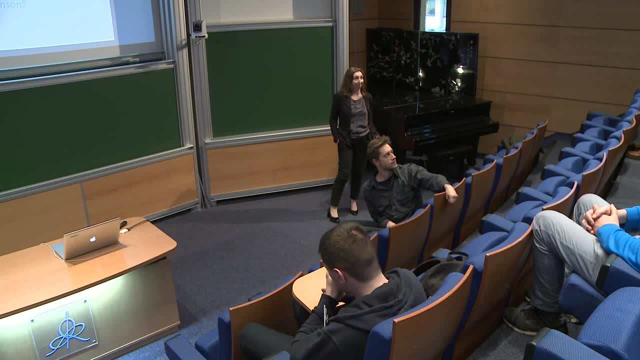 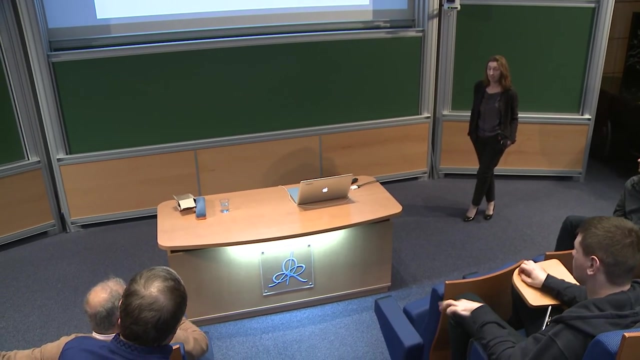 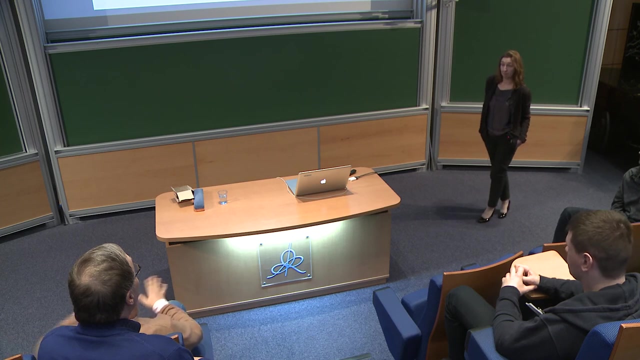 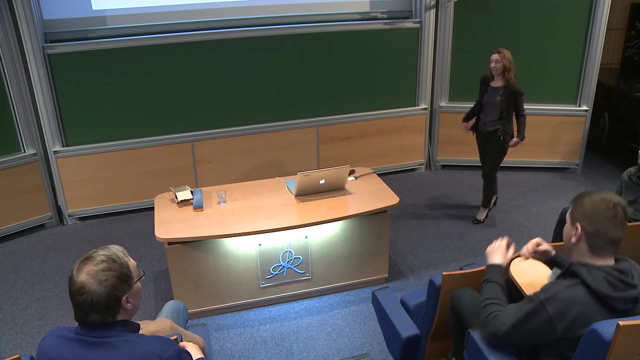 effective field theories. so the field is actively discussing amongst itself all of these issues. very self-critical, actually, I would say: well, it already does. yes, and that's already happening, Samson, so I didn't show here, but in no, no, no, I mean there's look. I mean it's very nice if you can make predictions and then